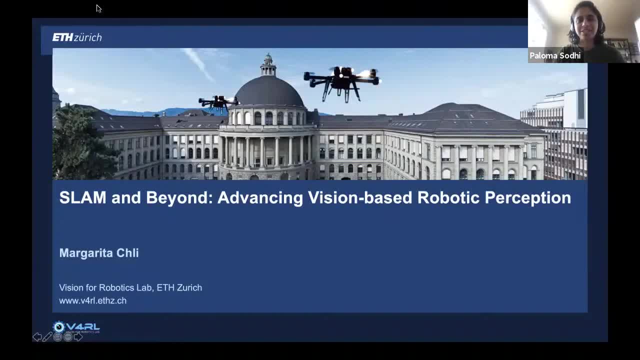 Hi everyone. So today we are delighted to have with us Professor Margarita Klee. She is an assistant professor at ETH Zurich, leading the vision for robotics lab there. She's also the vice director of the Institute of Robotics and Intelligent Systems of ETH Zurich and an honorary 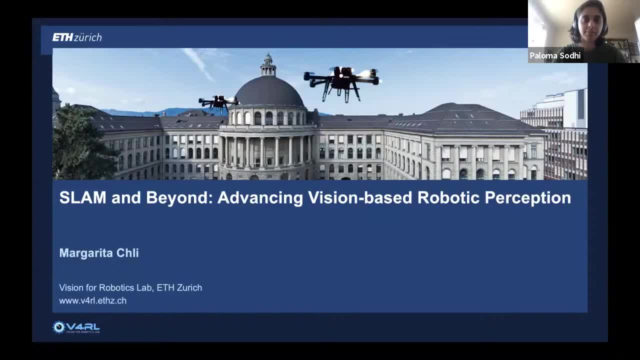 fellow at the University of Edinburgh, UK, She has held the prestigious Chancellor's Fellowship of the University of Edinburgh, as well as the highly competitive Swiss National Science Foundation professorship. Her research interest is in computer vision for robotics, with a group looking at various aspects of robotic perception, in particular focusing on real-time perception with. 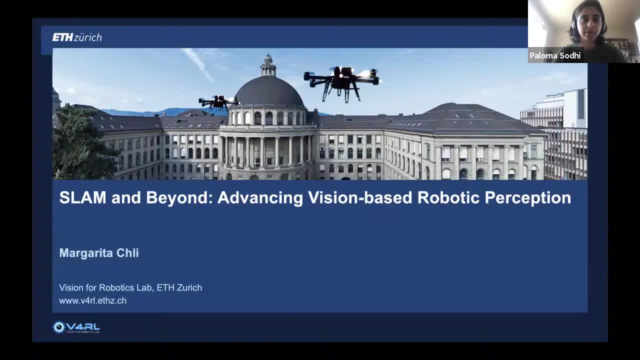 small unmanned aerial vehicles. Her contributions to the development of robotic vision have been recognized at several venues, such as the Zonderpreis Reuters World Economic Forum in Davos and Robohub's list of 25 women in robotics you need to know about Today. she will be. 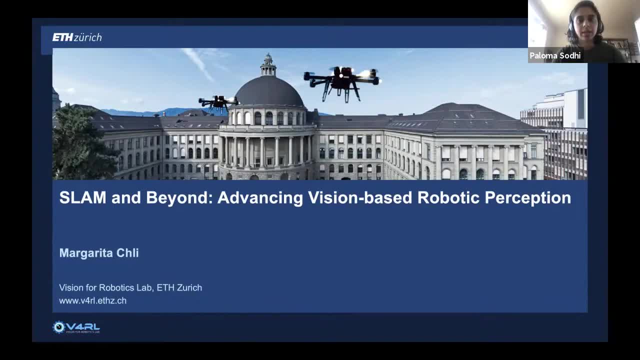 talking about the research interest in computer vision for robotics, with a group looking at various aspects of robotic vision for robotics. She will also be talking to us about her work on SLAM and Beyond, Advancing Vision-Based Robotic Perception, And with that I hand it over to you, Margarita. 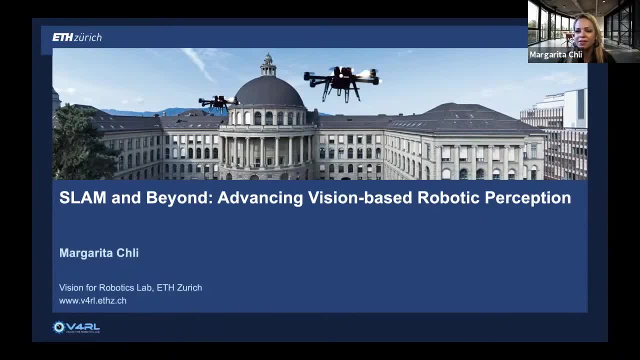 Great. Thank you very much, Paloma, Thank you very much, Nikhil and the rest of the team for the invitation. This is an amazing SLAM series for SLAM discussion and SLAM talks. So hence my title: SLAM and Beyond: Advancing Vision-Based Robotic Perception. 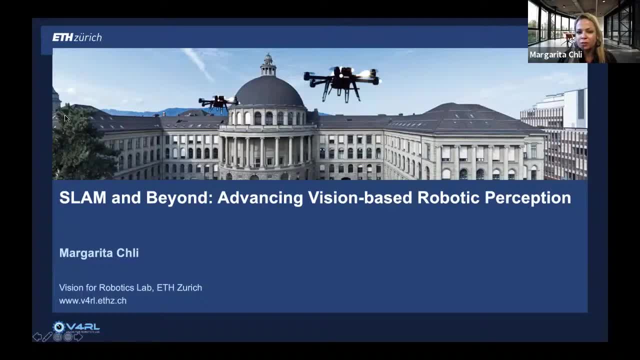 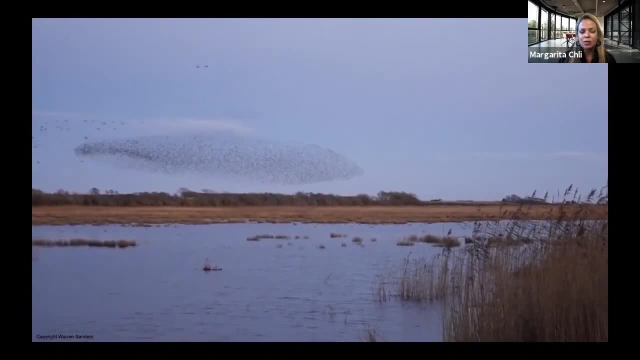 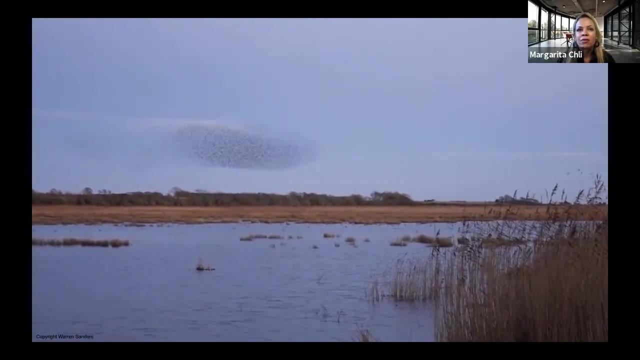 Now I wanted to show you two videos that, yeah, here we go, where you can see this flock of starlings, that they're moving in space in seemingly perfect unison without crashing into each other and creating these beautiful formations. So the question where I'm going with this is: what level? 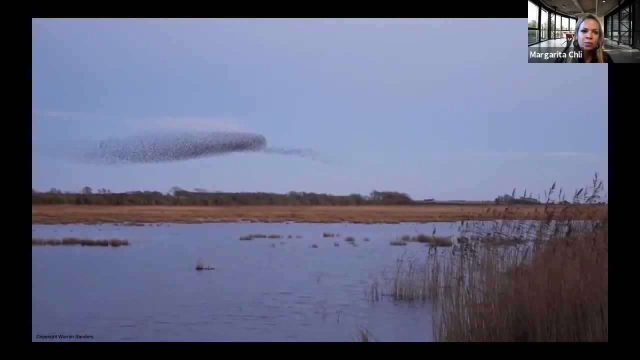 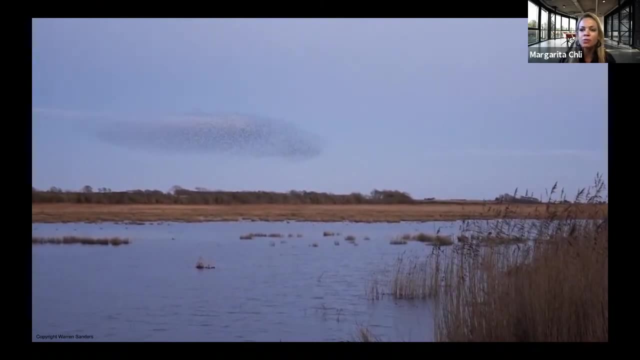 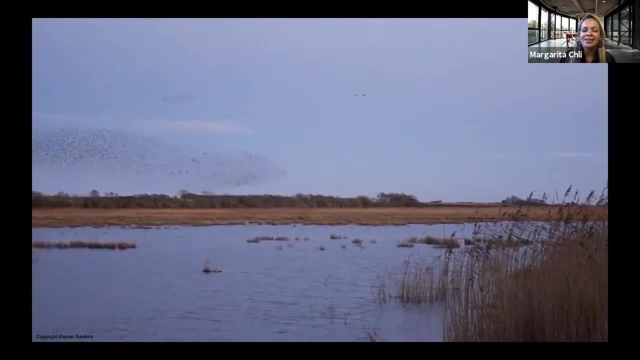 of skill and situational awareness. do we need to build into our robots in order to have the ability to navigate so seamlessly in our world around us and interact with each other, with us, with our world around us? So I've taken this huge question and I've broken it down into three 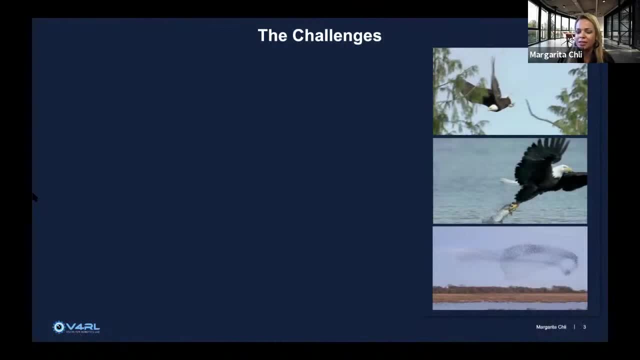 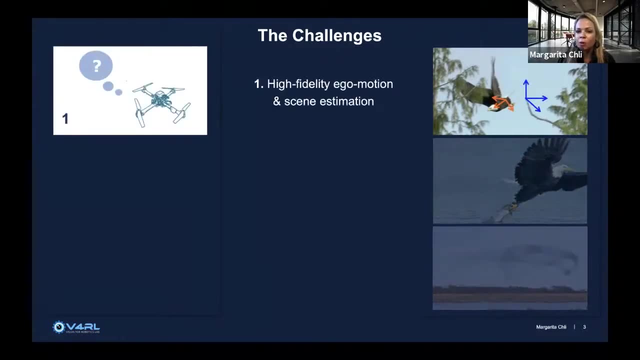 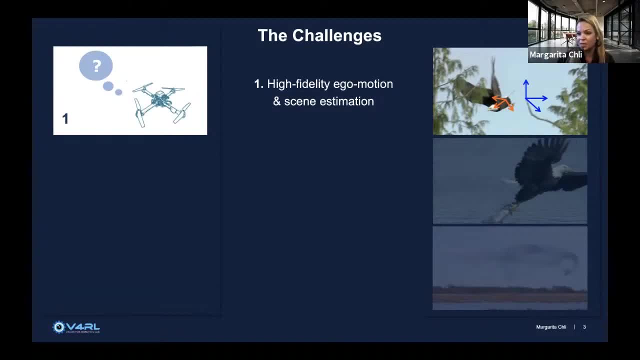 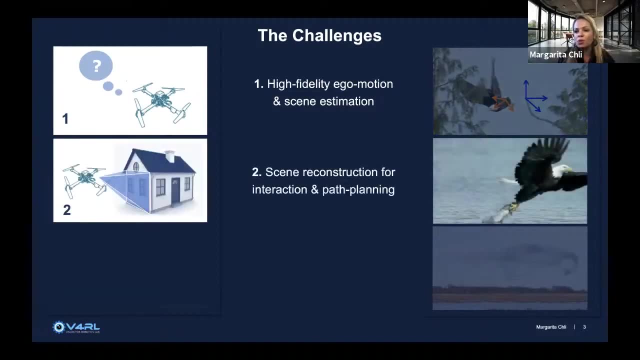 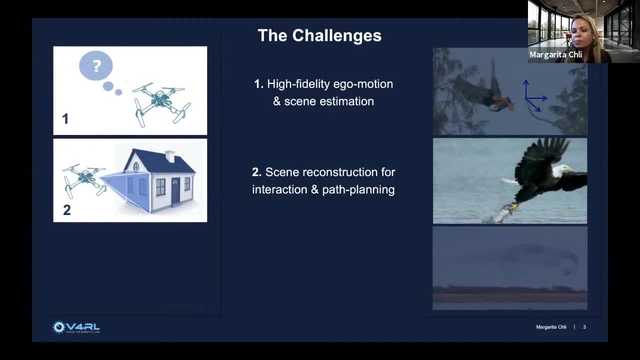 be able to interact with their scenes and actually perform some autonomous task, for example to fly from A to B or even to plan a grasping motion through space. And then, when you imagine that you have robots, that they're able to address challenges one and two, then how about? 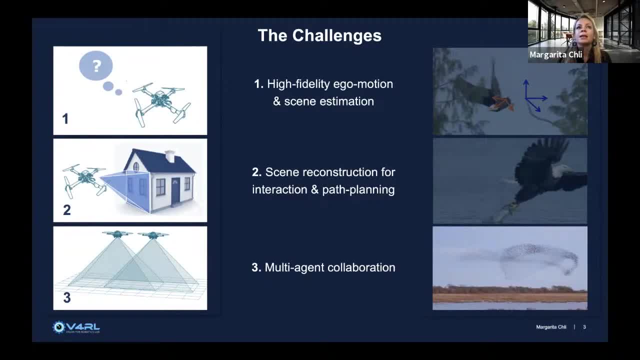 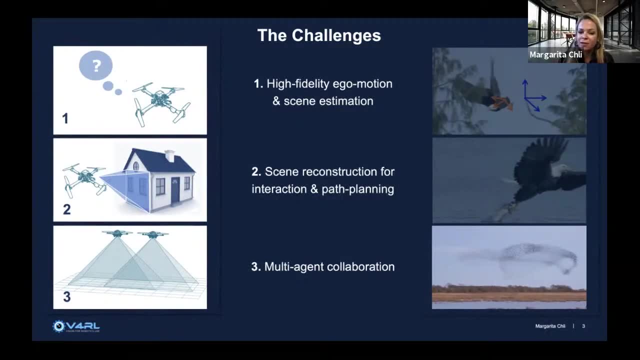 assuming that you have multiple robots in the area, that they're tasked to do the same mission, and how can we have them collaborating effectively with each other, For example, to build a common map of the scene or to transport the load of one object that one by themselves cannot transport? 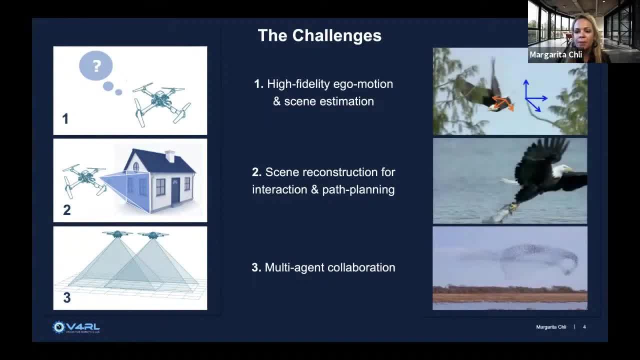 Now, these three challenges represent the three main research streams in my lab and I'm going to go through them, explain a little bit what I mean again by each of them and give you a taste of some of the works that we do to address them. 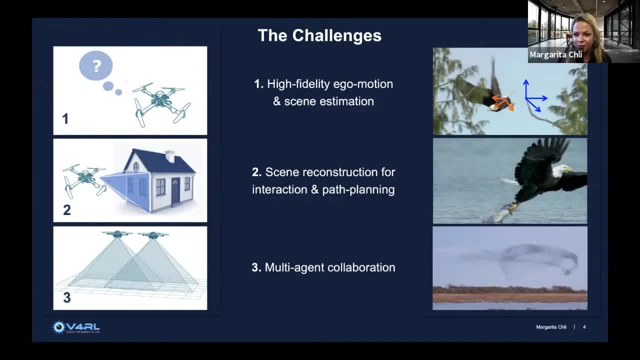 Let me clarify already that we haven't really solved any of these questions. They're very much open questions, And so what I'm going to show are approaches to addressing parts of the system, And I'm going to go through a number of these questions. So, and as you know, every 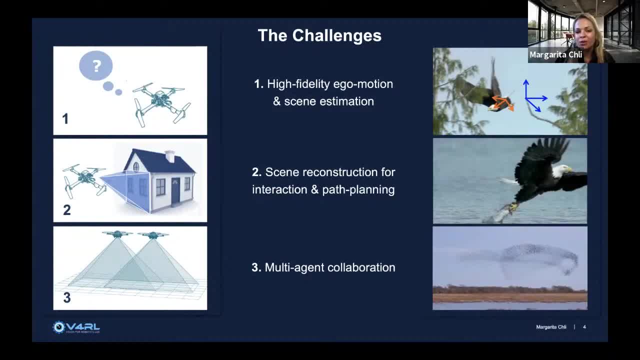 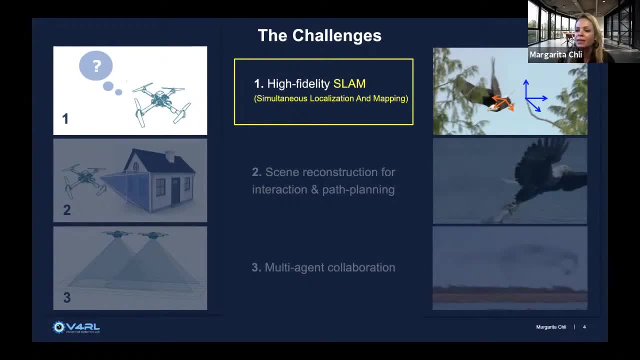 approach has strengths and weaknesses, So your task is to figure that out. No, I'm joking. So let's start with the first challenge: high fidelity ego motion and zine estimation. And, of course, what I really mean here is high fidelity SLAM. Now, in this crowd, I don't really need to give. 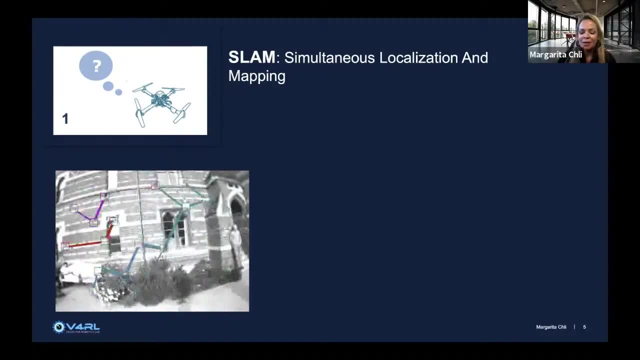 a definition of what SLAM is- the acronym simultaneous localization and mapping- But it is important to talk a little bit about the problem. So whenever I give this SLAM lecture to my students and I asked them what do they think SLAM is doing, They managed to come up with the 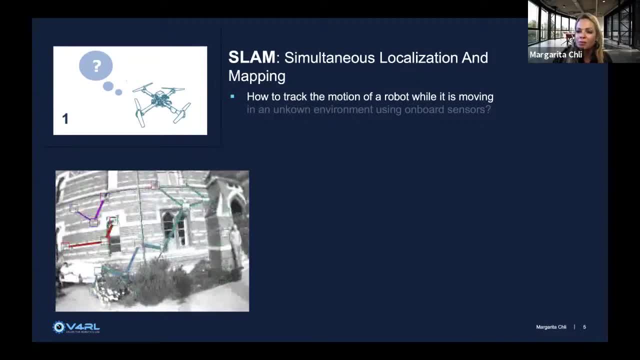 first bit of this question, So how to track the motion of the robot while it is moving. but usually they miss out the next two parts, in an unknown environment and using onboard sensors. So looking at this video here, we humans are pretty good at. 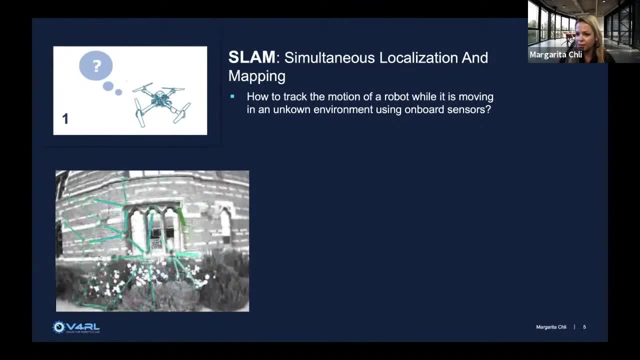 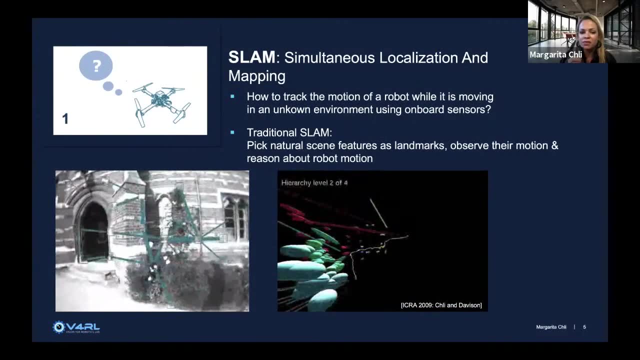 understanding how the camera has been moving in order to capture a video like this, But the way that we do this in traditional vision based SLAM, is that we're picking natural scene features- these patches that you see on the left- and we observe their motion, how they move from one. 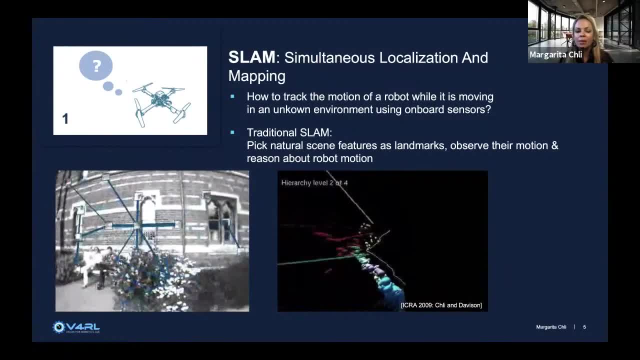 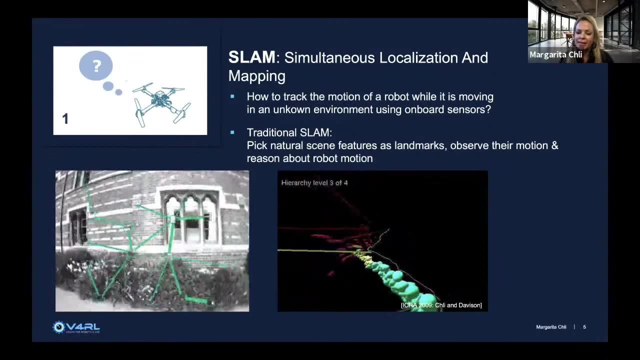 frame to the next And we start reasoning about how the camera has been moving in order to capture them. And on the right hand side, you can see an EKF map there of these features placed in relation to each other and in relation to the camera pose. 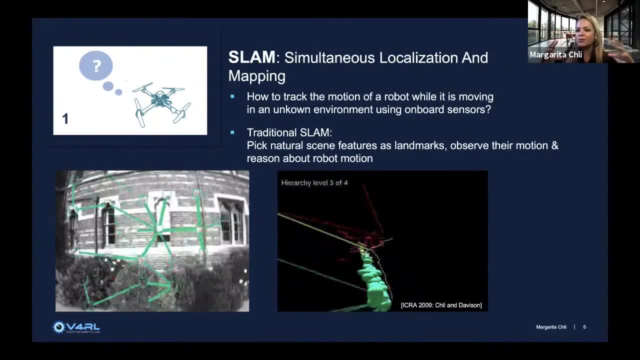 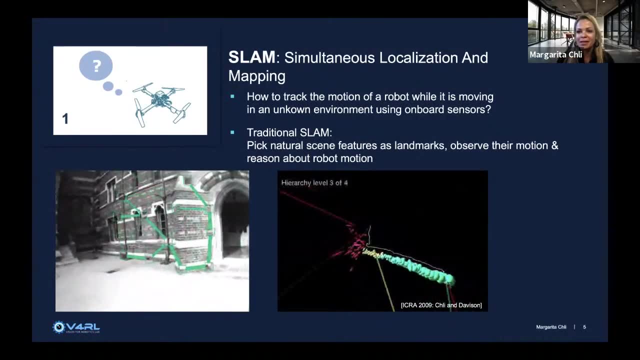 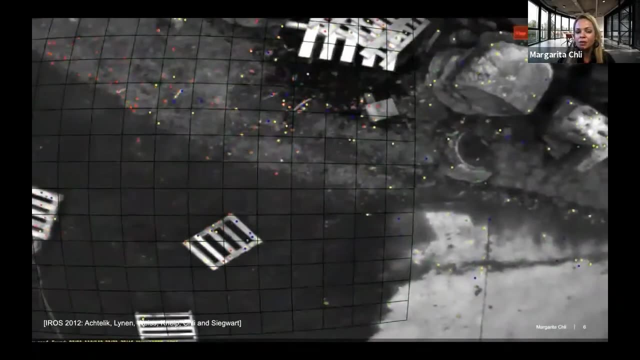 You see these blobs there that they're ever expanding. right, because we're moving away from the starting position. Now, this is an old video. it's back from my PhD. it's ancient times already, But fast forward a few years down the line. This was during my postdoc time here at ETH Zurich. 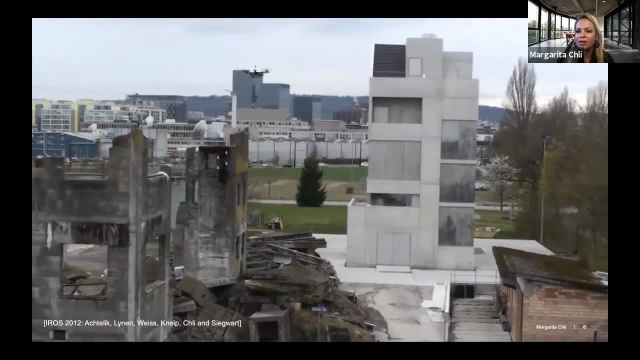 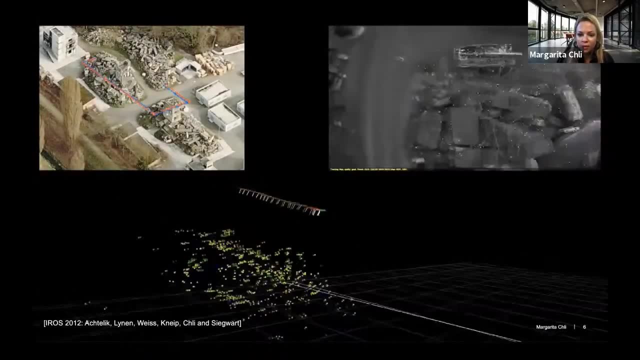 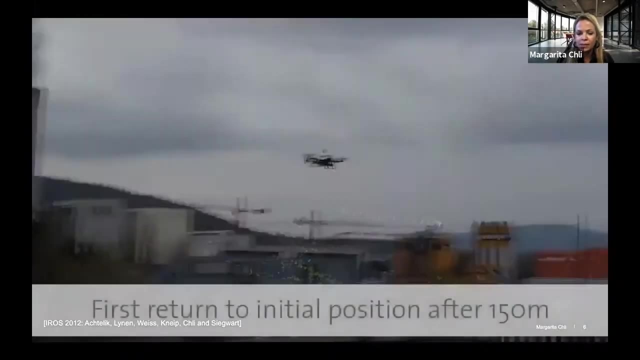 where I got to work on this project to automate the navigation of a small aircraft, And indeed what you're looking at is the result of a few years of work to make this happen. So we have a small drone that is equipped with one camera and one inertial measurement unit And we were able to show for the first. 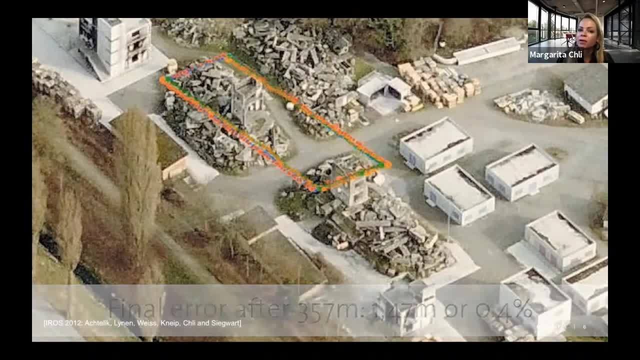 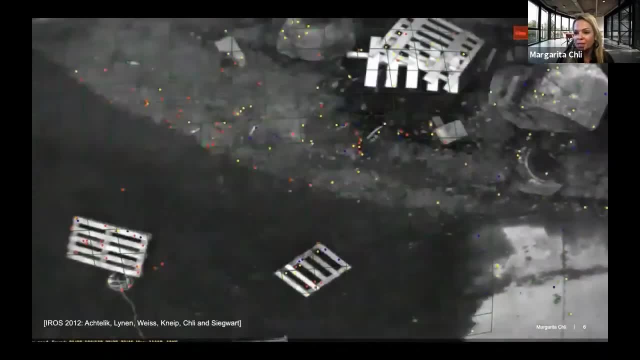 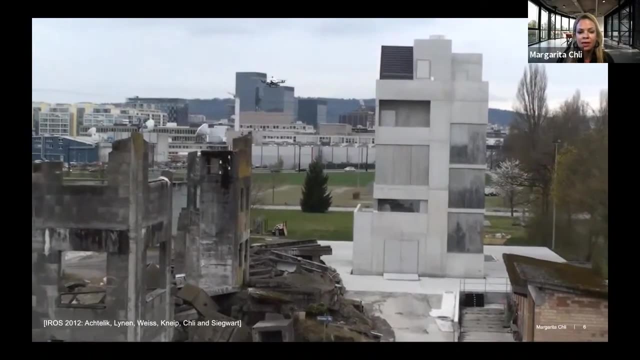 time that it is possible to automate the flight of a small aircraft like this with these sensors, right, So you can see the type of features that we're tracking. So we're using PTAM in the background, for those who know, but also using some tricks with GPS for initialization. 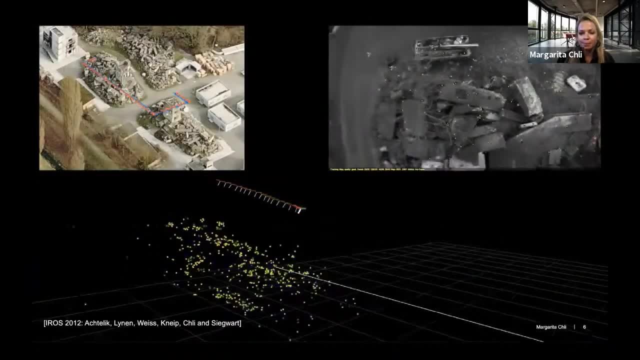 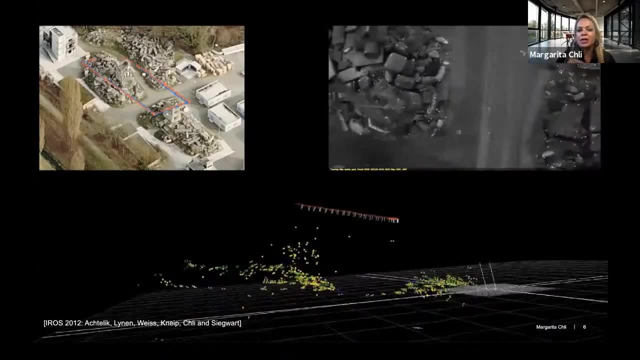 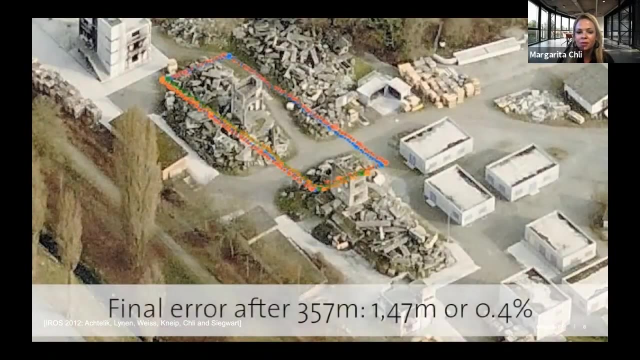 of the system And, of course, some inertial information as well. Right Now, I didn't want to talk about this, But I need to say this: that whenever you see a video like this, you need to know that there is quite a few days in advance that we needed to go. 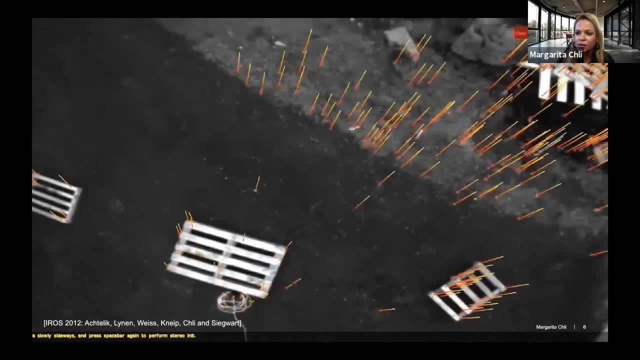 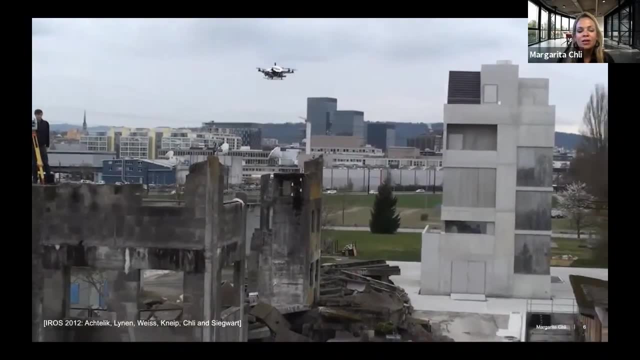 on site to calibrate our cameras, make sure that connections work well And on the day, of course, we're very dependent on how strong the sunlight is and everything. So when you're seeing one autonomous flight, of course there's a lot of manual work behind it as well. 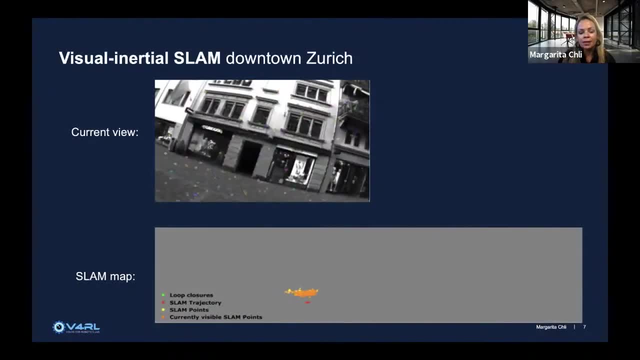 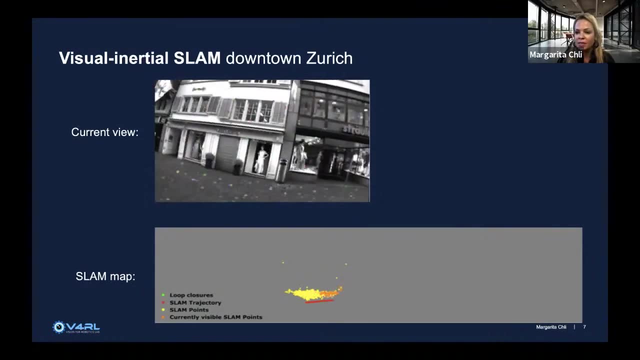 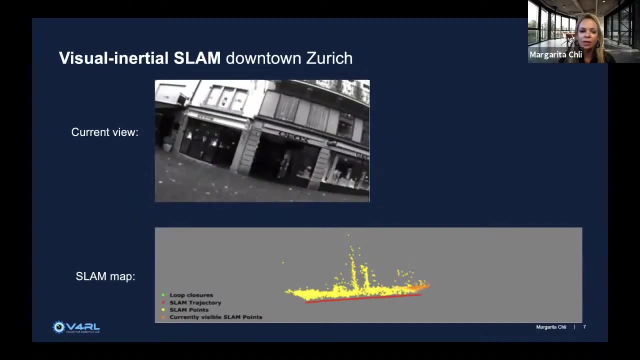 Which brings me also to my next point. when? so here you're looking at a video, a more recent one. Now, my student is walking down a pedestrian street here in Zurich. she's holding a visual inertial sensor And she's running visual inertial SLAM, actually, in this case. 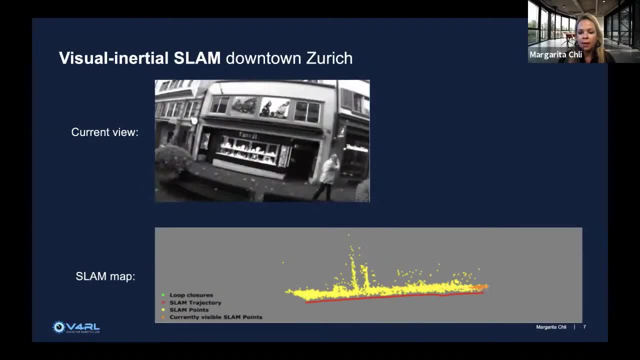 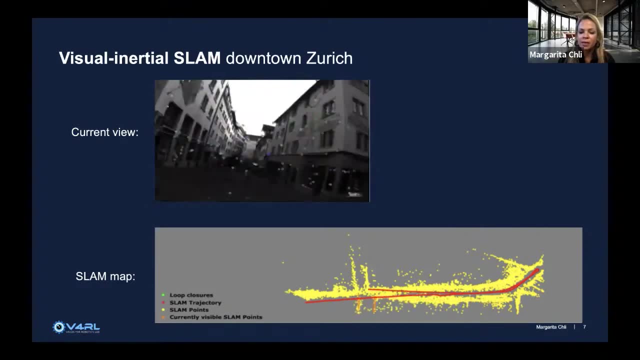 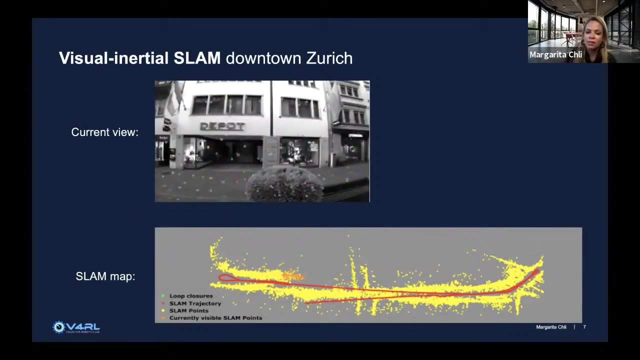 it's OQVIS using brisk features, And at the time that was the leader in the literature. So you can see the red trajectory being estimated at the yellow and orange points being estimated. So this is a straight street. she walks down one side and comes back the other side And, of course, 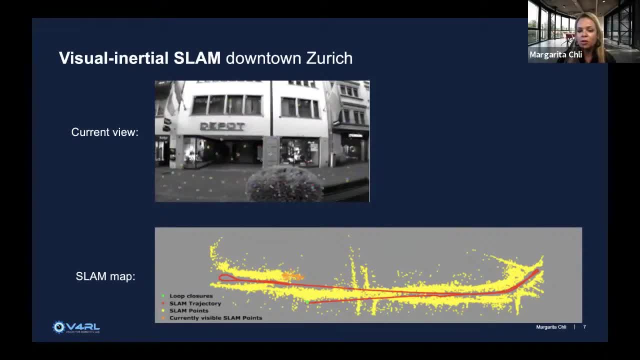 what you're observing. there is the drift, So these two locations should have corresponded to exactly the same place. So what has happened is that, during the course of time, errors have accumulated in the system which result in drift, And no matter how. 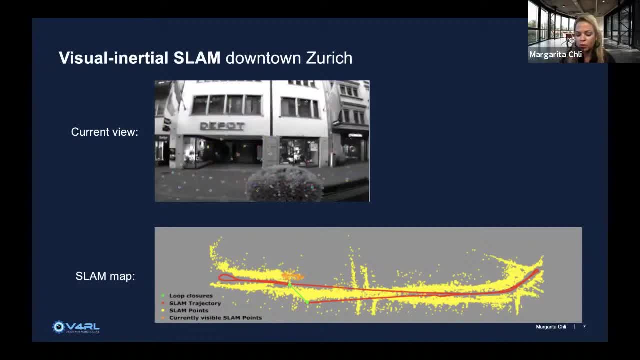 brilliant your SLAM system is. if it's not using a global positioning system or global measurements of some sort, then it's bound to drift. Good SLAM systems drift slowly, okay, but they always drift, So in cases like this, it is well. this is a well known problem in the literature. 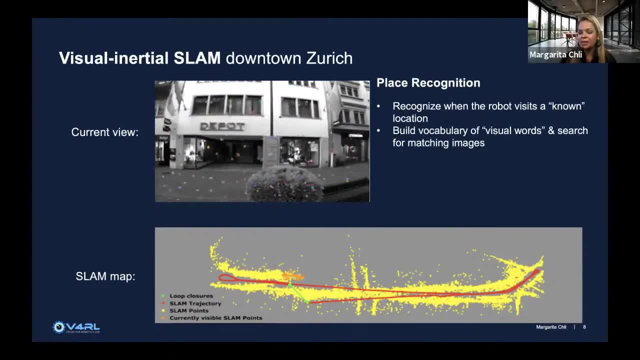 this is the place recognition problem And in cases like this, when we want to recognise when a robot is coming back to a location where it has been to before, we want to recognise that it has been to before. So we want to recognise that it has been to before. 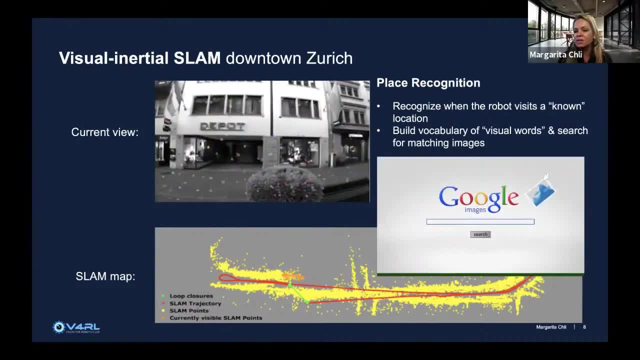 Sorry, then. we are using analogies from Google Images, basically, and Google text retrieval, to build a vocabulary of visual words and search for matching images in this database of images that the robot has captured throughout its trajectory. Right, I'm sure some of you have heard of this before. 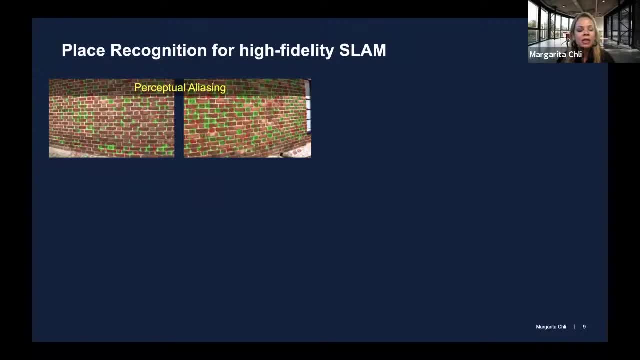 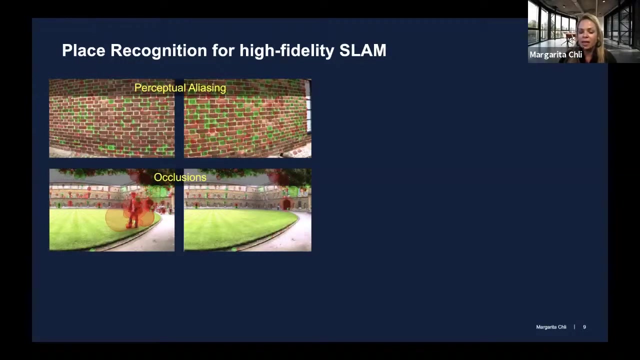 But just to show you a few of the problems that we have in place: recognition for vision based SLAM. Well, different places can appear to look the same. the same place can appear to look very different or a little different between visits and very different when you consider. 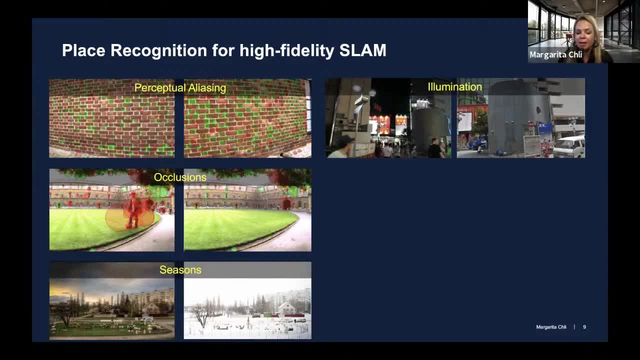 that the change in seasons and the change in illumination, so day and night changes. So you all know that these correspond to this. Well, we all know. when you look closely, you can see that these places correspond to the same location, But you can see that the visual 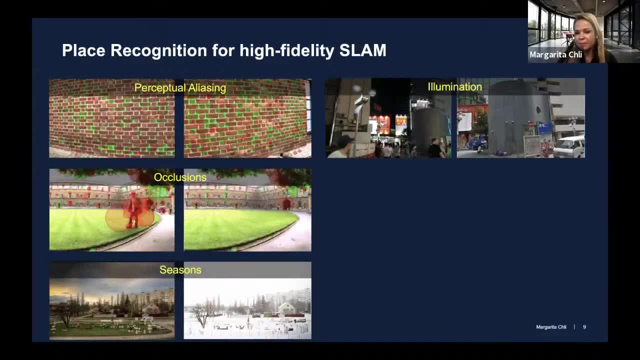 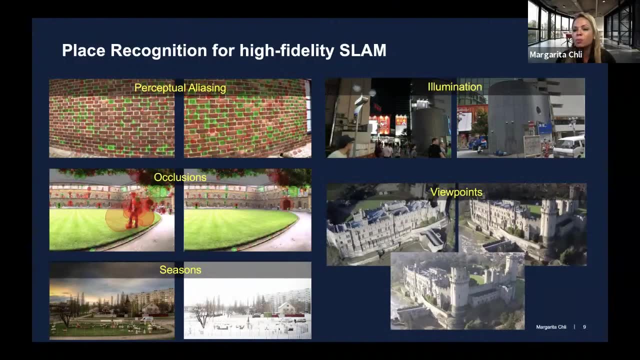 appearance has changed a lot And, as if this was not enough, when you're experiencing the scene with the drone, then you also have to take into account the problem of viewpoint changes. So this is the same place viewed from very different viewpoints. How can I make my system? 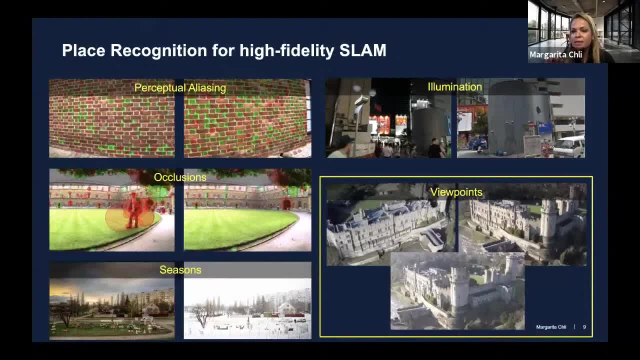 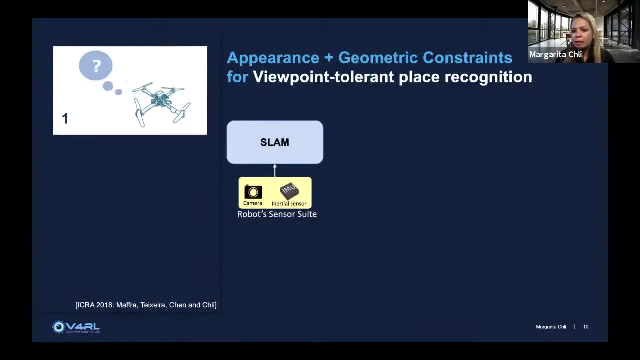 recognize that I'm coming back to the same location And let me focus a little bit on this challenge in particular. Right, so we're saying so. this is work that Fabiola and Lucas have developed in my lab, And they said we're anyway running SLAM onboard our robots. 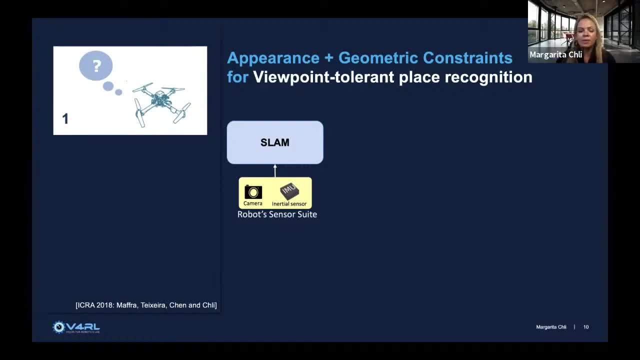 probably visual inertial SLAM- Let's assume visual inertial SLAM in this case- And we know that in traditional place recognition we are holding appearance checks, checking the current image with respect to an image database, to see whether the current image matches the visual features of. 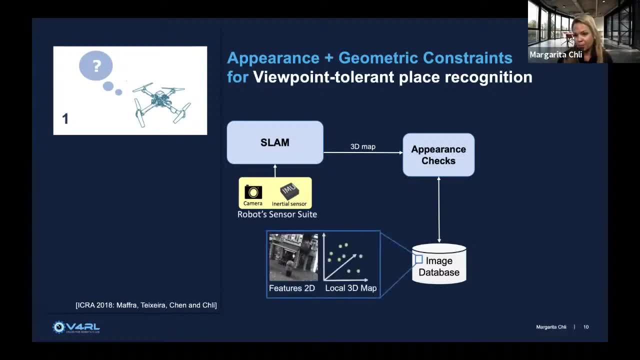 what we've experienced in the past. But since we are running SLAM anyway, why not also store a local 3D map of that location as a geometric signature of what that location looks like And what does that mean? That means once you run your appearance checks. 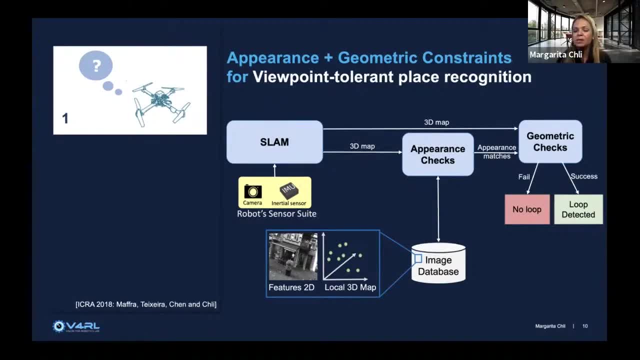 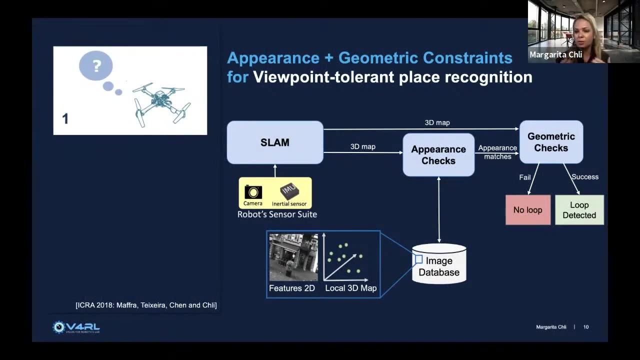 then you can run also geometric checks to filter out any false positives that you get out of the appearance match. So here we are running three-dimensional and two-dimensional appearance checks from 3D to 2D and from 3D to 3D, basically. 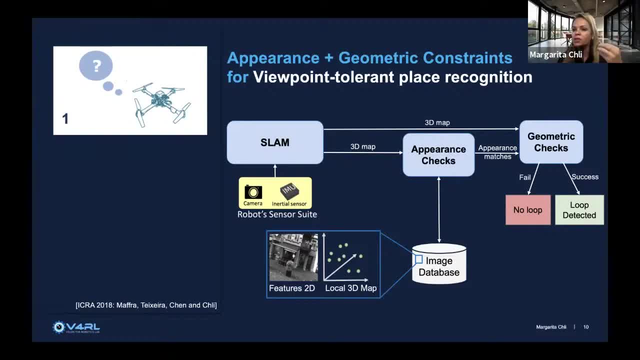 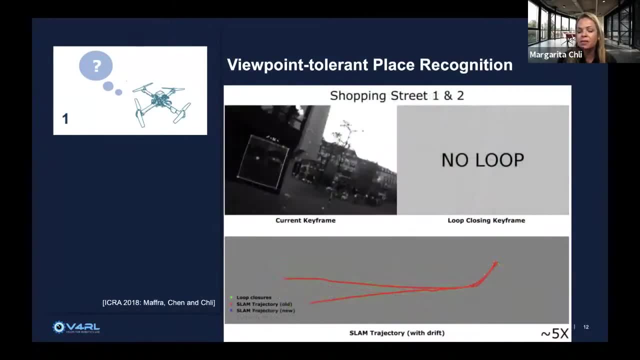 to match the current view with respect to potential matches from the database, And here you can see the system in action. We're going back to the same place a few months later, actually, And you can see the trajectory here in blue- And we are able to recover a lot of loops. 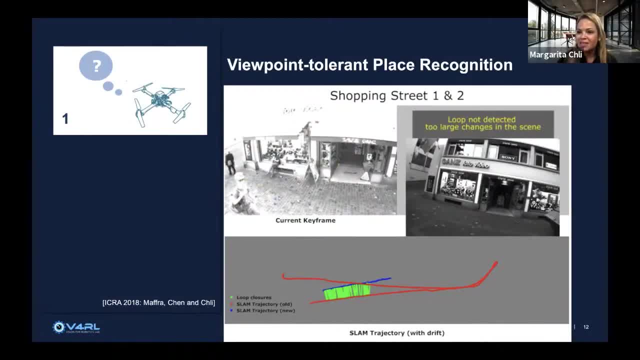 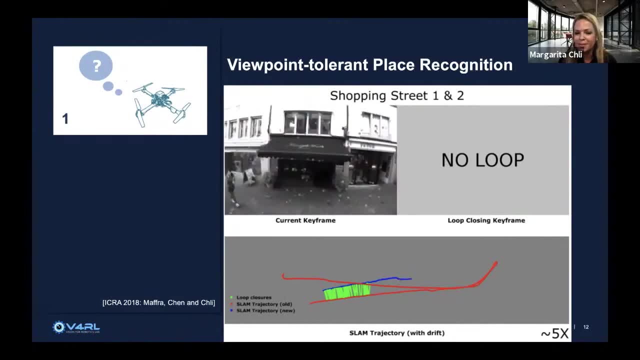 Here. you can visualize them in green, But you can see that some of them, some of the loops, we were not able to recognize. Why? Because when Fabiola was labeling this, the data set, she was telling me it's actually so hard for the system to recognize this because the stores have changed. 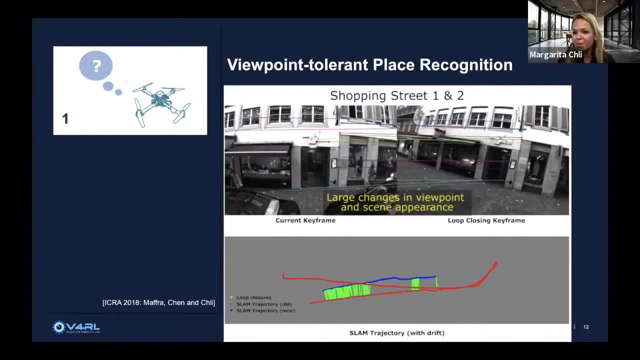 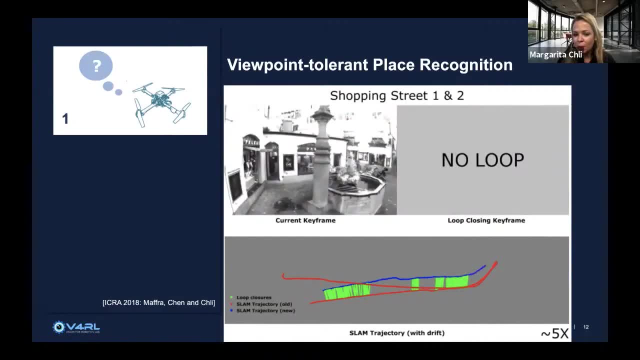 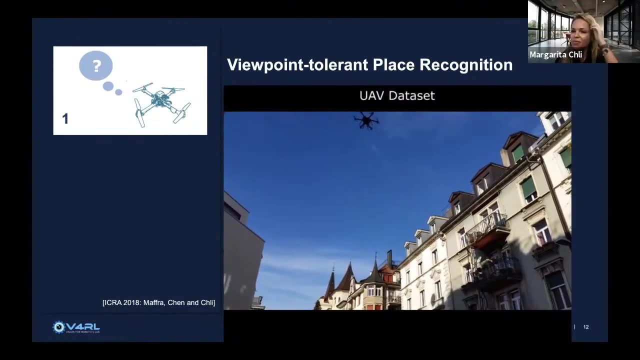 their displays right. We've gone from- I don't know- the summer collection to the winter collection, and some stores have even changed their logos. So these are. it comes to show you the whole pipeline of suppression of information that we do as humans, when we are recognizing whether we are 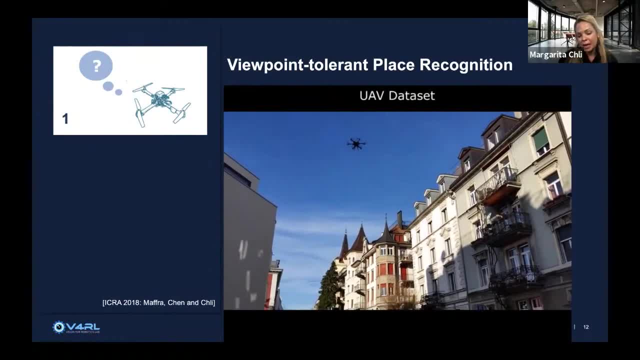 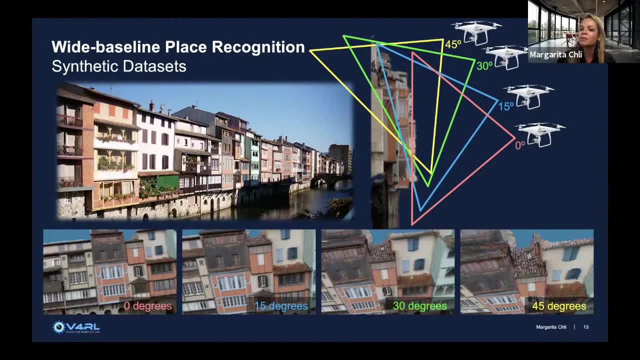 in the same place or not, right Right, But nevertheless we had some good results in viewpoint tolerance. but we wanted to push this a little bit further for wide baseline place recognition. So we actually thought, you know, we want to have 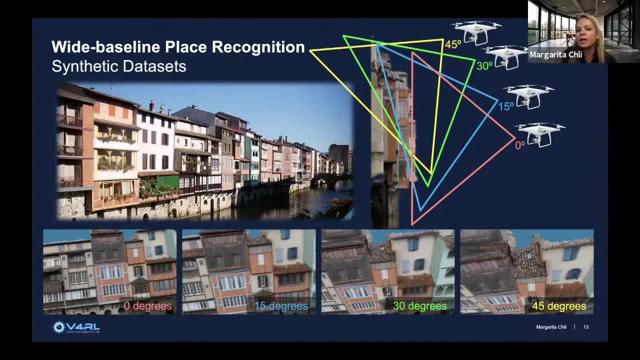 up to from zero to all the way up to 45 degrees, as you see here, as I define 45 degrees here from the horizon right. So we know that current systems were not able to perform at this level of baseline changes And the way to test this would only be a simulation. 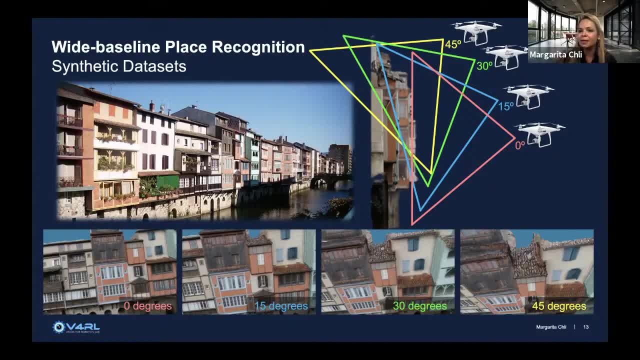 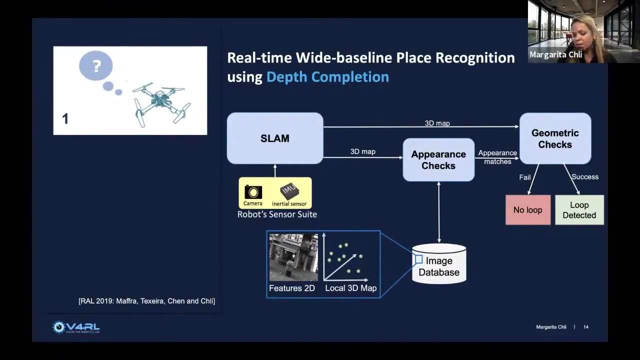 because then we would have the ground truth on what really is the correct viewpoint change and the overlap of the scene from scene zero to scene 45 degrees. So how we did that? we've taken the system that we had before, but in order to augment the tolerance. 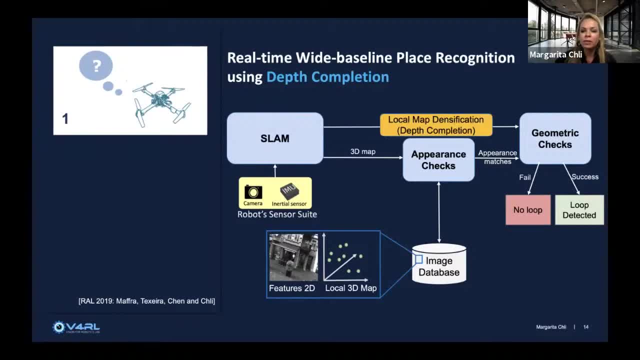 for viewpoints. then Fabiola and Lucas came up with this idea of doing local map densification to come up with a local mesh, three-dimensional mesh of the structure that we are interested in, in order to enhance the geometric checks that we're doing, because that's exactly what is. 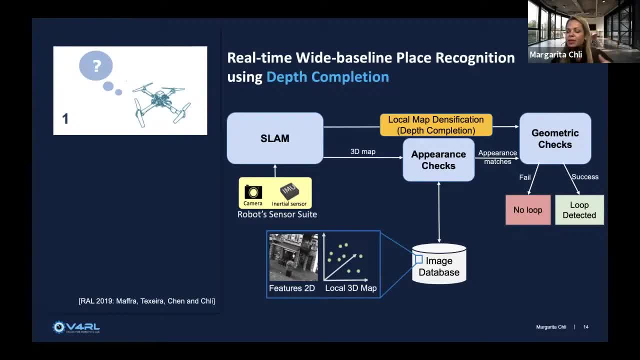 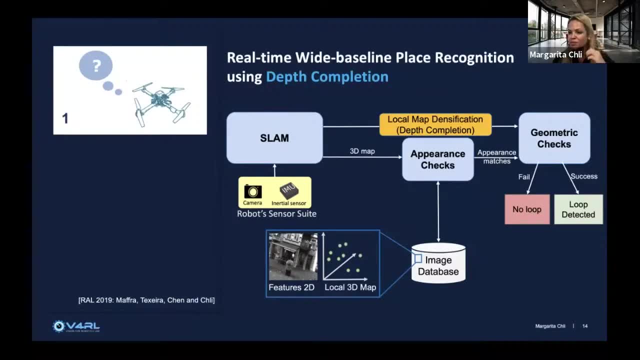 breaking right. So the planarity assumption that we usually make by looking at the geometry, you're looking at 2D features, right? Yes, it's a little bit changed when you're looking at the 3D structure of your sparse features, but they're still sparse. So some local map densification has proven to be. 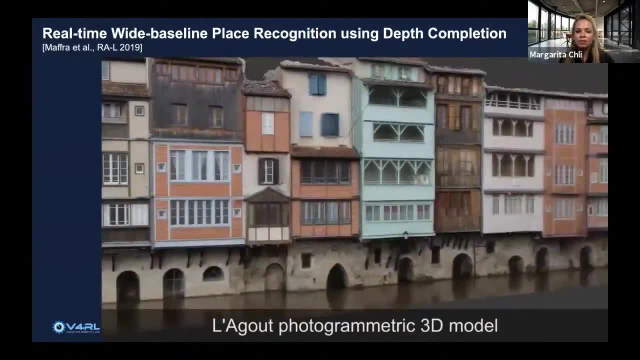 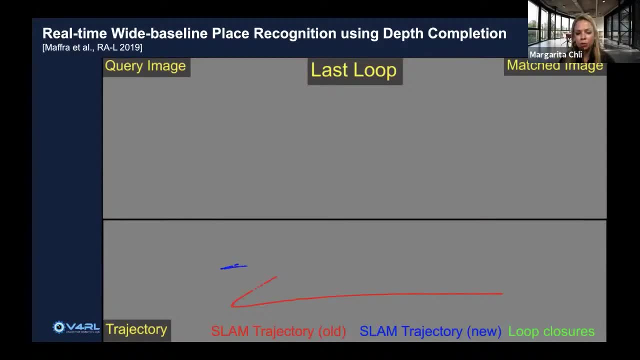 very, very helpful. And here you are looking at some examples. First of all, at this planar scene- the lagoon photogrammetric dataset, we are matching the new blue trajectory against the reference red trajectory. You can see that the blue trajectory is the reference red trajectory. 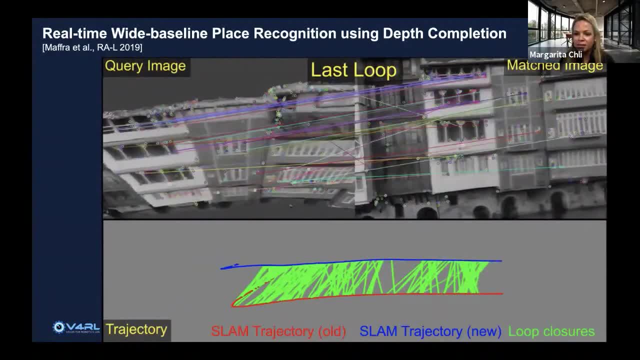 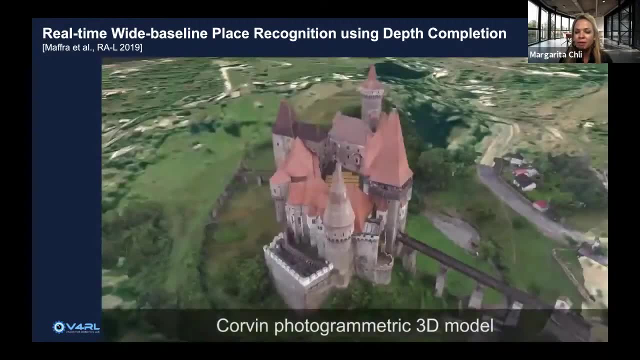 You can see on the top the two images from zero to 45 degrees and have a look at how different they actually look. And it's on purpose that they're in black and white and a little bit degraded because we want to simulate the kind of images that we get from our sensor onboard. Here you're looking at a 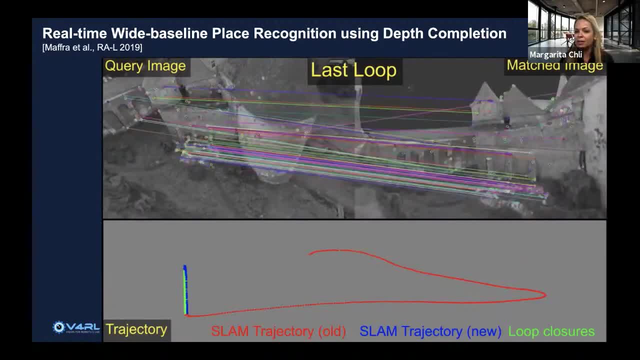 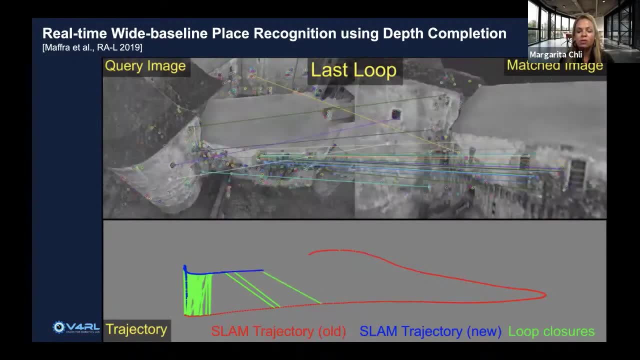 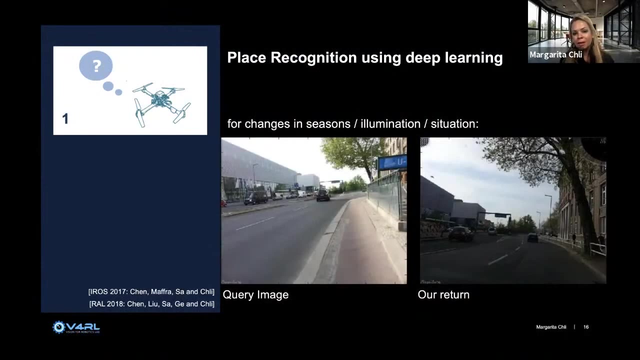 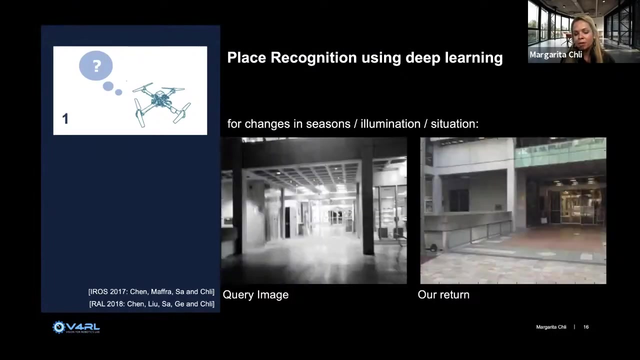 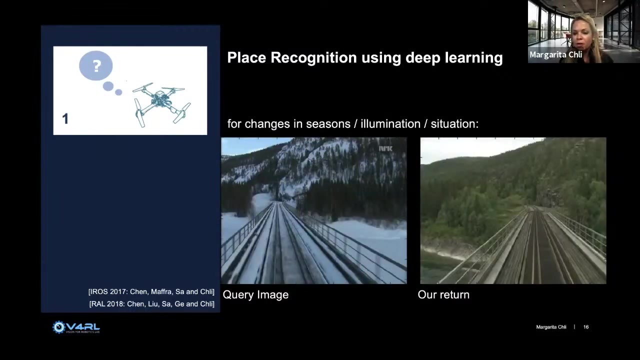 more three-dimensional scene where viewpoint tolerance can actually is really challenged, but we have shown that we achieve better recall for perfect precision with respect to the state of the art. Right Now, when we are talking about seasonal illumination and situation changes, then not only in my lab, but also in general in the literature, I think it's fair to say that we resort to deep learning right, And here you're looking at a system that has been trained. 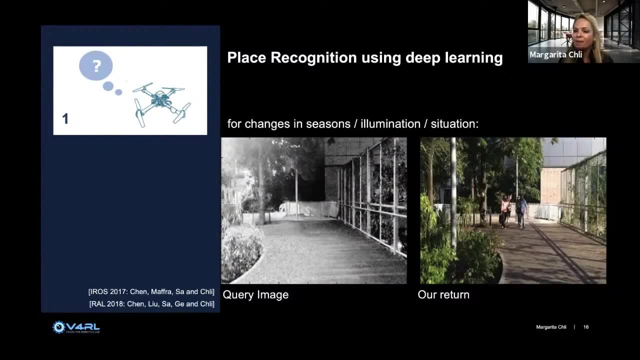 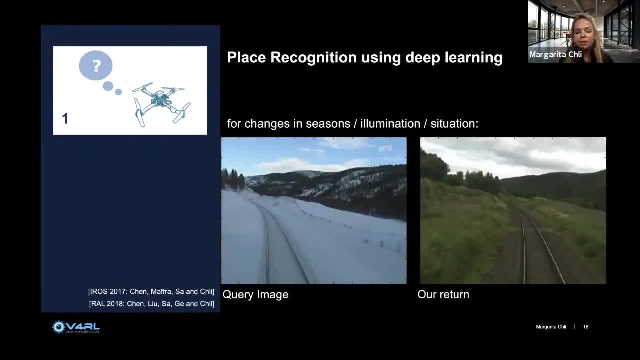 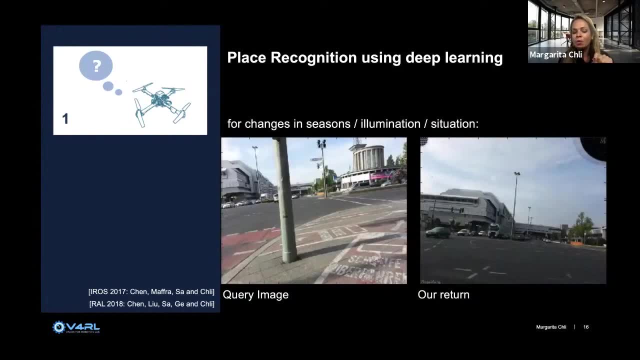 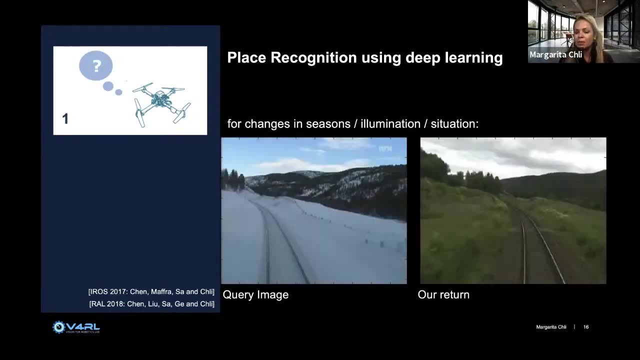 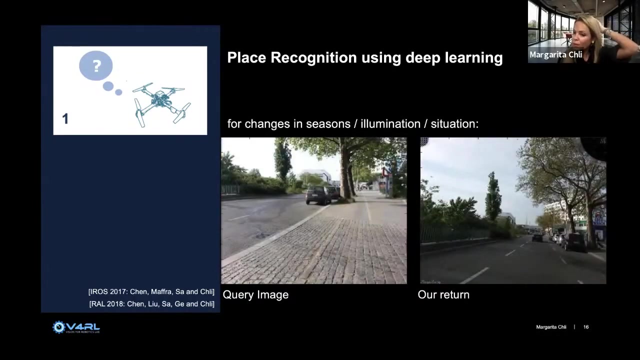 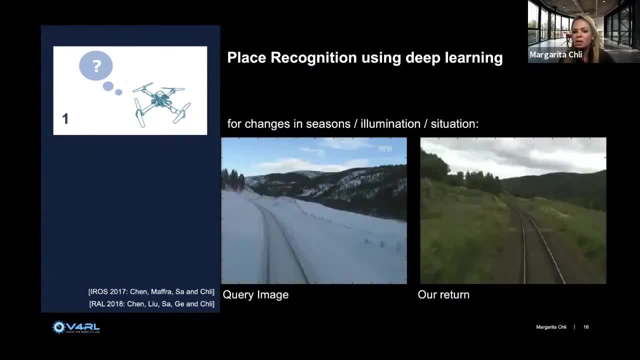 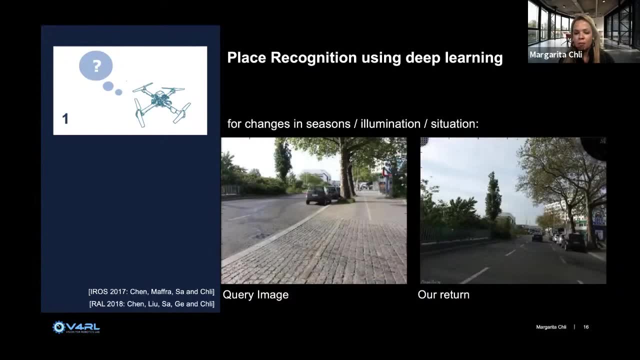 We have on one side the snow here and on the other side the grass, and you can see that the system is able to recover the correct return for that query, which is a little bit of a magic, but I have to say it doesn't work always. Of course it has its limitations and we can talk about them. 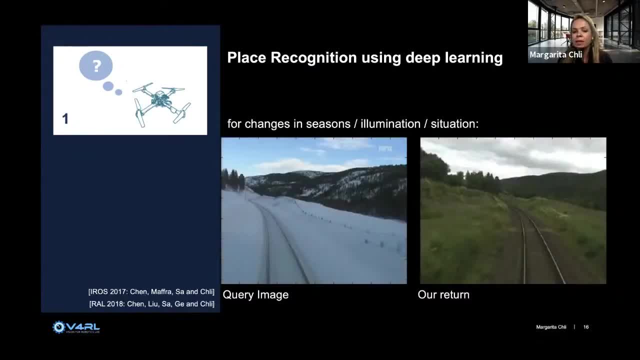 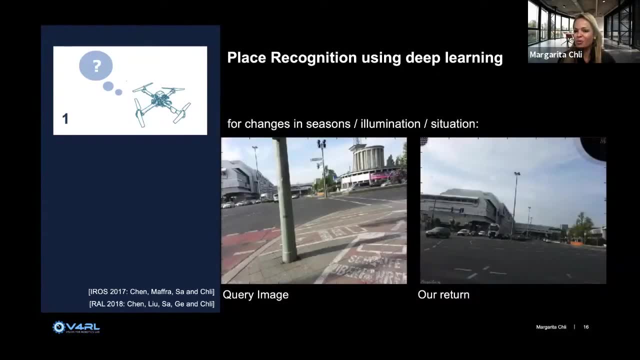 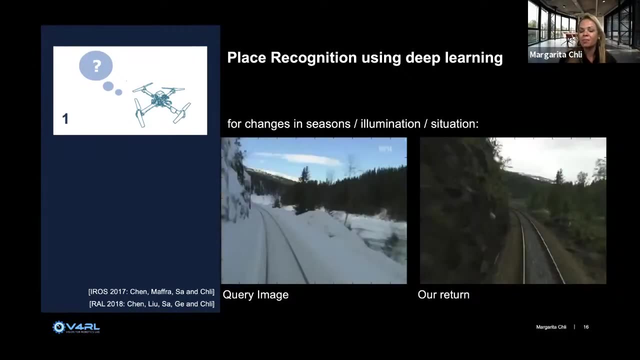 later if you'd like. but just to hint a little bit, it has to do with, of course, the viewpoint here. All the viewpoint is really looking upright right. No viewpoint changes here. The sky is always on the top and of course it really depends on what kind of data you're training your framework with. 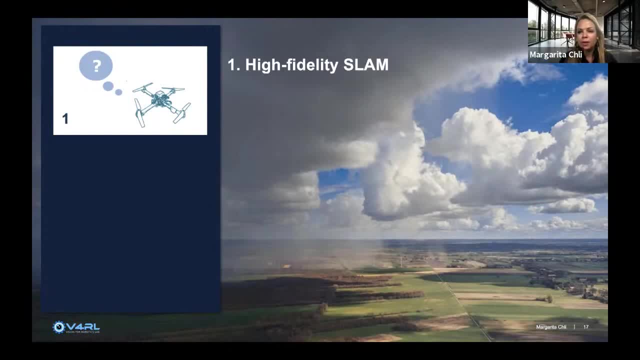 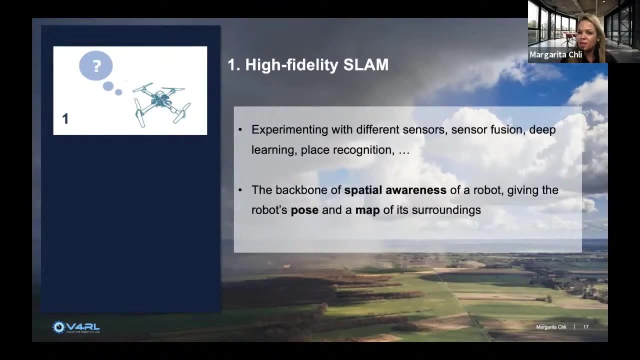 Right. so for high-fidelity SLAM, I've shown you quite a few works. So we've been experimenting with different sensors. I didn't really talk about this, but we do work with different sensors. When I say vision, we mean it in a very loose term. so we work with event-based cameras with depth. 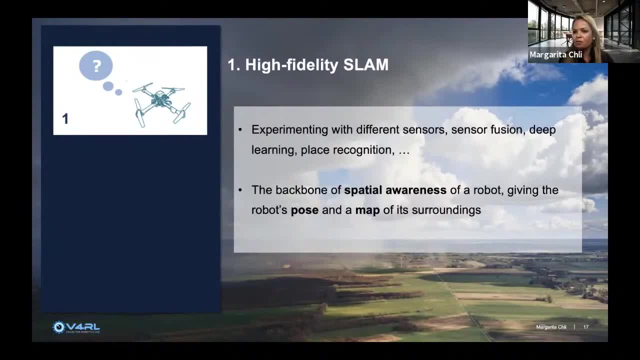 cameras with LiDAR, but, yes, of course, primarily with traditional visible light sensing and then, of course, with sensor fusion, with deep learning, with place recognition. Why? Because we want to form this backbone of the awareness of space. 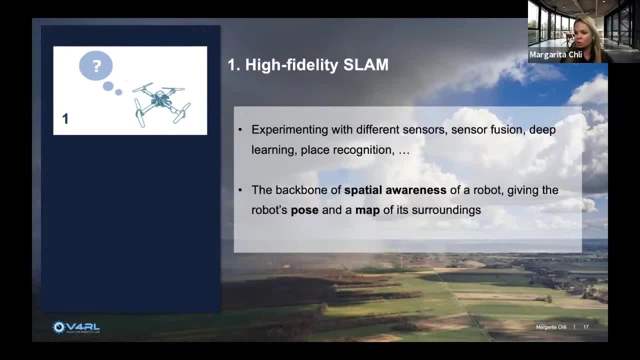 for a robot right to give it a sense of its pose and a sense of the map of these surroundings, and the key word here is that this map so far has been largely sparse right, which brings me to the second challenge. So we would like now to 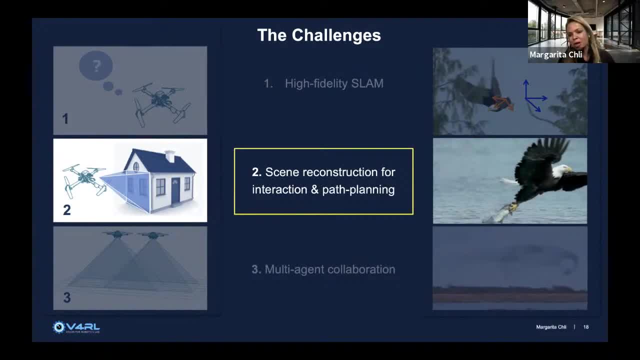 build in some more intelligence in our robots to come with richer scene representations. Why? Because when you have a point cloud as your scene representation, if you reach out to grasp an object and in between your points there's nothing in your point cloud, you don't know if it's free space. 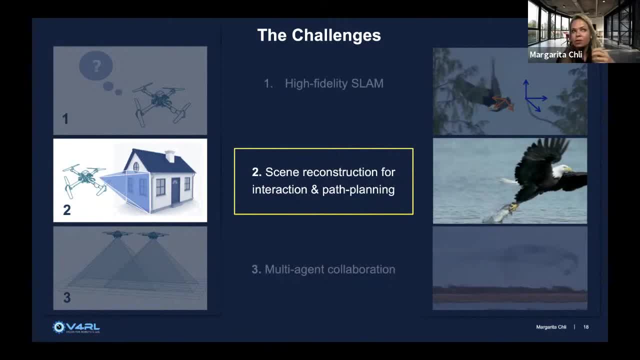 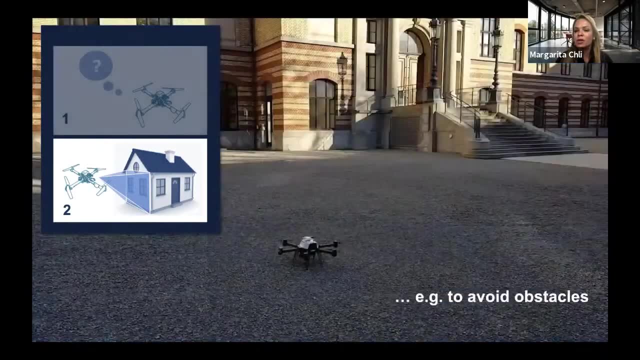 and you're not going to crash into it. and you don't know- sorry, you don't know if there is a wall and you're going to crash into it, or you don't know if it's free space and you can actually navigate through. So that's why we want scene reconstruction. 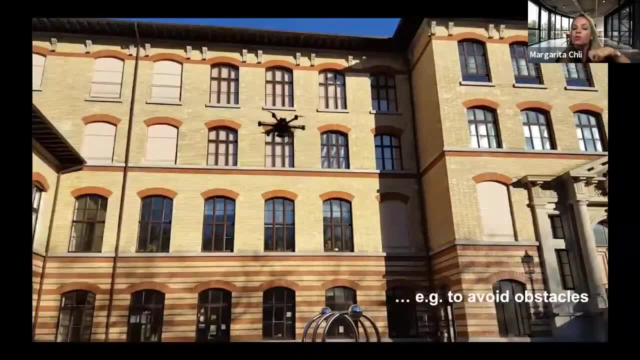 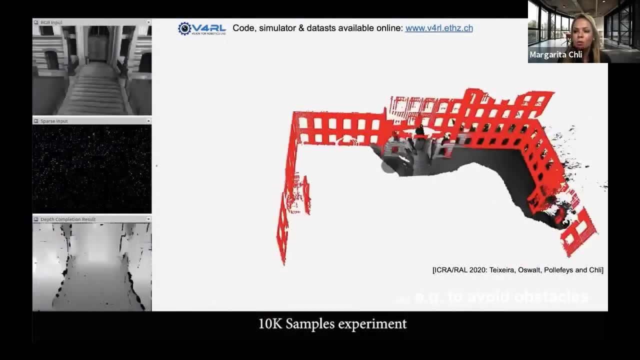 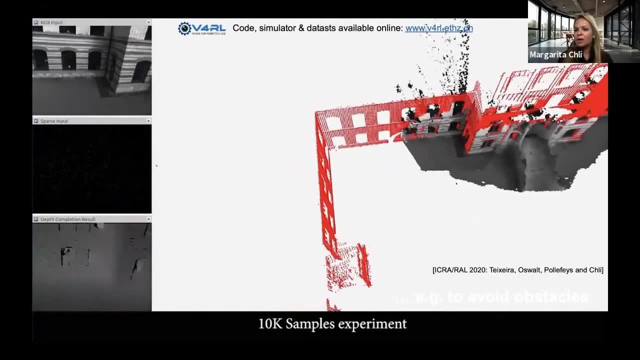 for interaction and path planning, to reach out and grasp objects or to avoid obstacles while flying. And now you're looking at an example. we have a drone that is using one camera on board, and we have gone to this area before with a tripod and captured a laser scan of the scene. Here you're. 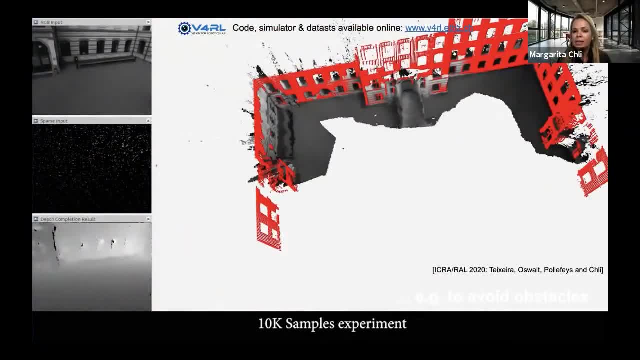 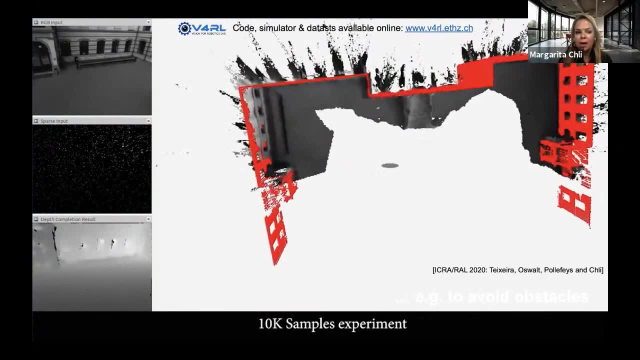 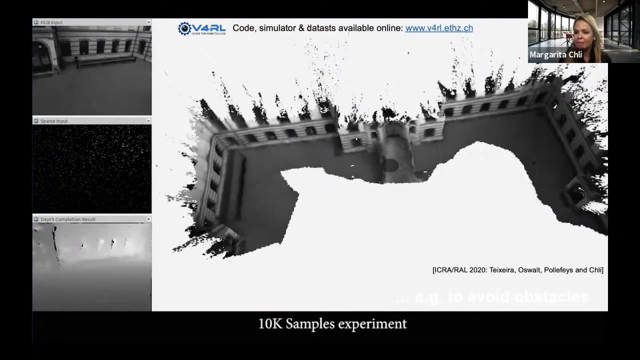 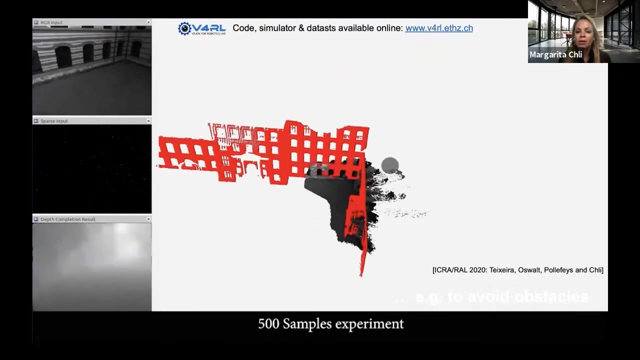 looking at that laser scan in red. This red laser scan is serving as our ground truth. We are using sparse input, sparse depth input, for example coming from SLAM, from point-based SLAM, and then we are augmenting this depth information using a trained network to come up not only with 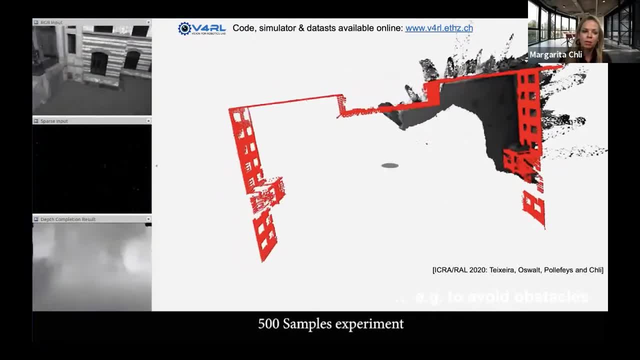 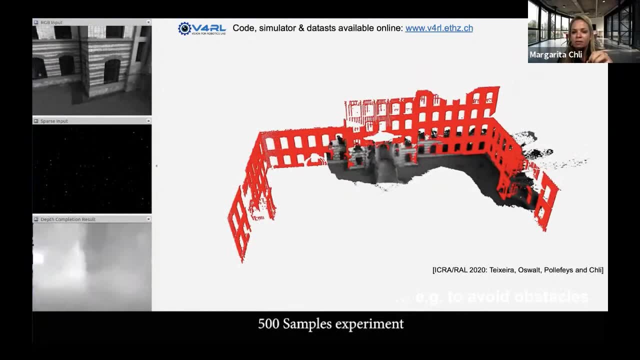 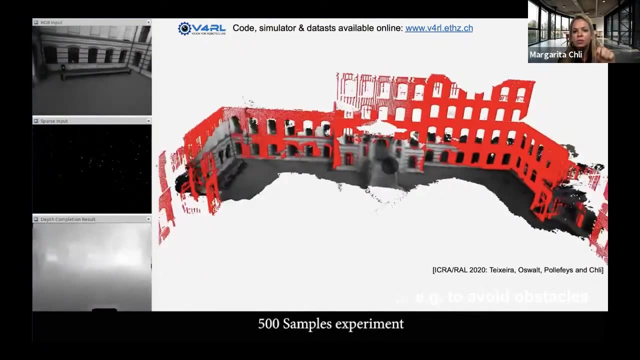 a more complete depth estimate, but also with a confidence value on how confident we are in each depth value. So you can see, for example, that as Lucas is bringing this reconstruction from a top view, you can see that through windows. we're not doing that well. 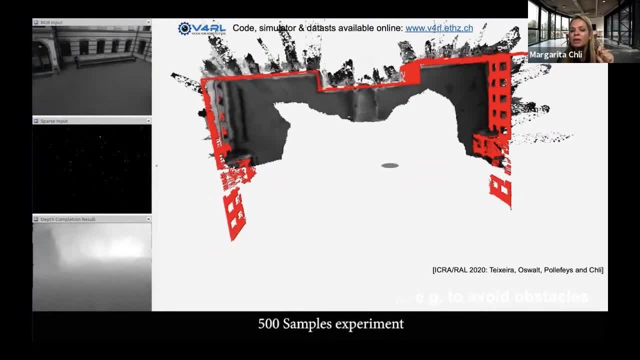 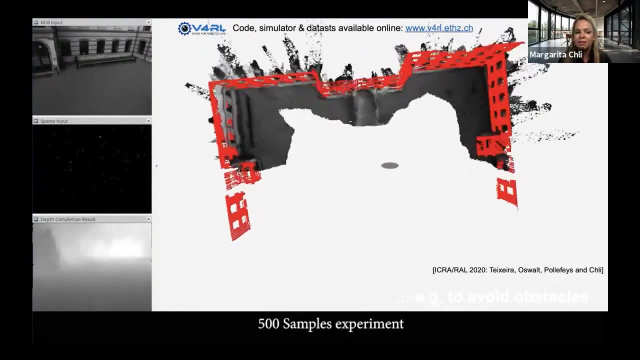 Of course this is a problem with vision, right, But this is where I would expect my confidence to be low, or around the staircase. you can see that it's a little bit fuzzy and that's also places where the confidence of your depth is not really very good. But this is very useful because 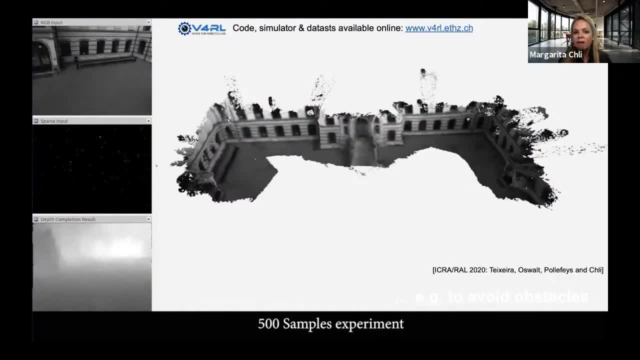 in obstacle avoidance. you don't necessarily need to have a very, very accurate 3D reconstruction. Maybe you do when you're doing monitoring of archaeological sites- but when you want to avoid obstacles you want to maintain a certain safe distance right, Maybe one or two meters away from your structure. 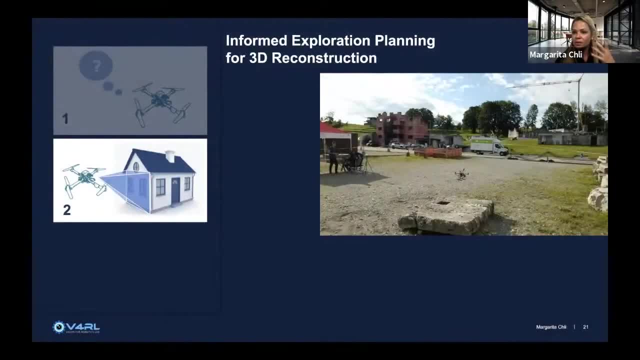 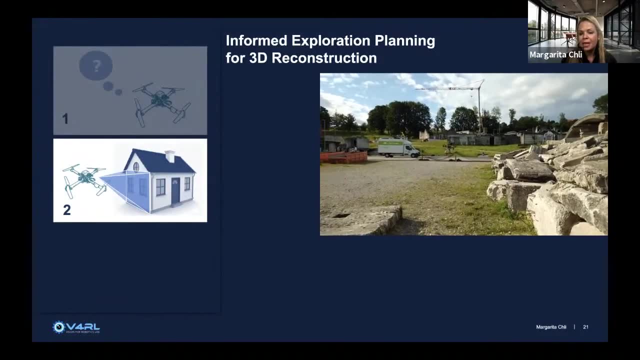 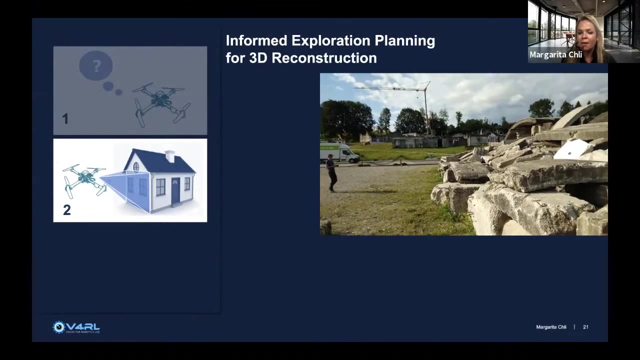 depending on what it is that you'd like to do, So having access to this confidence is important Now. with dense reconstructions like this, we can enable some autonomy, and here you can see it now in action. So this is a video captured from this summer, actually. 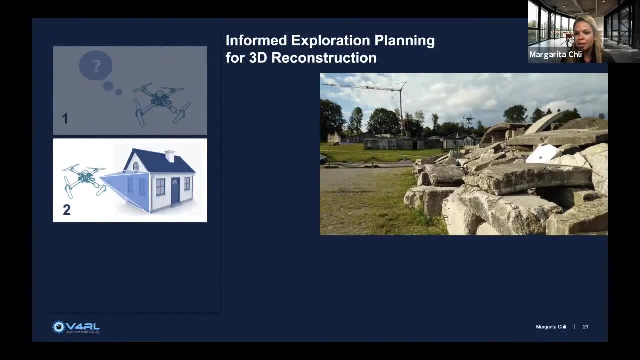 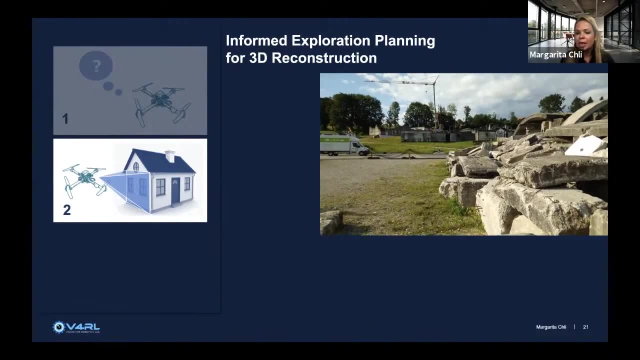 We have now a drone that is using a gimbal-actuated camera and it's tasked So it takes off and nothing about the scene, and it is tasked with coming up with the reconstruction of the scene that it is looking at. Bear in mind that these two features are not actually synchronized. 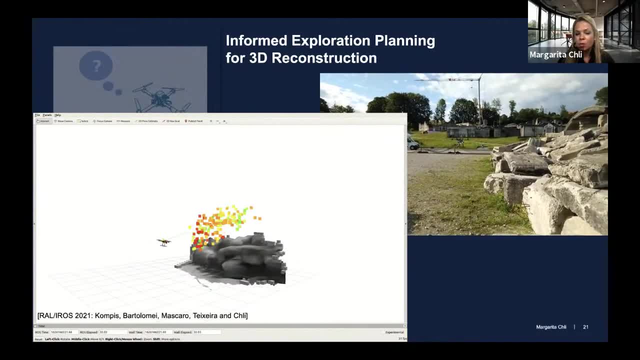 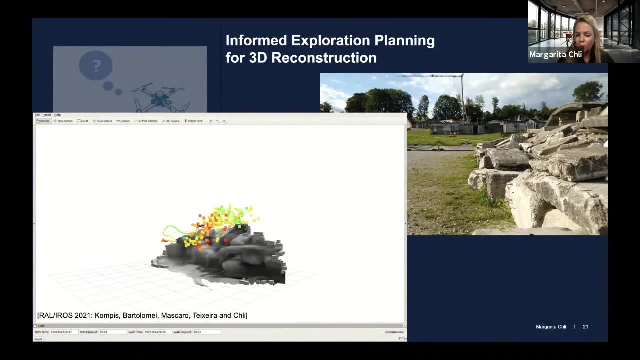 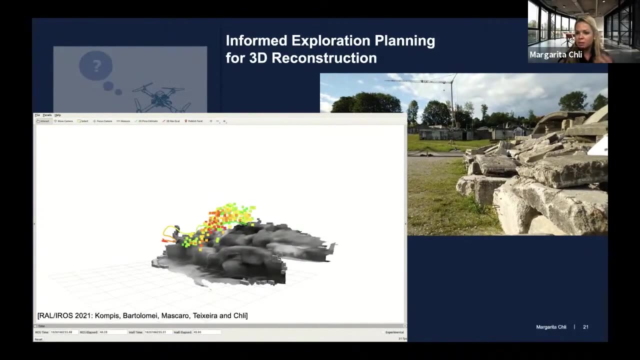 But what you're looking at is here. The drone is not piloted, but it's programmed to explore a great plethora of hostile objects in certain areas, this space, in order to optimize for the best coverage of this scene of rubble and the red. 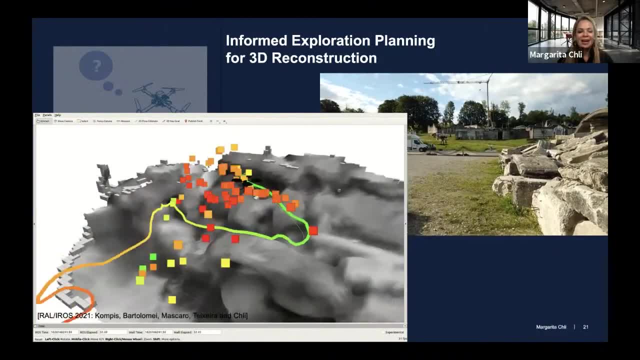 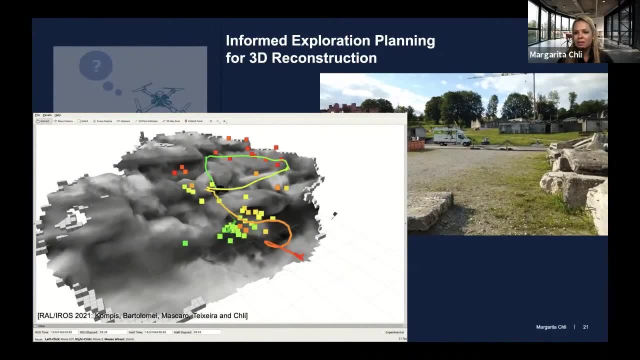 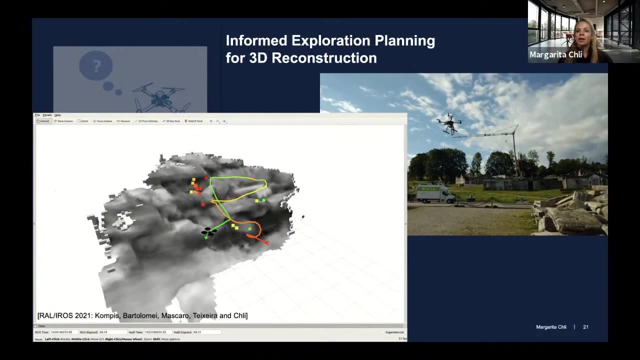 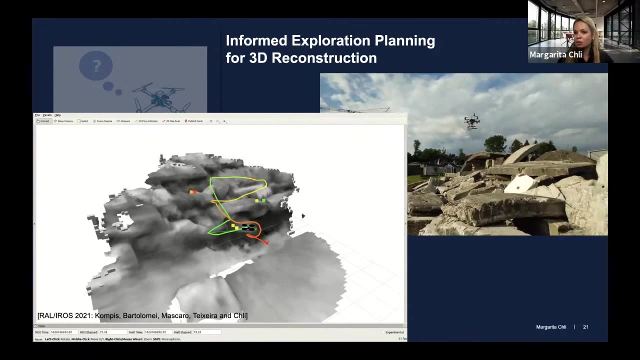 green, blue, not blue, red, green, yellow squares that you see. here are the evaluated viewpoints in the vicinity, local vicinity, of the drone, and these are ranked according to the expected information gain that they are estimated to provide us with respect to completing this, this scene, reconstruction and um. let me show you a little bit here, um, on the inside, about 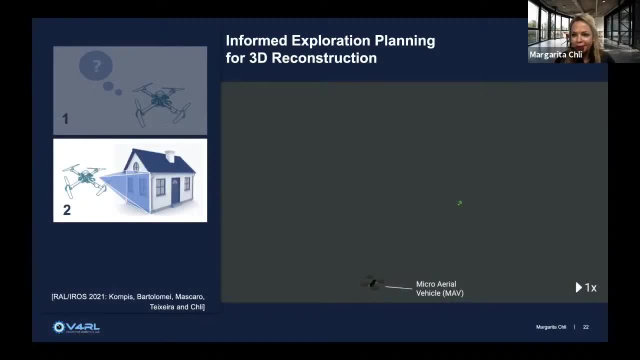 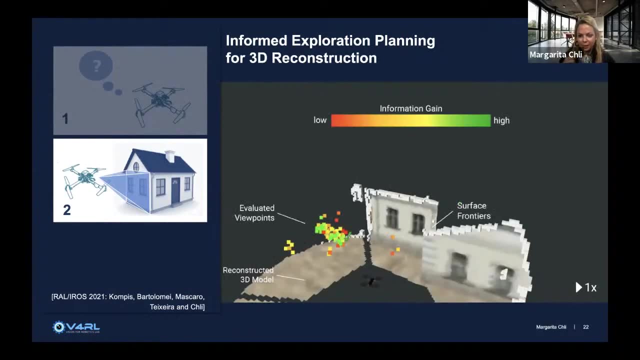 how this works, and i will let eve explain this better than i do. we present a path pattern for 3d reconstruction of large scenes for an mav equipped with the gimbal actuated camera potential. next, best views are sampled the MAV's configuration space and ranked by their expected information gain. 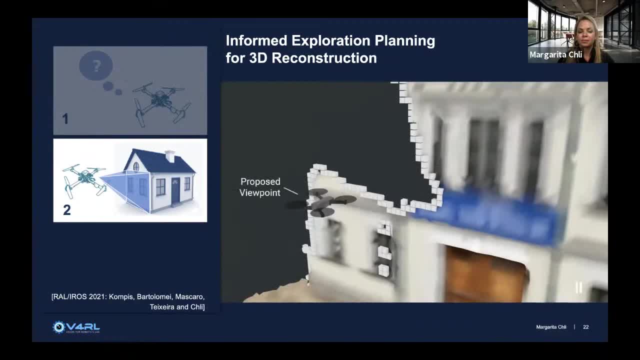 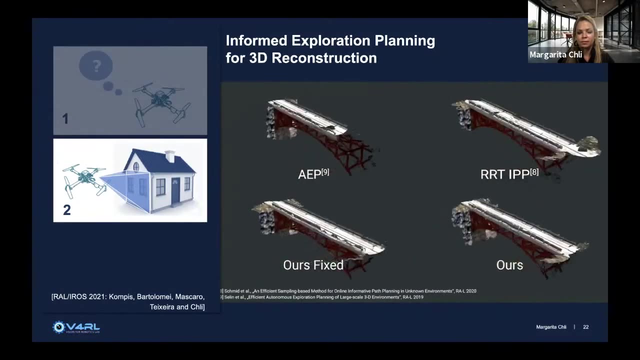 The information gain of a proposed viewpoint is calculated with the ray casting operation and encodes visibility of frontiers, visibility of unknown space, as well as quality improvements of the reconstructed surface. In this more intricate bridge scene, the actual gimbal seems to be necessary to fully reconstruct the scene. Without the gimbal, the underside of the bridge, 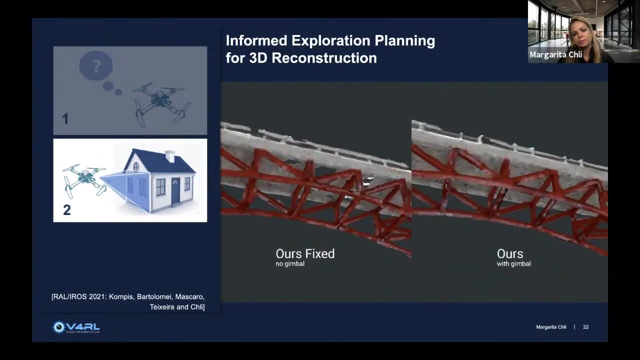 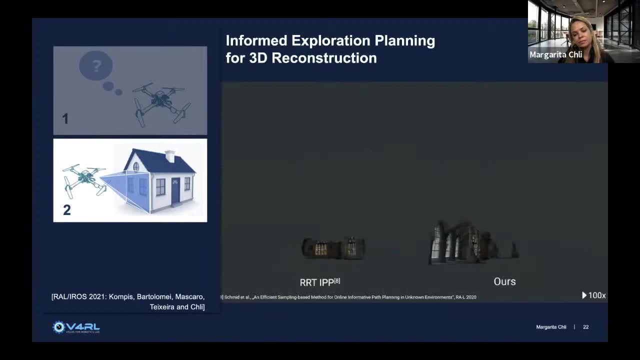 is not fully absorbable, leading to gaps in the mesh. Our planners also perform well in large indoor scenes. Not only is our approach faster, but once again some surfaces are only observable with the actual gimbal. So this was just presented at Iros and we could show that with the system we 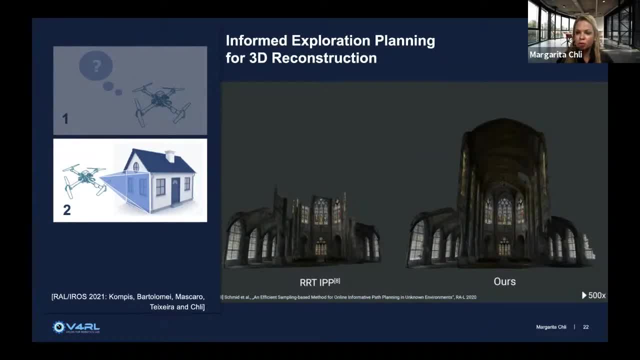 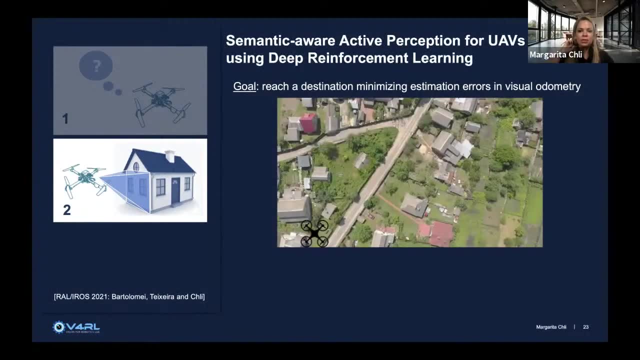 have a very good coverage and very good reconstruction quality With respect to the state of the art. and maybe one more work that was presented at Iros just now is Luca Bartolome's work on semantic aware active perception for UAVs using deep reinforcement learning, where our goal here is to plan a path for a drone like this to navigate through space. 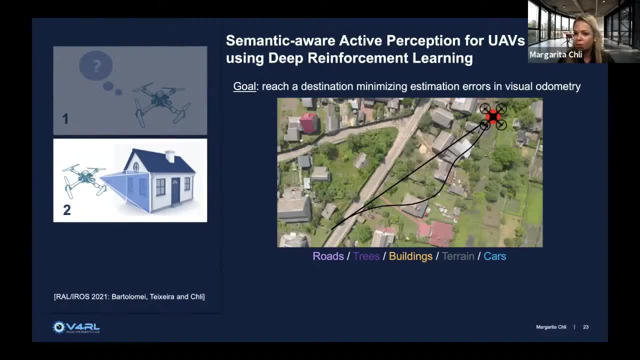 in order to minimize the estimation errors in the visual odometry. So yes, of course this can come at the cost of a bit of a longer trajectory, but the aim is that we want to avoid any areas in the scene that are bottlenecks for our visual odometry, For example. 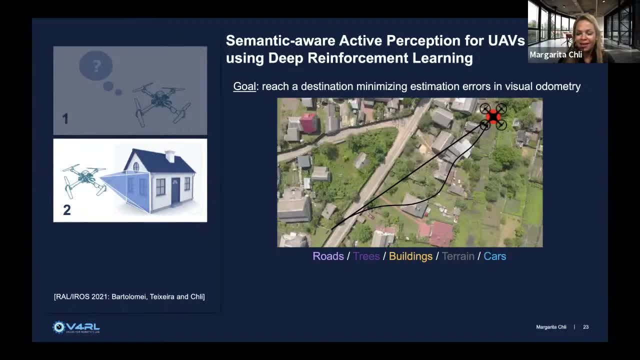 whoever has worked with water knows that water is not the best area to to look at when you want to to navigate right when you want to perform slam, or how about moving trees or cars right. so having access to such semantic labels and putting these in our optimization function of how we generate this path, then, is bound to lead to more robust. 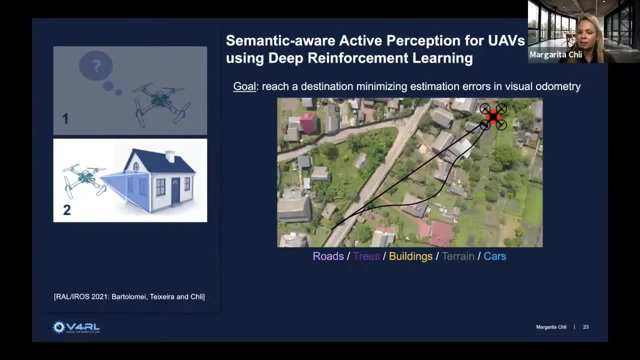 and realistically applicable paths. And just to say a few words here about the deep policy training: we are maximizing the reward in an episode-based fashion and here we're using as a reward, we're using a mixture of these three components. First of all, we are interested in the 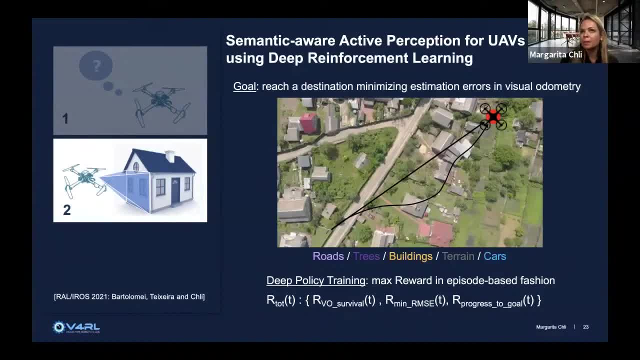 survival of the visual odometry. so we're trying to keep in the field of view as many landmarks as we can, and then we also want to minimize a root, mean, square error of the trajectory as a whole, and also we are penalizing any progress to the goal that is not fast enough. okay, So that's. 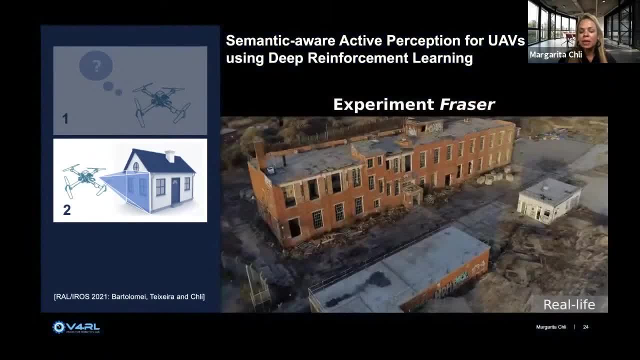 so we're using these three rewards to come up with these and now i'm going to show you some results that we have um in these examples. so you're going to see i think it's two examples is on photorealistic um simulations that we came up- uh, give up, actually it's, it's a real life. so 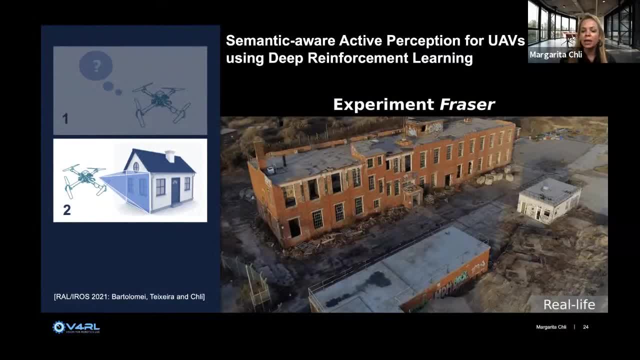 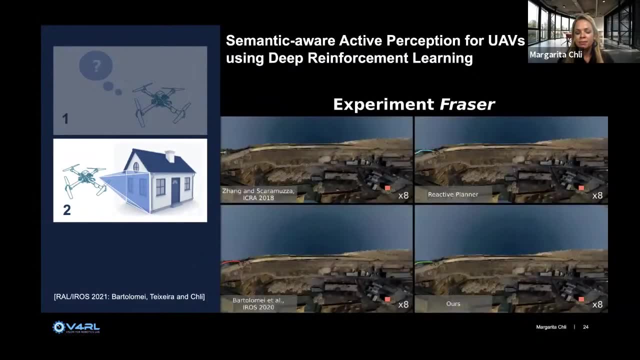 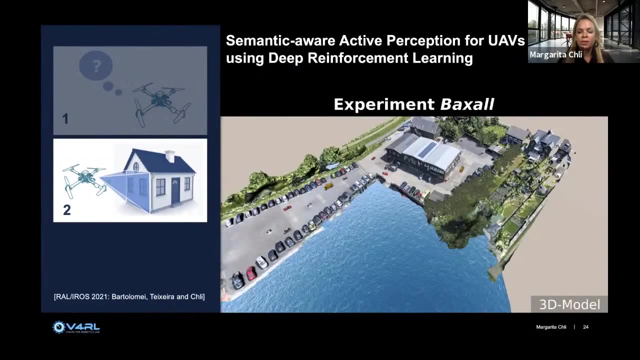 here you're looking at the real life view of the scene, and as soon as i start the video, you're going to look at them, the reconstructed view. and here it is. now we are um comparing against three different planners on the top. the top two planners have no semantics encoded in them. 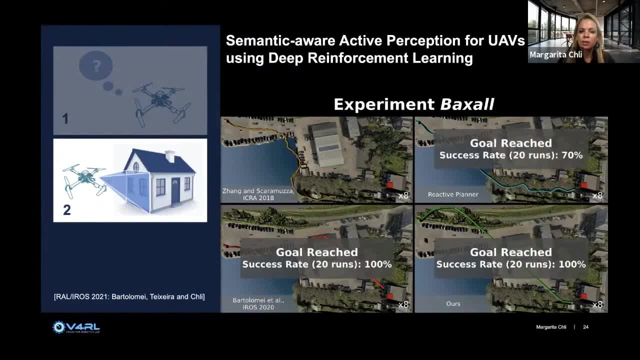 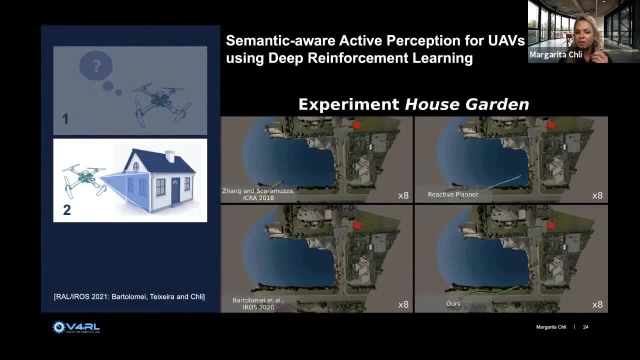 so the first of all, the first top left, is doing a lot of detours. it's using um active perception to maximize the air, the number of landmarks that are visible, but it's not really using semantics to gain the floor, to Manipulate akkorini's. 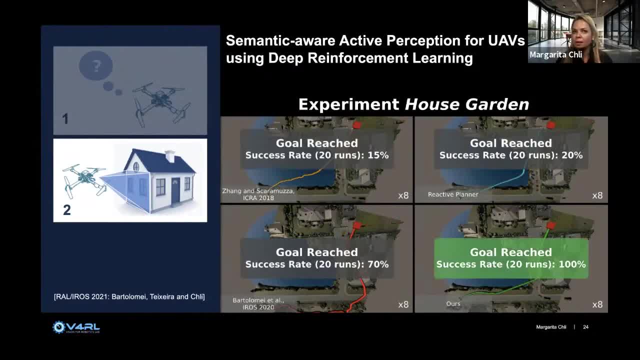 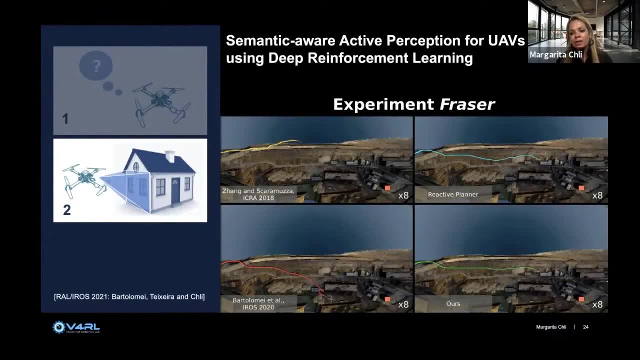 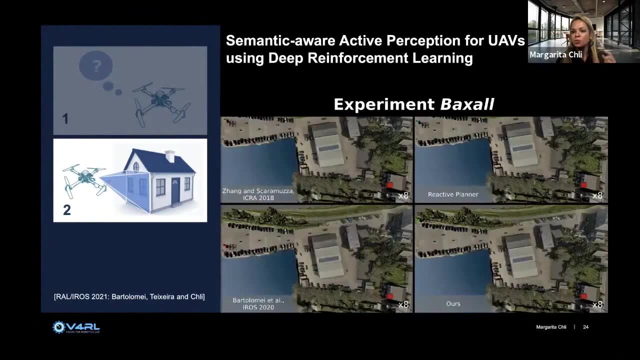 this robot towards the goal, with taking into account, really, how good the roof means. square error of that trajectory is On the right hand side, top right. there's no perception that is taken into account. So this is a reactive planner that is trying to reach the goal as fast as. 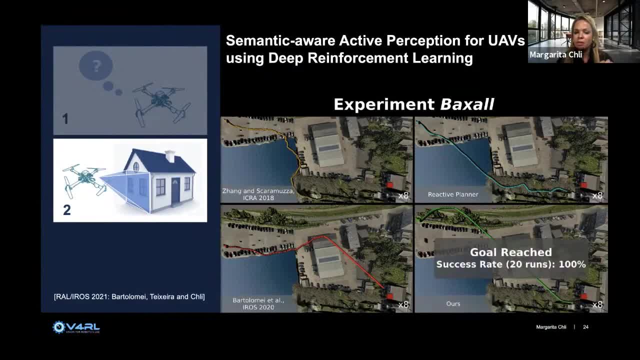 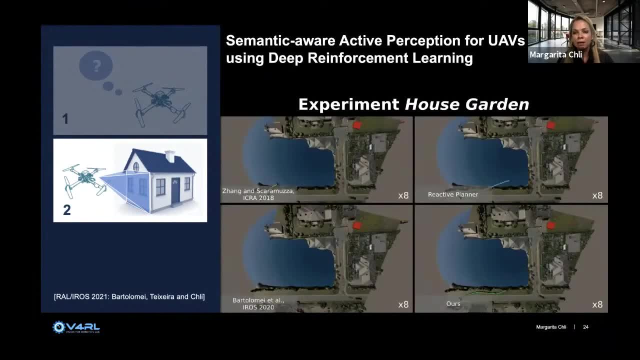 possible. On the bottom left we do have semantics, So this is our previous work, But in this case, semantics, we're basically having a binary weight right, a zero or a one of being a safe or unsafe space to navigate through or navigate on top, actually, And on this new work that you're 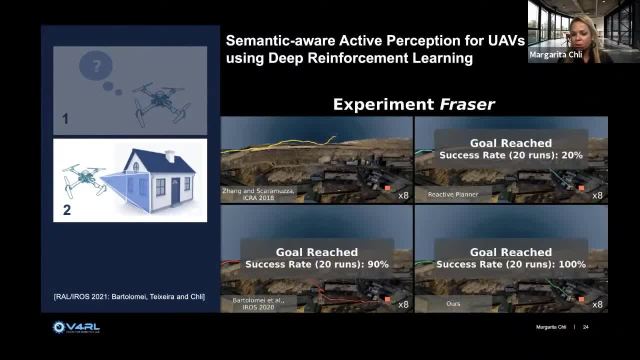 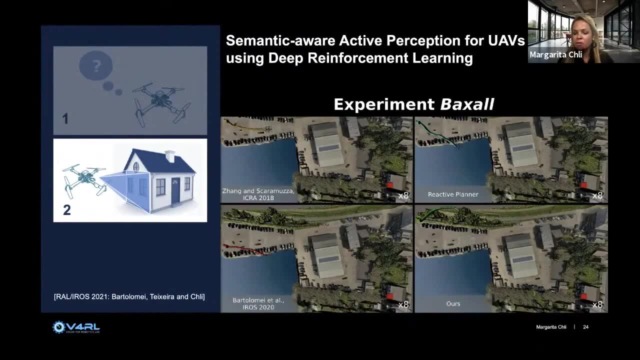 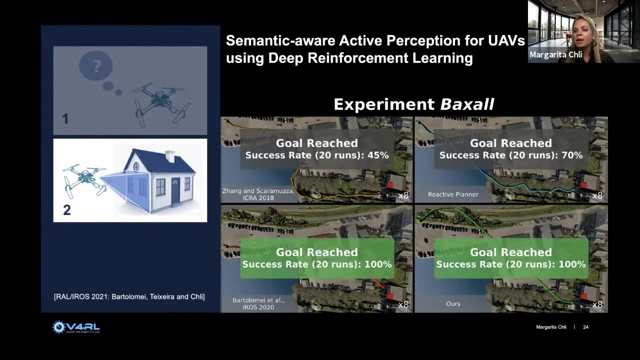 seeing on the bottom right we have the best performance because we're actually adapting the relative weight of how good or bad an area is to navigate on top of right, because sometimes, when we're we're when a road is very busy, it might be a good idea not to navigate on top of it, But if the road is 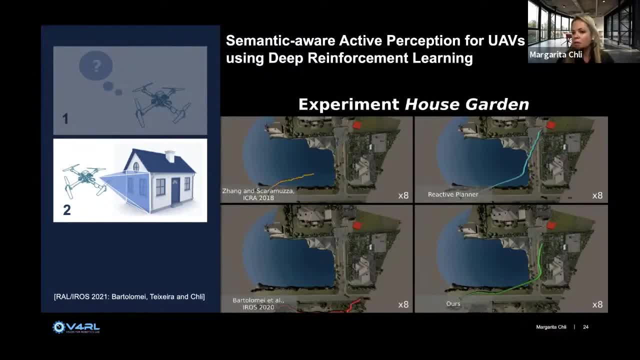 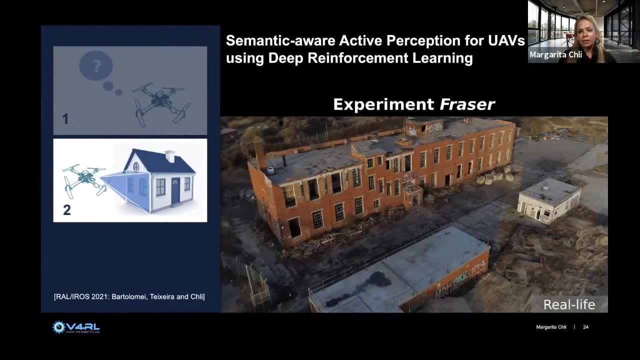 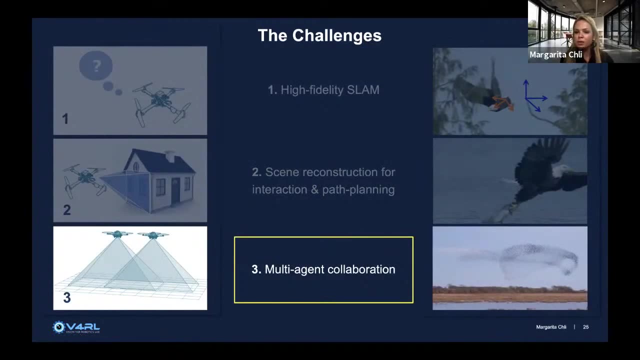 empty, for example, then it doesn't mean that it's not, it's not a good area to to use to localize from Right. And with this I'm coming out to the final challenge, the multi agent robot collaboration. And in order to explain to you our contributions here, I want to zoom out a little. 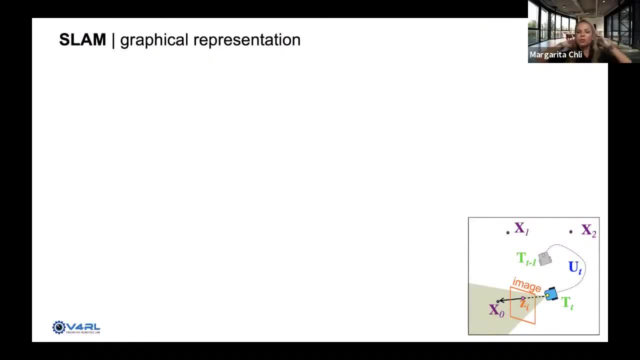 bit And talk a bit about SLAM in general. So we're going now into the basics of SLAM. Okay, So I'm going to show you the graphical representation of SLAM. I'm sure some people have talked about this before But again, I think it's always useful to to see how someone else is explaining it And 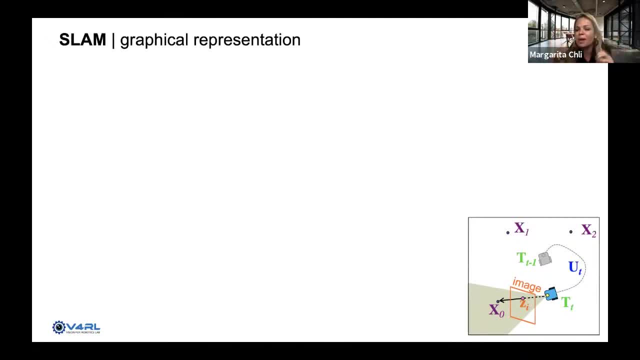 hopefully you get something and put the bits and pieces of your puzzle and come up with a very good view of what the SLAM problem is and what it's trying to do. So here we're having some 3d landmarks. I named them X, And please consult this legend here on the bottom right where I have this. 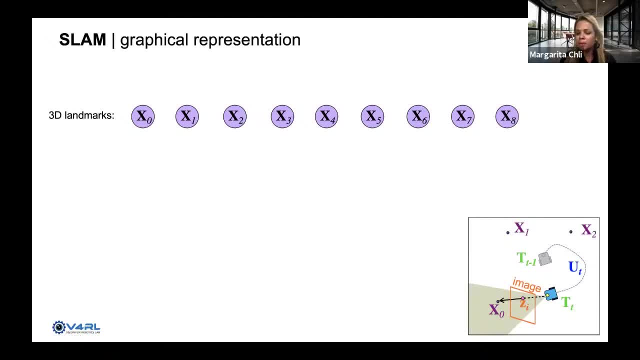 simplified room, right where we have a robot, we have a few landmarks. this robot is equipped to the sensor, let's say a camera, and it's able to view, experience these landmarks through this camera via images right So back to our graph structure. we have our 3d landmarks here as nodes. 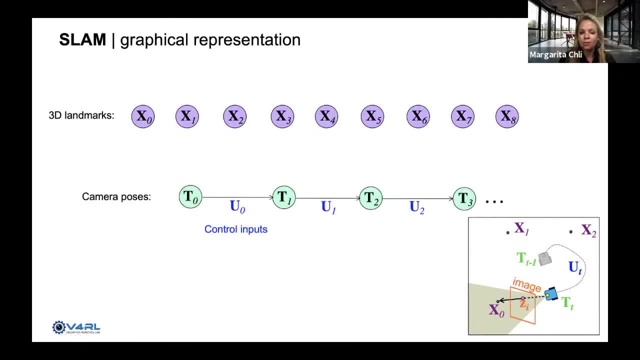 X And these are the camera poses that they are related. In this case, I'm assuming I'm having a ground robot And the camera poses are related with respect to the control inputs of how the robot has been moving right, move left or right forward. And now, how are these landmarks related to the camera? 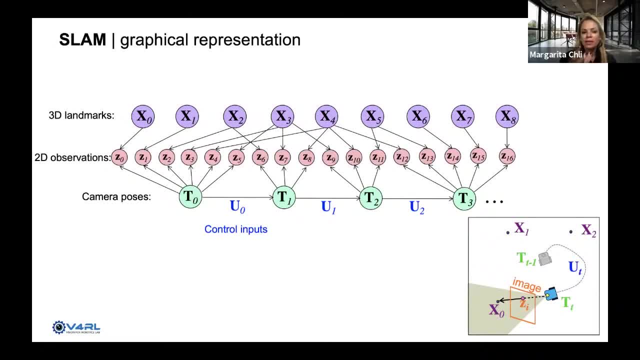 poses. Well, they are related with the experiences of these landmarks through the images, right. So these 2d observations, these Zs have here, As you can see, I have a lot more Zs than Xs, because you can observe the same landmark from: 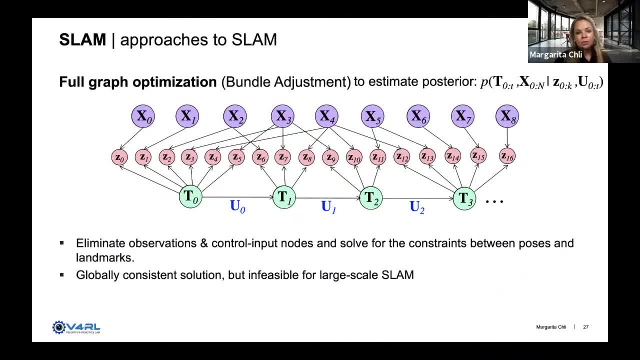 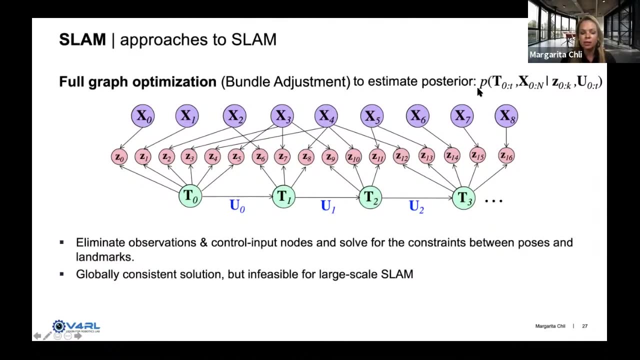 different viewpoints right Now. how do we go about solving this problem? Now in the, we know that the best solution for for SLAM is the full graph optimization, what we term as bundle adjustment, And it's basically trying to estimate this posterior right here. So the way that we do, 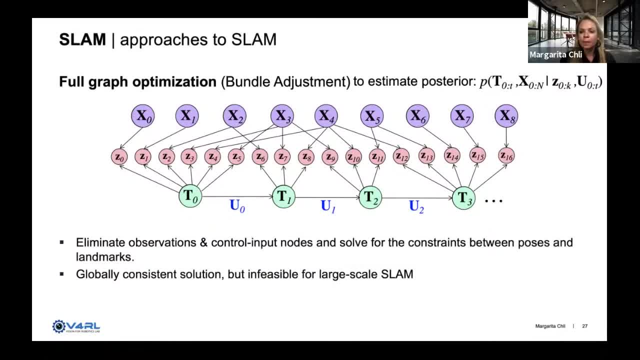 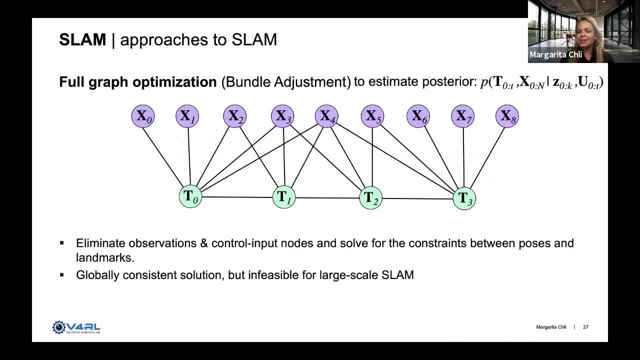 this is that we marginalize out the, the variables that we know about, And then what? what remains is direct constraints amongst the notes that we're trying to figure out, And you can imagine that this is: instead of looking at lines, imagine them to be springs. So here I have a network of springs, Every pose And every landmark. 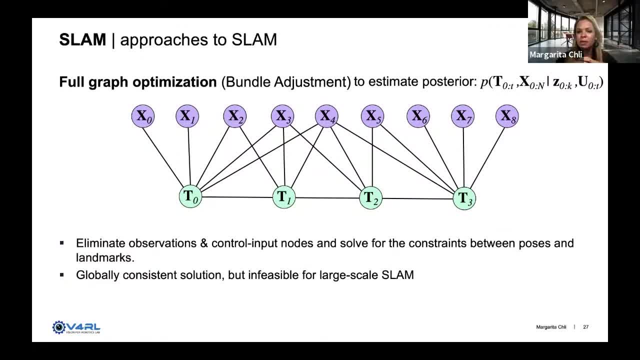 wants to pull and push their own way, But the full bundle adjustment is actually coming up with a steady state of the full bundle adjustment is actually coming up with a steady state of the cool, cool, cool, cool, cool, cool- this network that you are looking here. 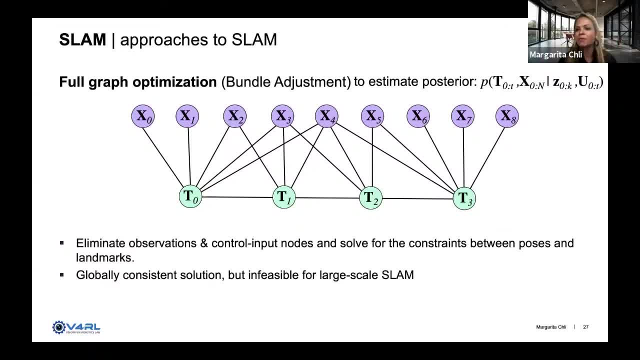 So this is the best solution that one can have with this data right: To come up with a globally consistent solution. But of course you can see that this is largely infeasible when we start adding more poses and more features and landmarks and more observations. 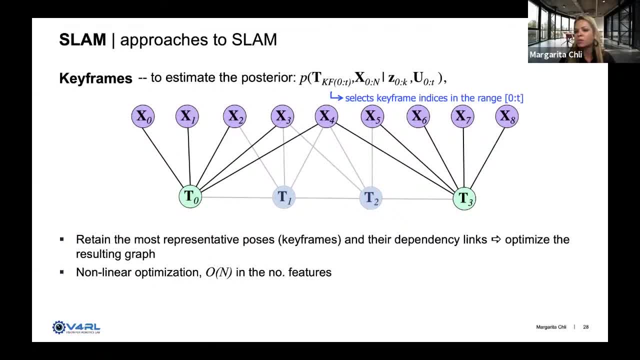 So for this reason, we're coming up with the filtering approach to approximate this, as you've seen in previous lectures, but also with the key frame based approach that is turning out to be quite a lot more popular these days, where actually what we're doing? 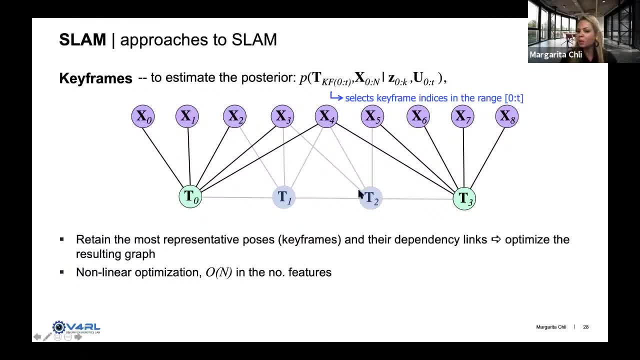 is that we are choosing to ignore some intermediate poses and retain the most representative frames, the key frames. Now, what makes a good key frame is subject to research, I would say. So far, it's largely been people resort to ad hoc metrics to, for example, the co-visibility. 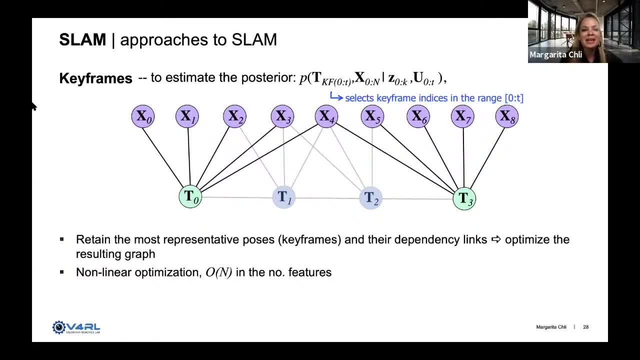 of features, right. So let's not go into details of this, to remain on point. But the idea is that we want to estimate this posterior now. So we want to estimate all of the poses, camera poses, all of the landmarks, when I know the observations. 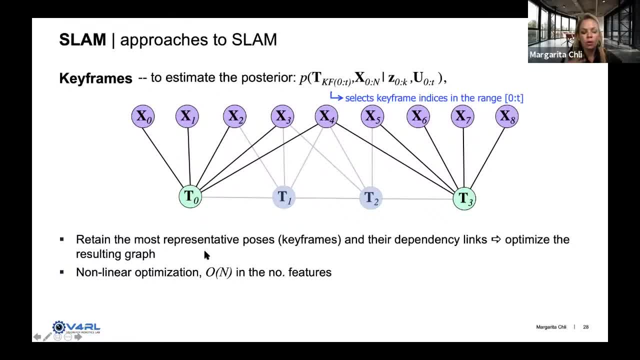 and the control input right, And so we're optimizing now the results and we're looking at the result in graph using non-linear optimization And that scales much better with a number of features than the full problem that we've seen before, Right. 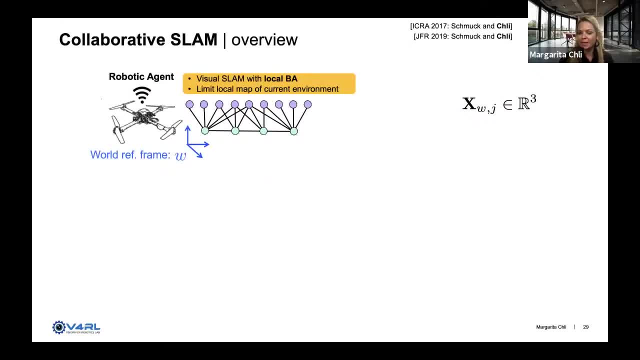 Now, with this in mind, let's look at how we can build collaborative SLAM. But first of all, some notation. So imagine here that you have this drone and it's building up a map of its environment, of its surroundings, right? 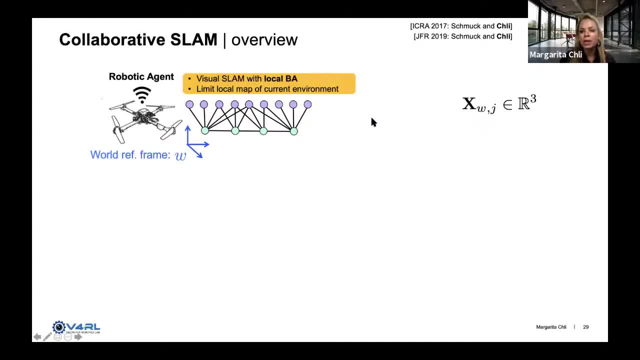 So it's a little bit of a and the same map structure that I've shown before Here. x is a three-dimensional vector and I reference it with respect to the world frame And j is the jth landmark right. I index it on the landmark. 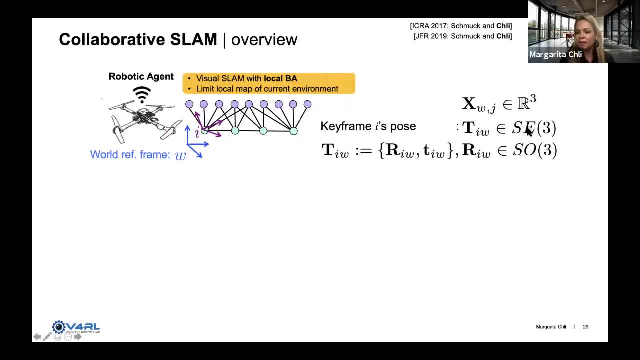 Now we also want to define the keyframe poses. If you're not familiar with the Lie group, then don't worry too much about this. The keyframe pose would be a transformation with respect to the world frame right. So I say that my keyframe is actually. 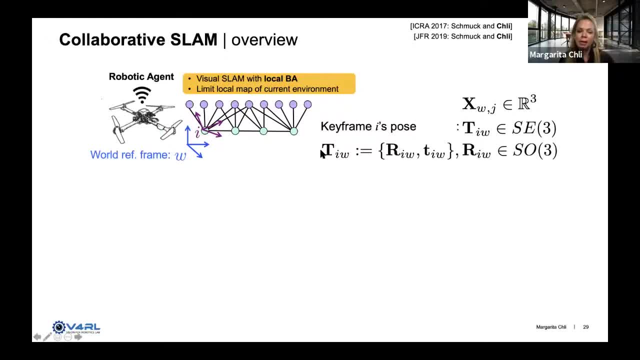 a new frame of reference, and t is my transformation to that. It's a rotation matrix and a translation vector from the world to the i-th keyframe, And the objective here is now. I'm just putting in an equation what I said in words before. 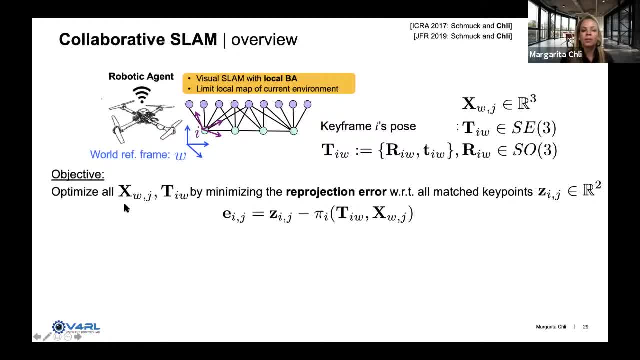 The objective here is to optimize all the landmarks and all the camera poses by minimizing the projection error of these landmarks with respect to all the matched keypoints z's- Remember the z's that we've seen before, And so I have a projection function. 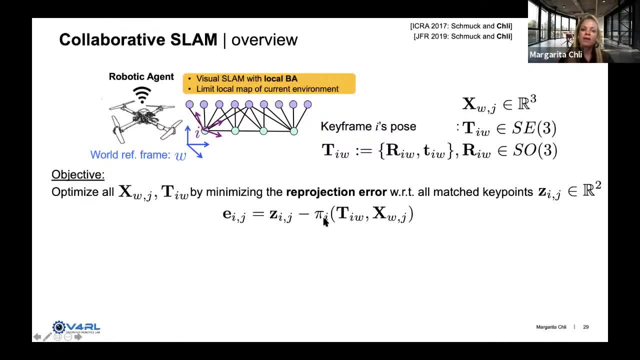 Again, there are projection models for your favorite camera here that take a landmark and project it to the image of this keyframe from this pose and then subtracting it from the actual observation to come up with this reprojection error. And then the idea is that we want: 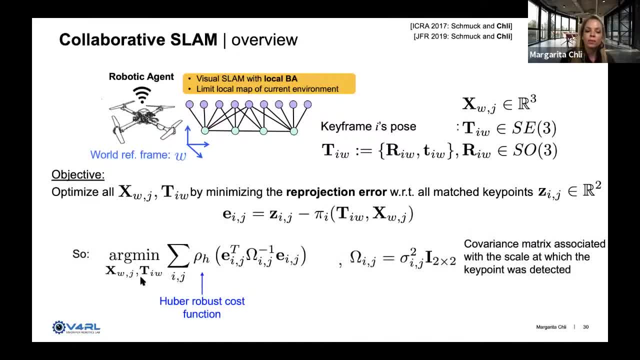 to minimize the sum of the Huber-Loss function of the squared reprojection error, that they are scaled with respect to the covariance matrix of where that keypoint was detected right. So now imagine that you have one robotic agent that is running Visual SLAM and is 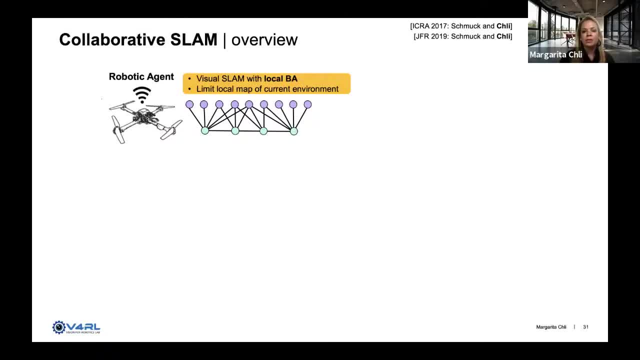 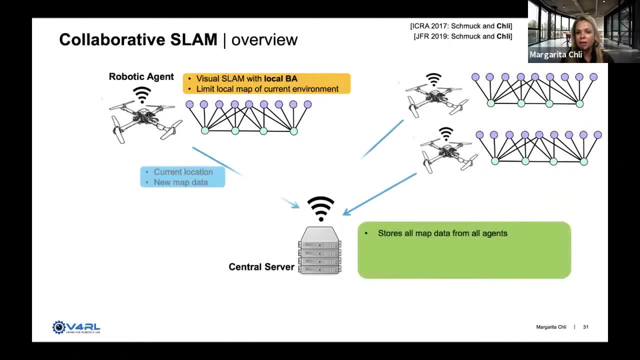 doing all this local bundle adjustment all the time. Then imagine that you have more drones that do exactly the same thing. So to do collaborative SLAM, what do we do? We are saying right. I know that. I know that at some point you need to keep forgetting. 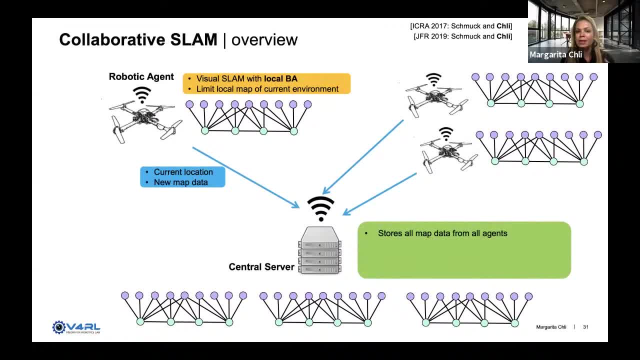 You need to start forgetting about your past camera poses and your past experiences. So, before you forget, just send all your data down to a central server- Or, if you'd like, this could be the cloud as well. So, basically, this central server. 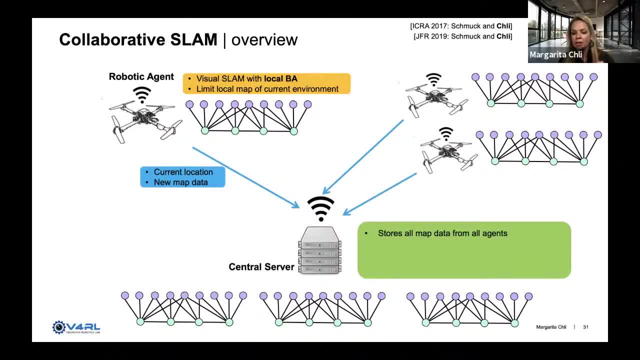 keeps a copy of all the experiences of each agent. It's acting a bit like a bookkeeping entity Now, because this is also a very, very, very complex system. it could be an entity that has a lot more computation than on board the central server. 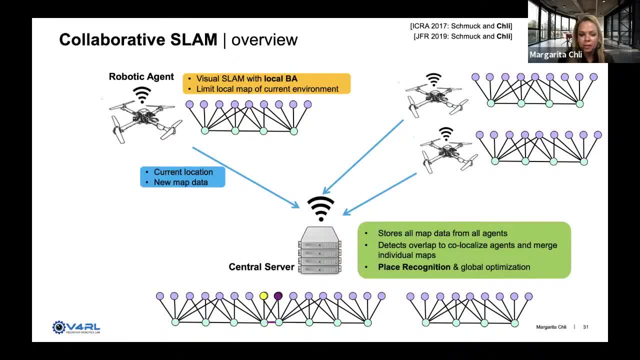 We are running more computationally expensive things. That's also what I replay, what you've seen before here. This is the loop closure that, in this case, I simulate to be detected between two maps, right? So here we have seen two maps that. 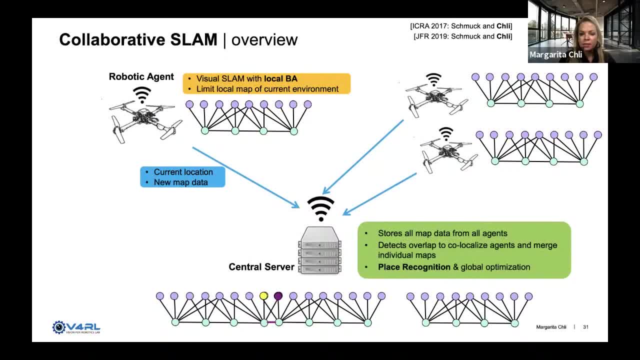 are merged with each other And we have new links inserted And in such cases we run- We run the optimization, global optimization- on the central server And then we can inform any participating agents about any changes that have happened in their local vicinity that would be relevant to them. 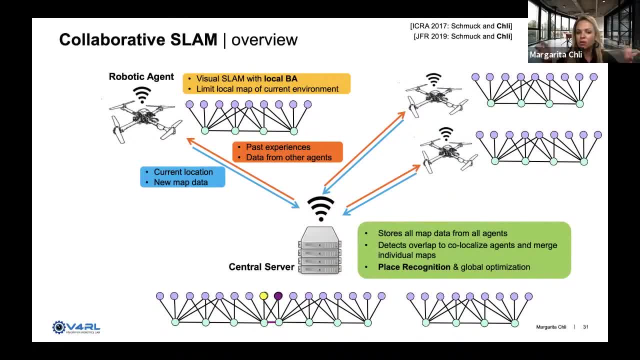 Right. So again we have multiple agents that we are assuming that they don't have a lot of computation, but they do have some computation on board, And we have a central server which can be a standard desktop or laptop, actually, or the cloud. 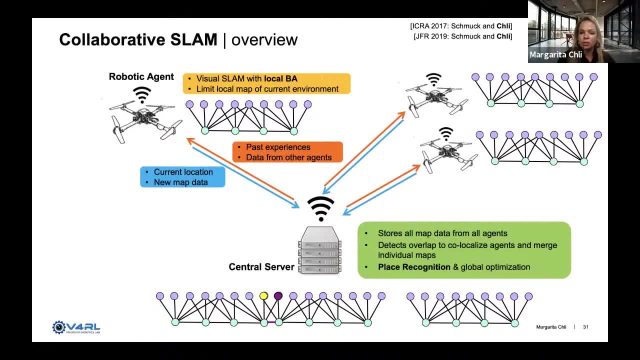 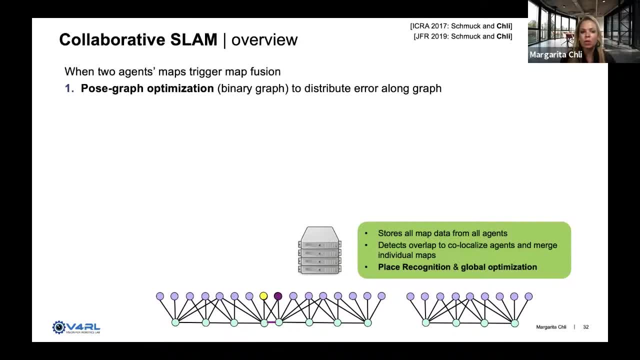 So we're doing all the map merging and global optimization before informing these agents. So let's look at this optimization, What happens at place recognition instance, Right before we go ahead and optimize the whole thing. it's a well-known strategy that it's. 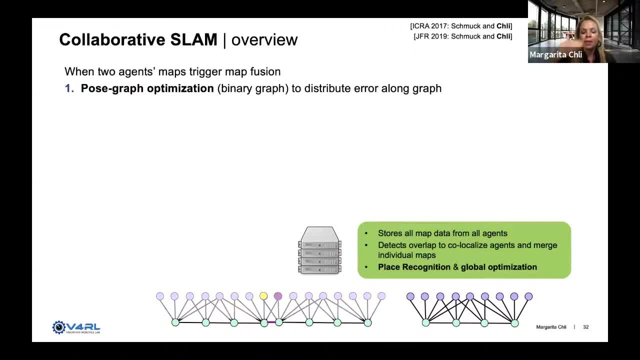 good to do post-graph optimization first, by not taking into account the features, the landmarks, for the moment, and only taking into account these poses. right To do post-graph optimization to distribute the error along the graph that is introduced by this new link. 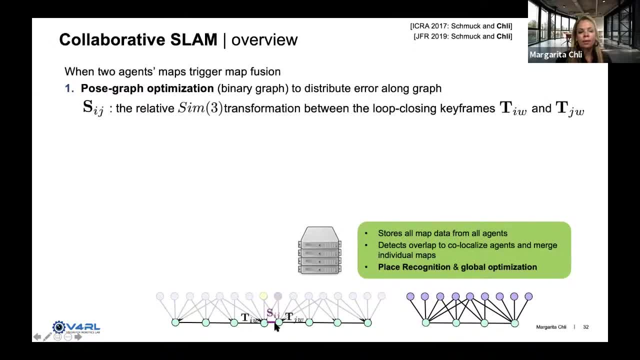 that I just added from my place recognition. So let's define this Sij, which is a similarity transformation, which is basically a rigid body transformation as Te's, but also has a seventh dimension for scale Right. So this is the similarity transformation. 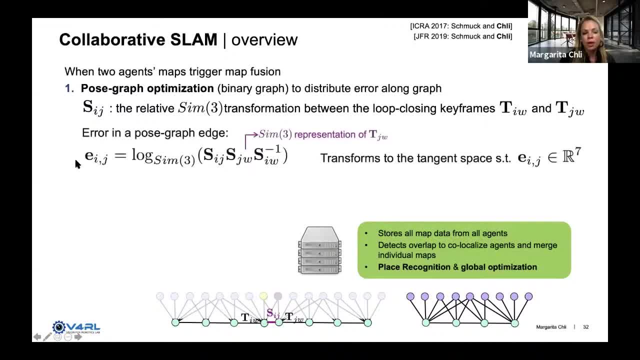 between two closing keyframes. And now I'm defining this new error, that it should again sum up to one, which is this circular error. I call it because we are multiplying all these errors that should accumulate to something that's close to zero or zero actually. 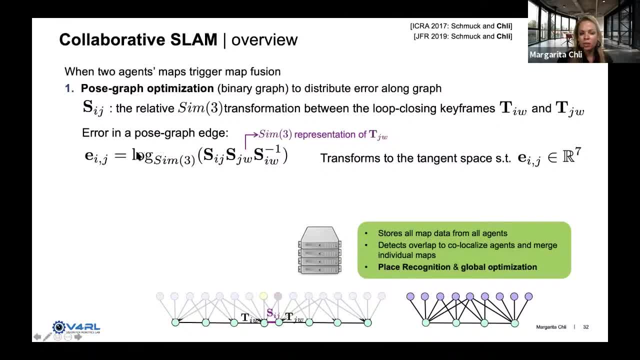 And again, don't be confused by this notation: This is a function that is transforming my error to a seven-dimensional space, So this is a seven-dimensional vector, basically. So, defining my errors like this in order to do post-graph optimization, we 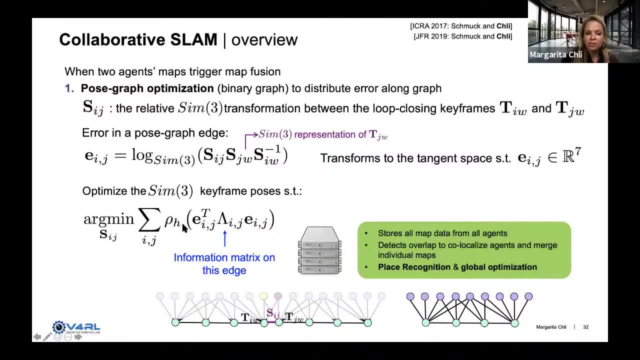 are minimizing this Hooper loss function, the sum of this Hooper loss function of the squared, such circular errors that they are weighted with respect to the information matrix on this edge, And once we come up with the first error distribution on this post-graph, then we are running full global optimization, which is 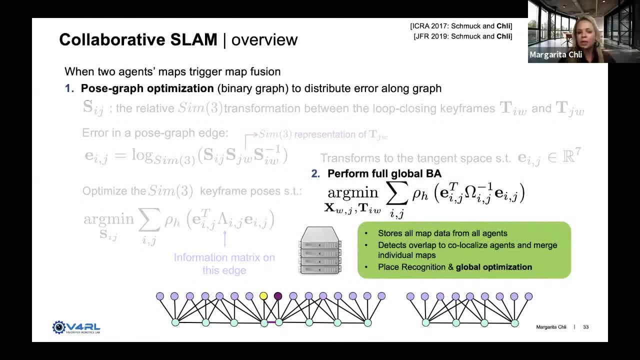 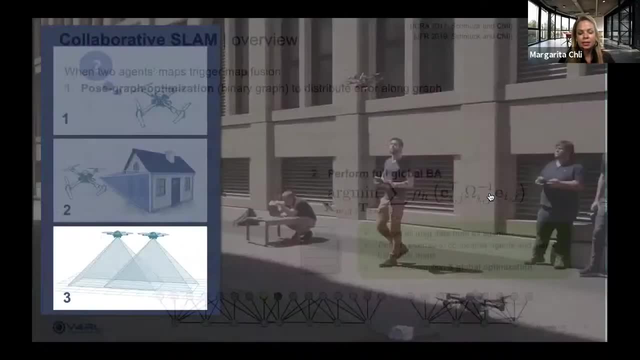 exactly what I've shown before. Now I'm taking into account the whole thing. So this is the full global bundle adjustment that I was talking about before, And that's exactly the same minimization that I was doing in the slide before. And let's look at this system in action. 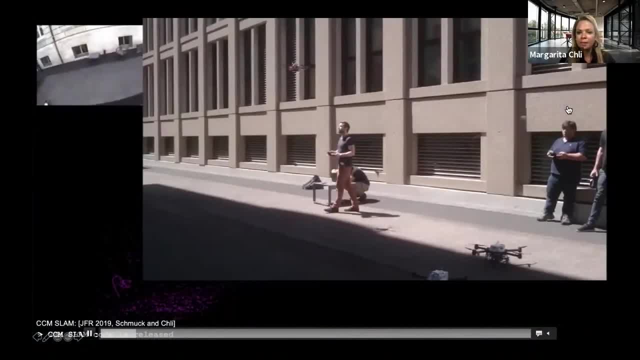 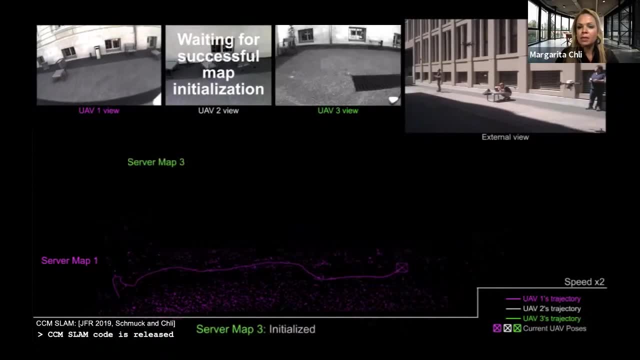 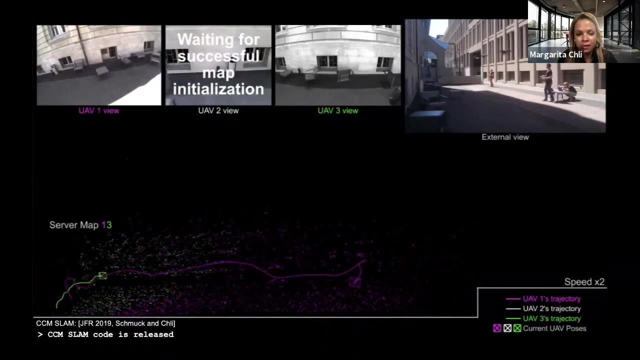 So here you're looking at my server. Here is a standard laptop. We have three drones and three pilots. My drones here are not autonomous. That means that each pilot is piloting one drone, And bear in mind that they take off. They know nothing about each other. 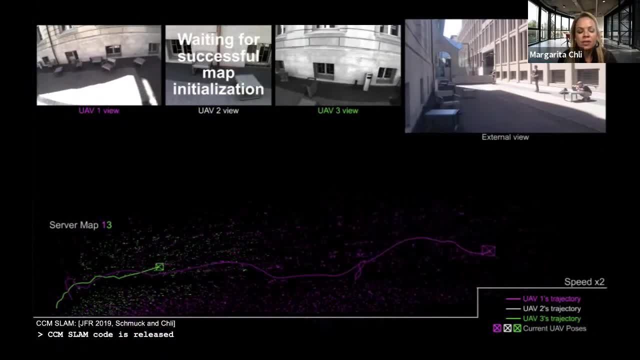 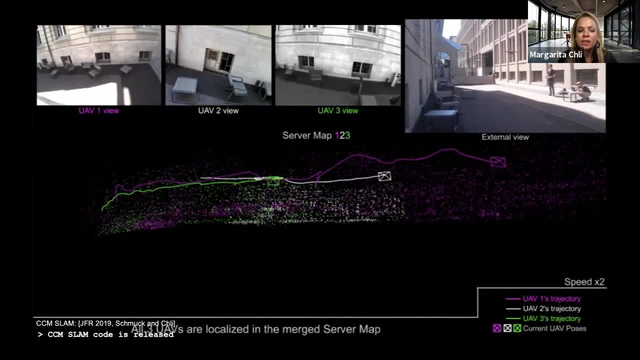 They don't know how many there are, They don't know where they are, So they start mapping their environment. But of course we are navigating their paths in such a way that they experience overlap And you've seen that progressively, these maps. 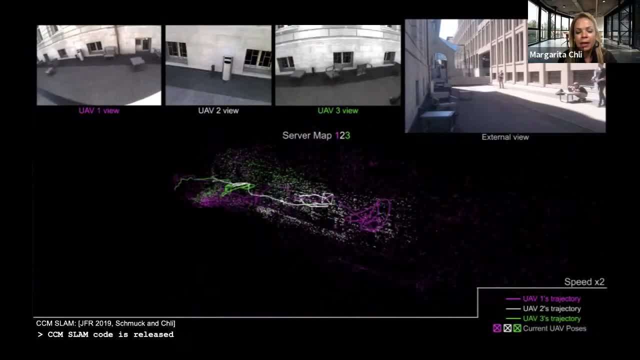 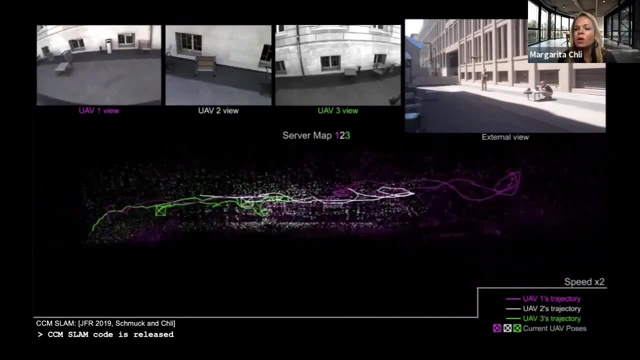 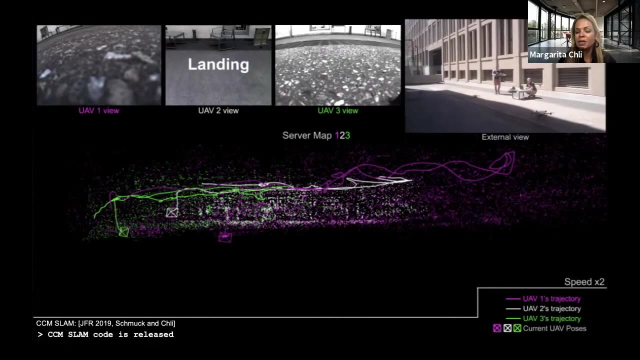 have been merged inside the server and optimized such that then all these three drones operate within this map. So where does the collaboration come in? Well, once these drones start to navigate in the same map, they actually exchange information about their scene. 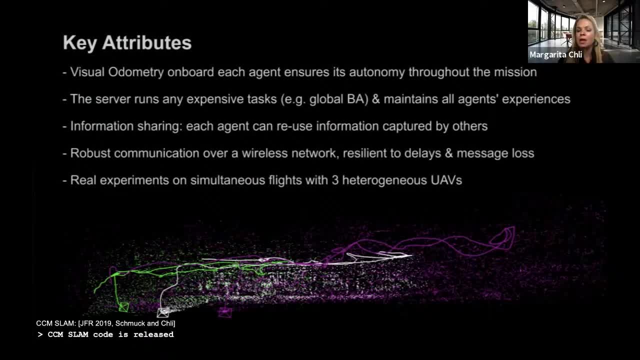 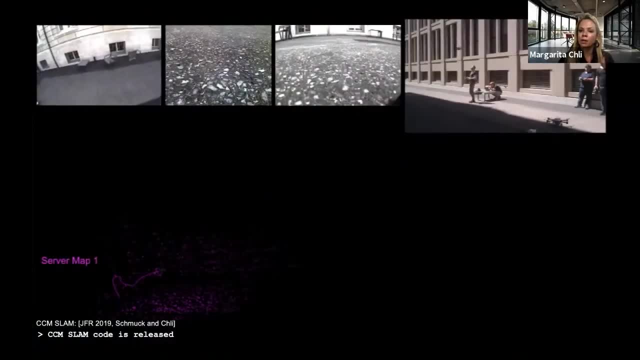 So one drone can navigate to a place where someone else has been to before, So it doesn't need to run a SLAM from scratch, But it's actually doing localization of a known map. then right, And so here we are, running localization, not only. 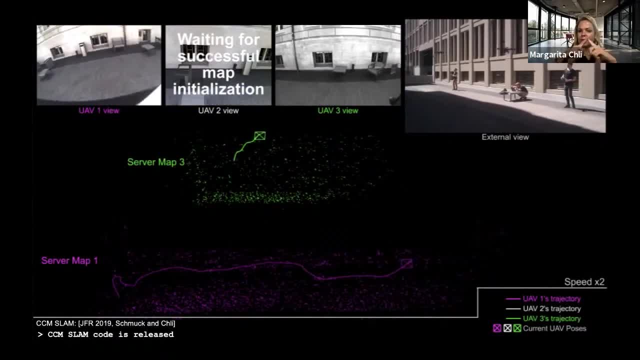 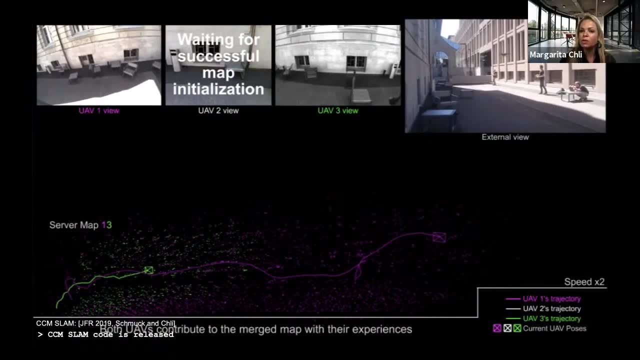 within the trajectory map Right. It's a trajectory of one drone, but also multiple drones to have to experience this overlap, And it's important to say here that, in the best case scenario, communication works well And we have a well collaborating and communicating team of drones. 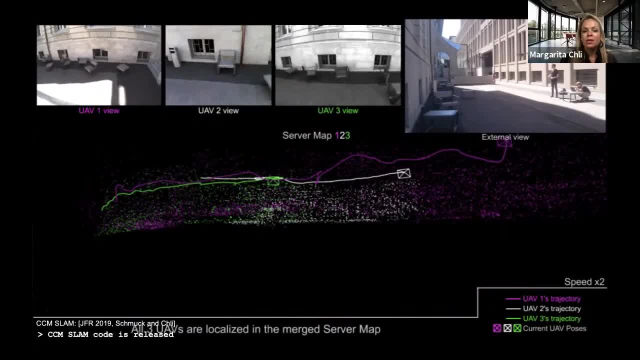 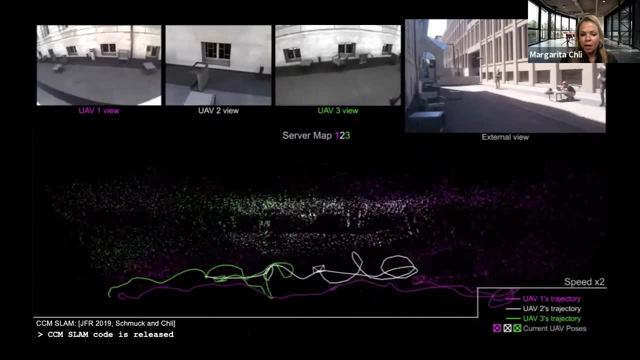 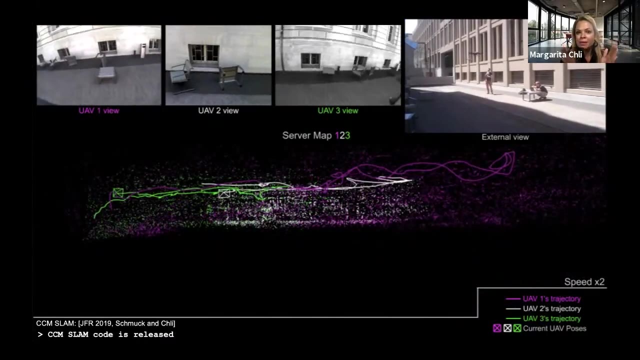 But in the worst case scenario where our Wi-Fi doesn't really work, then this reduces into a system where it's a sum of its parts. OK, So it's really three drones performing SLAM independently, individually And with a more limited time horizon. 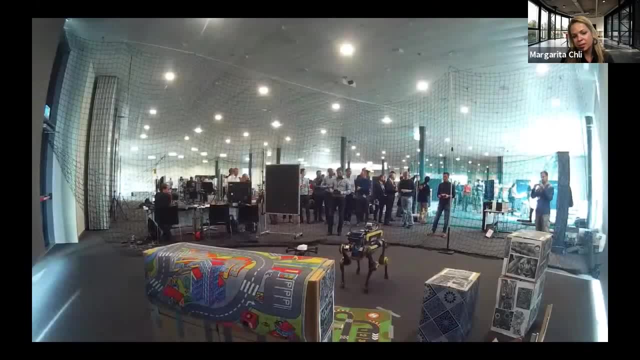 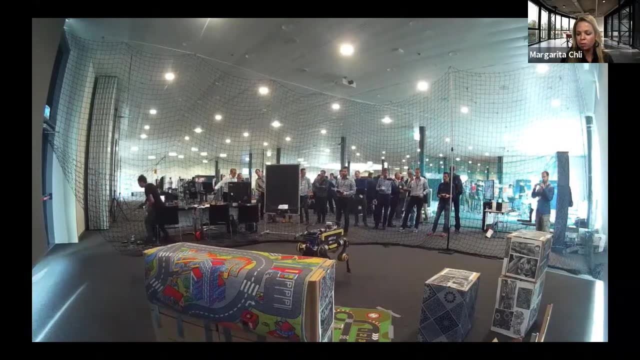 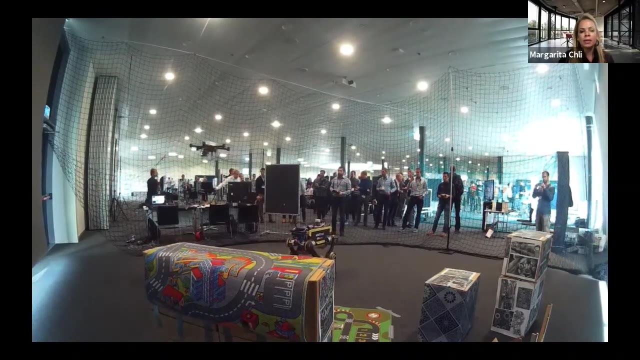 Right Now we have taken this system and we've expanded this to not only use monocular information but also monocular inertial information. And here you're looking at the same system ported on a ground robot and our drone. They're viewing the scene. 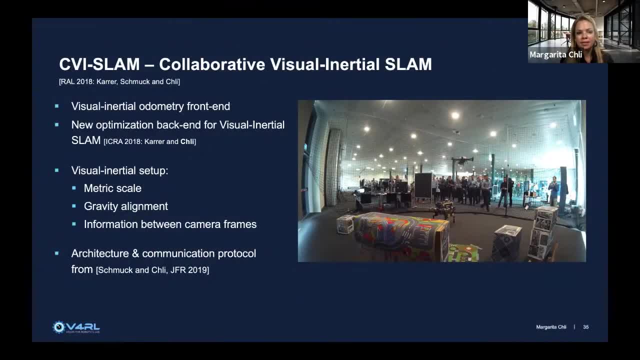 So the first version of this work, we called it the CVI SLAM- called the CVI SLAM- Collaborative Visual Inertial SLAM, Where of course we have visual inertial geometry front end And then, using this inertial information, 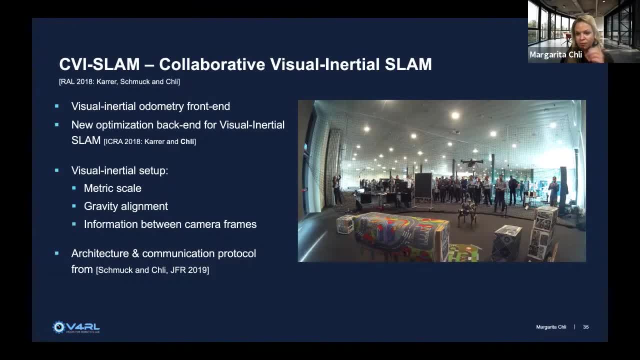 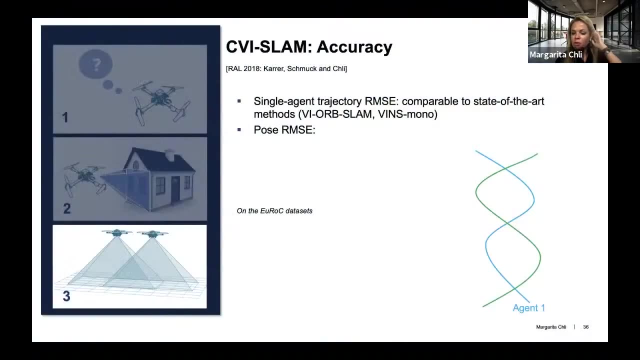 then we can have metric scale and gravity alignment And, of course, information in between the camera frames. But overall this metric scale can also enable autonomy Right. But the architecture and the communication protocol is the same as we had before. And just to share with you some insights about why, of course, 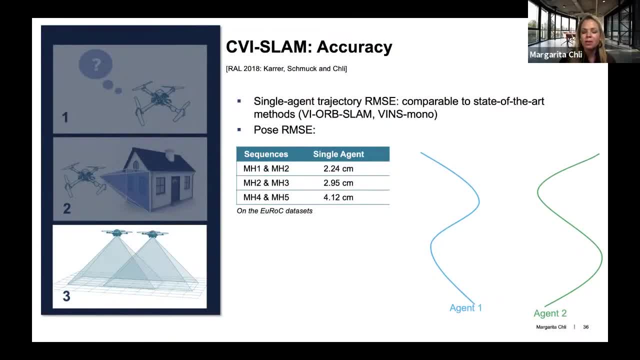 collaboration is important, It is intuitive, but it's also cool to see this in action. So here you're looking at some results. root mean square errors when considering data from the Europe. data set when considering them individually, Right. So the bigger the number, the worse the error, of course. 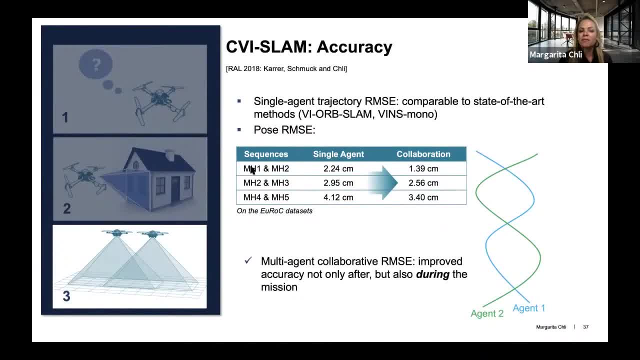 But when we consider them in collaboration with each other, so as if they've been captured Simultaneous, right At the same time, then the root mean square error, for the same sequences goes down. So this is really comes to show you. 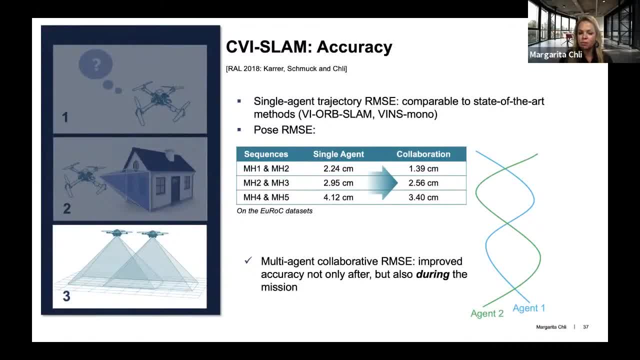 that, with multi-agent collaboration, the RMSE is improving not only after the mission- So not only after you land and optimize over all of your map, but also during the mission, which is very important, Because during the mission, you have access to more than your own data. 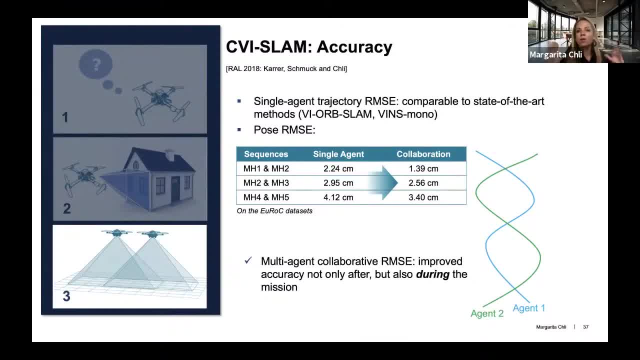 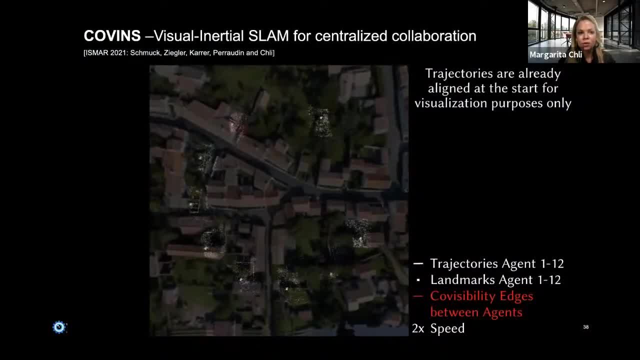 So you can be much more accurate than by incorporating your own data alone And just to do some advertising here. So this is the latest version of our collaborative visual inertial, SLAM. This is open sourced. It's already on GitHub. I promised Patrick I'm going to upload a page on our lab page. 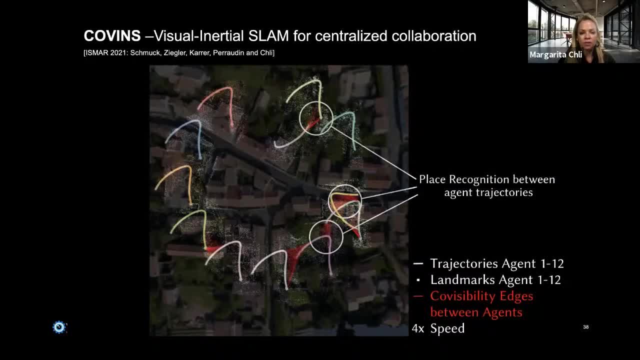 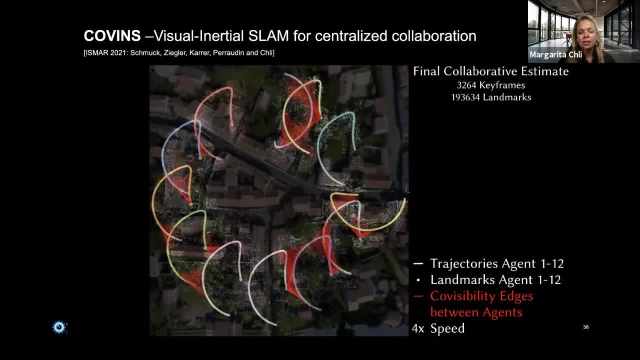 to advertise this properly. But this is Covins. So here you're looking at it in action, With 12 agents in the loop on a simulated data set, But they are doing exactly the same things that I said before. Only here you can benefit of all the fine tuning. 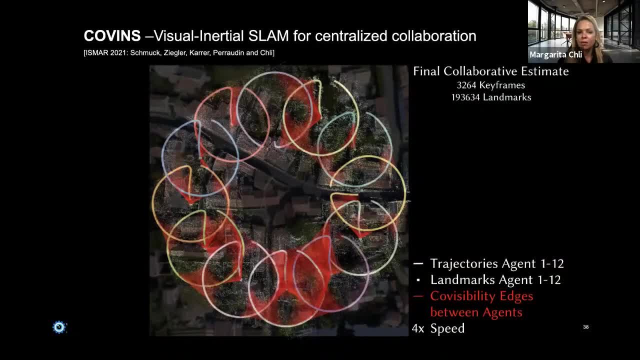 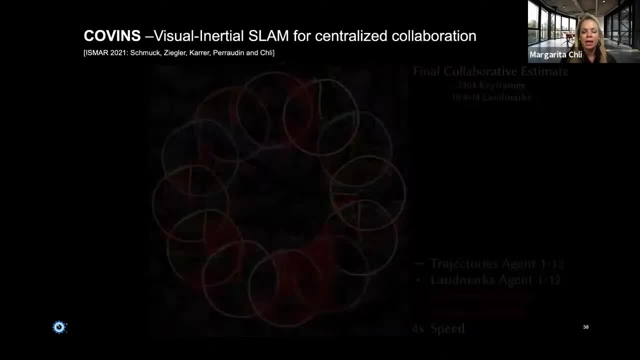 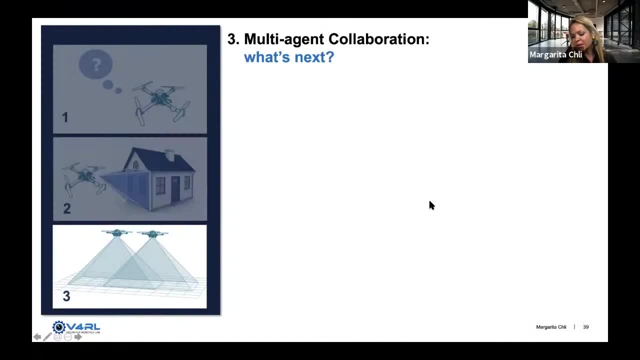 and, of course, modern twitches. So this system now works with Orb SLAM 3.. So the latest high performing SLAM systems And you can try to do collaboration with your own work Right. So multi-agent collaboration, what's next? 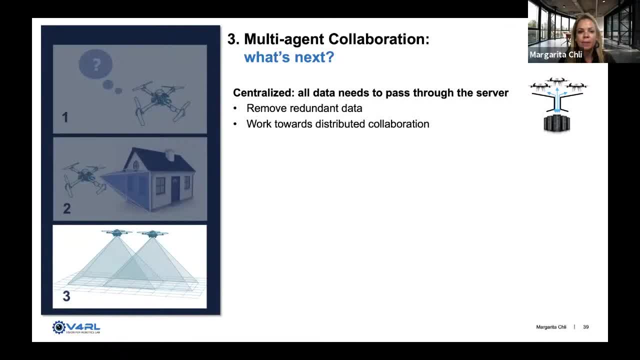 Well, of course, so far I've talked a lot about centralized architecture. So, yes, we do some work in removing redundant data, But we also work a lot on distributed collaboration, which I think is key to progressing this field further. 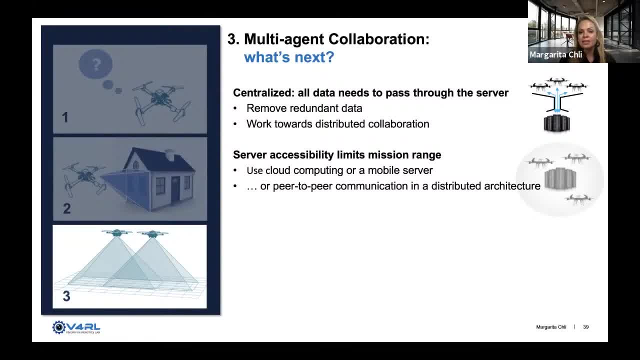 Yes, we do have the limitation of accessibility of our Wi-Fi range, But if I find a good way, of course, if I find a good way of communicating really from one drone to the other, peer-to-peer communication, then we can actually put our distributed architecture. 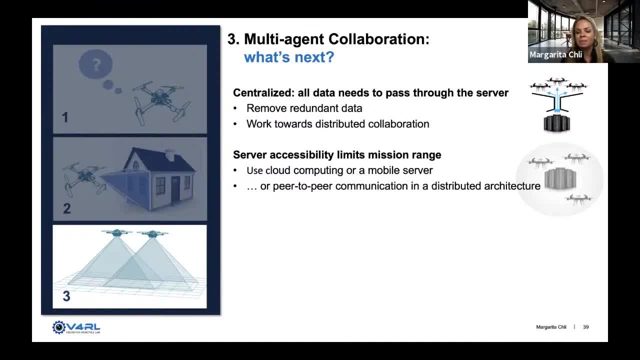 into action, Which again, I think it's the way forward for scalability of collaborative SLAM solutions, And we're also looking at enabling stronger collaboration. And here you can, yeah, looking at this scene, I'm sure you know what I'm talking about. 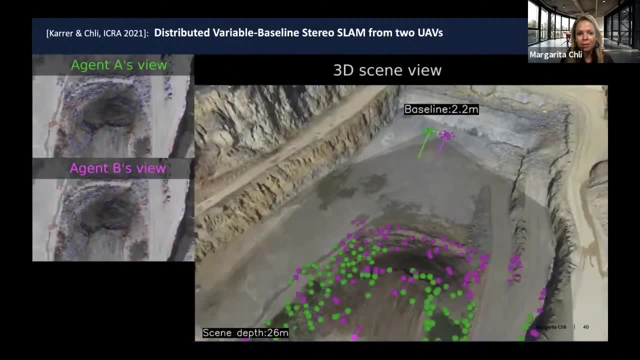 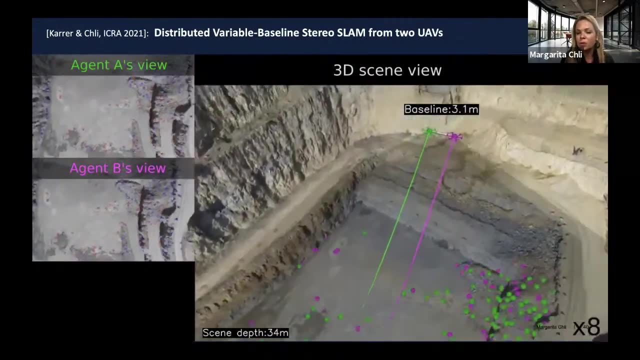 But I'm going to talk about it in this recent video that Marco came up with. He presented it at ICRA. So here we're having a simulation of two drones. They're forming a virtual variable baseline stereo using one camera onboard each drone. 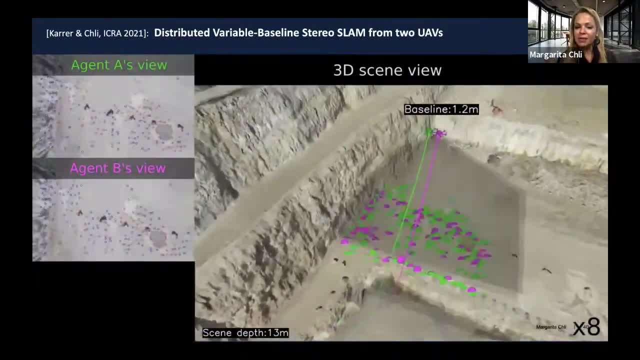 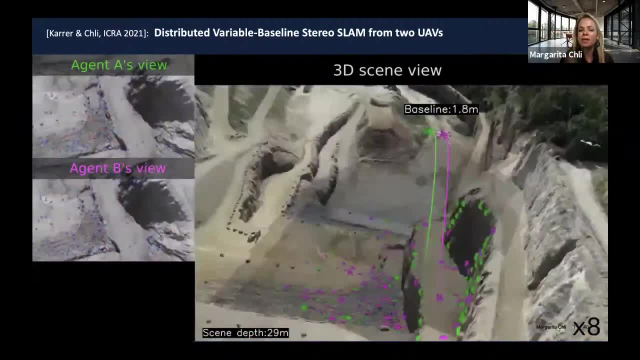 Bear in mind that the drones here are not colliding. We're just inflating their size for visualization purposes. But the key thing here is that these drones are able to control their baseline according to the depth of the scene that they're looking at. 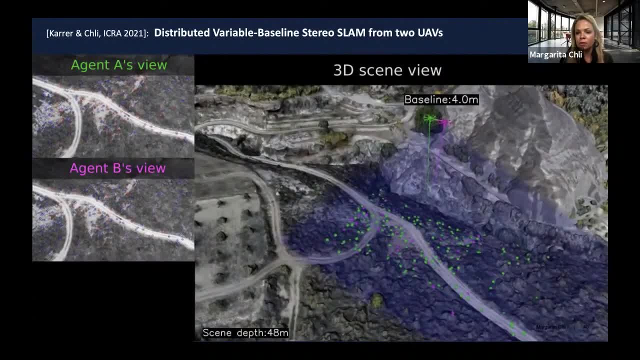 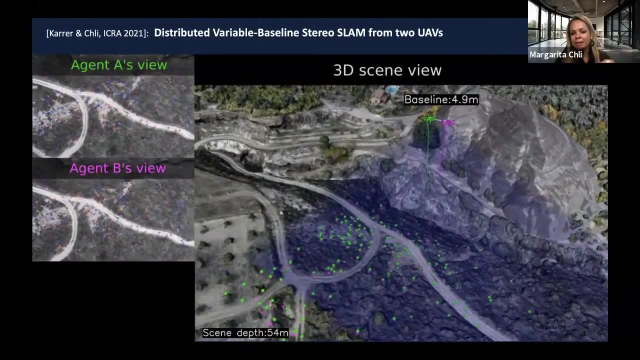 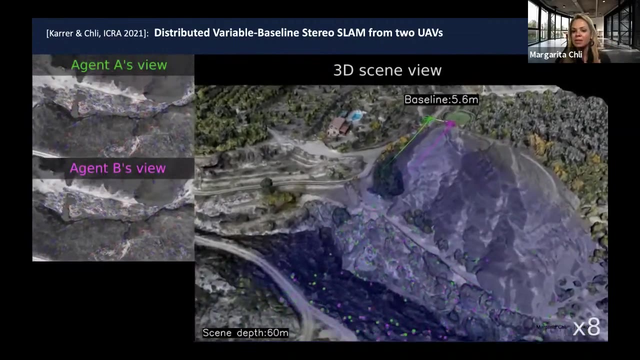 Right. So in order to so, look at this example here, for example, where they're going to navigate on top of this mountain, So they will need to change their baseline when they're going closer and closer to the scene base, So the depth is becoming smaller. 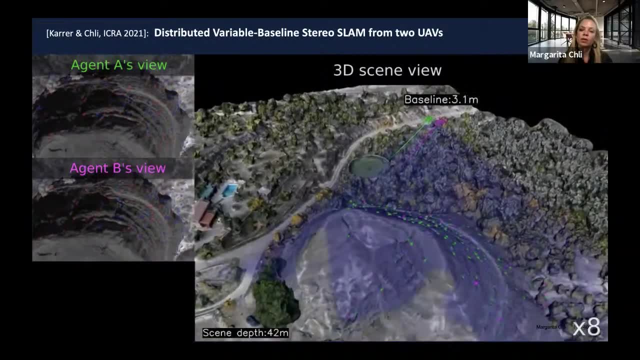 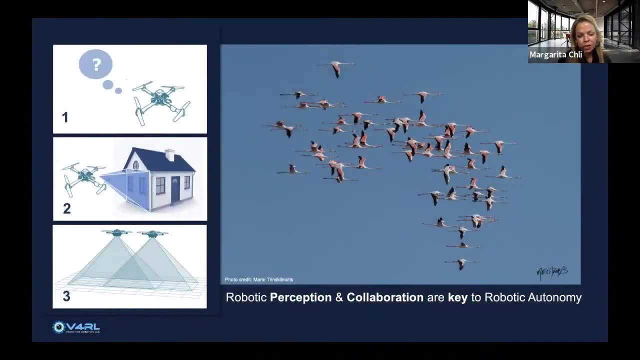 Right? So you need a different baseline, as with respect to when you're experiencing the scene that is further away from you, Right? So with these three challenges, we are aiming to teach robots to see and collaborate, because we believe that these are key to pushing robotic perception. and what? 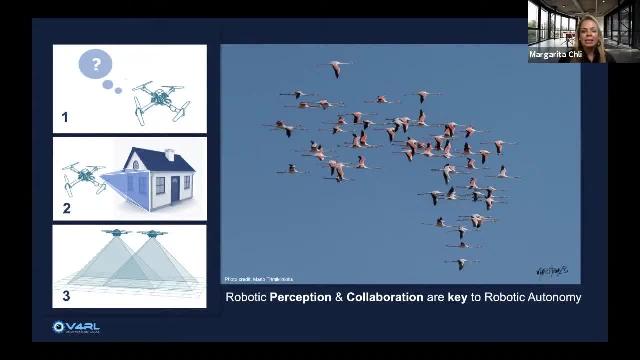 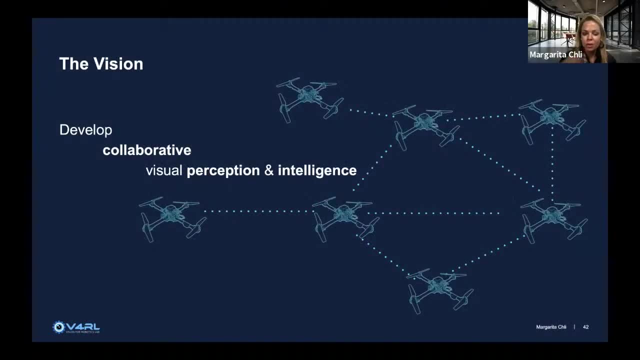 robotic autonomy can do today- And indeed I did spend a lot of my talk to show you videos on drones, because we at the Vision for Robotics Lab we're aiming to develop their visual perception and intelligence that will enable them to collaboratively perform as a team. 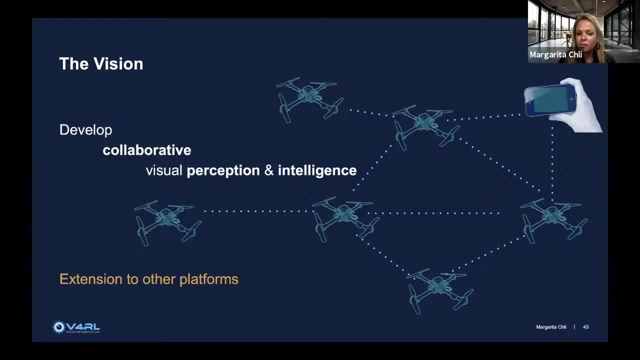 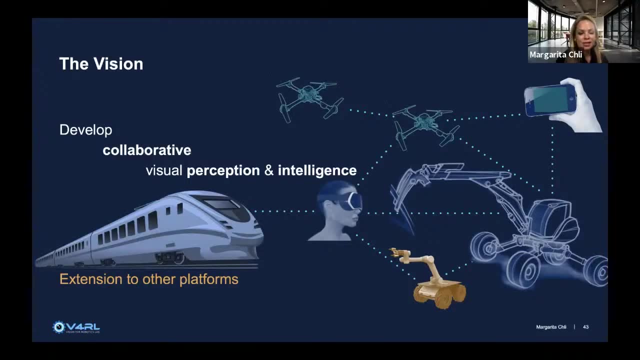 But the extension to other platforms is well. straightforward might not be the right adjective here, but let's say that it is possible to extend to other platforms using the same principles, And indeed here are some examples of projects that we've been running to automate. 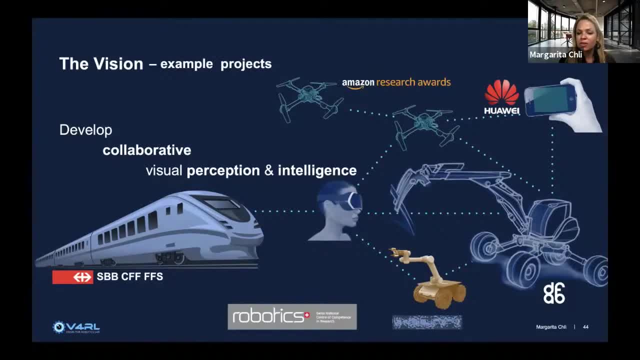 train navigation. So robotics for search and rescue. So we have a team of different types of robots That are collaborating with each other to map a disaster area or work with Huawei to have a gaming application for multiple phones, multiple users that operate in the same area and visualizing the same. 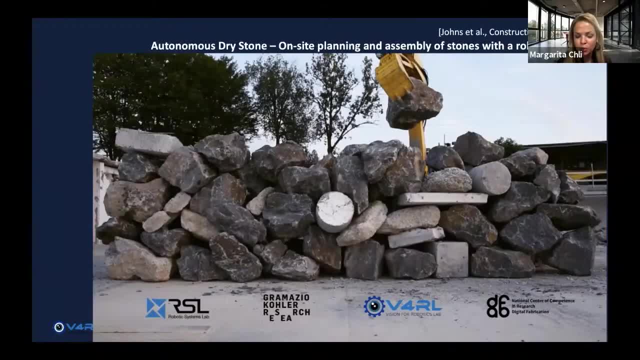 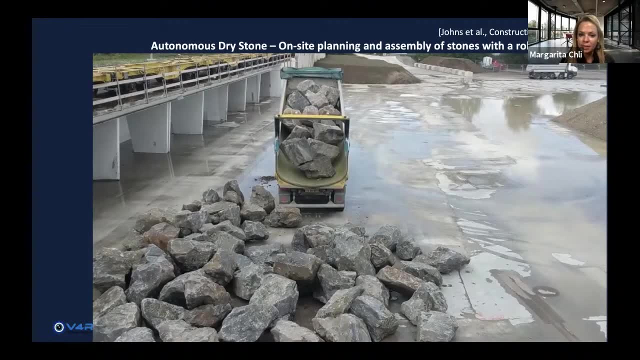 virtual area And this is the last video I want to show you because I think it's quite impressive. So this is a collaboration, not only from my lab, a collaboration different labs here at DTH: architects, roboticists, mechanical engineers. 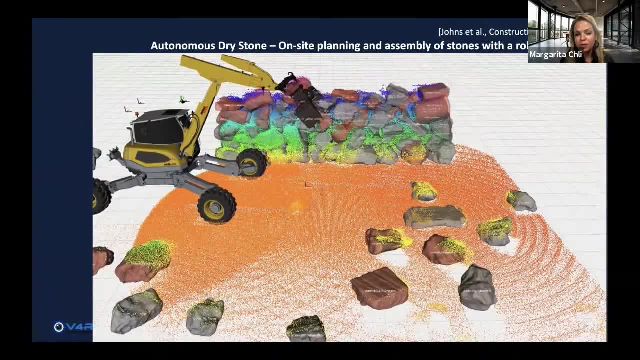 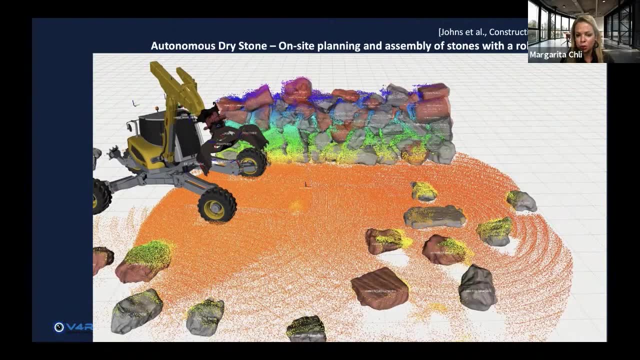 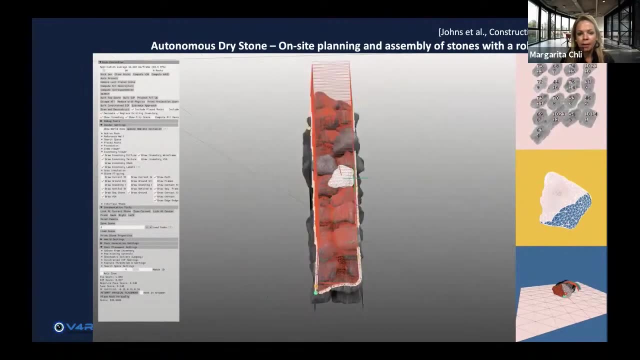 So we are building using an autonomous excavator that you see. here We are building a freestanding wall out of locally sourced stones, And so here we are using onward perception on the on the excavator itself. If you look closely, there's no driver in there. 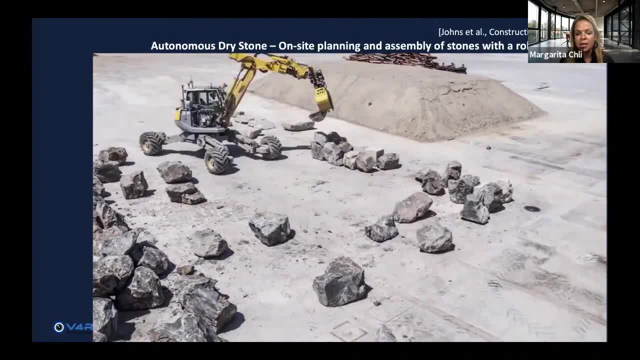 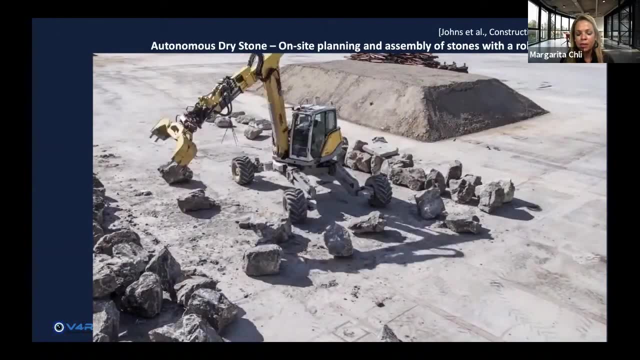 So this is a video that is captured over the course of a few days And you can see in a little bit how we're going to come up with this freestanding wall. Let me tell you that these stones and rubble, they weigh about one ton each. 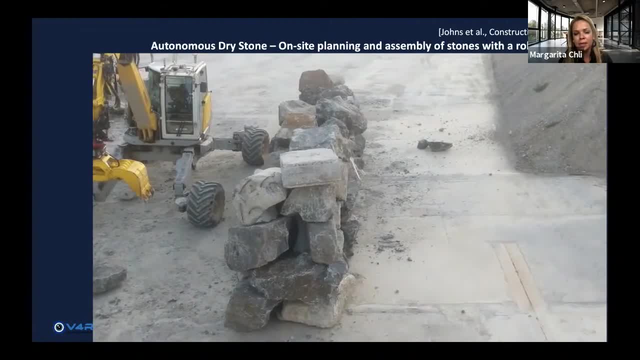 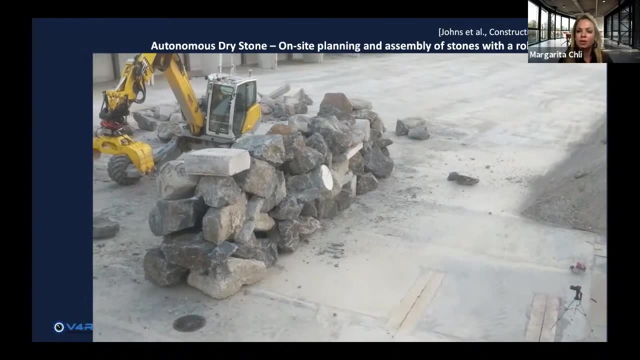 Here you go. It's not the most beautiful wall you have seen, but I hope you agree That is pretty impressive to see really how far robotic perception can go and what it is That it can do. So I think this is just the beginning. 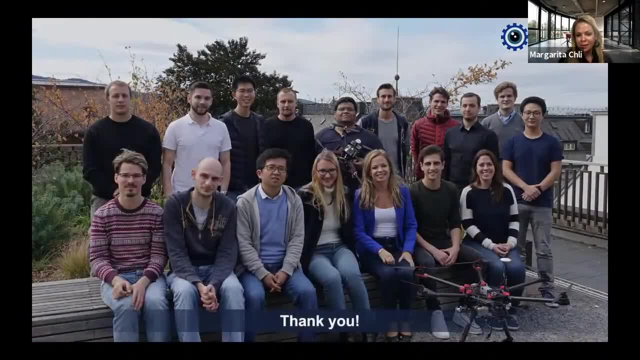 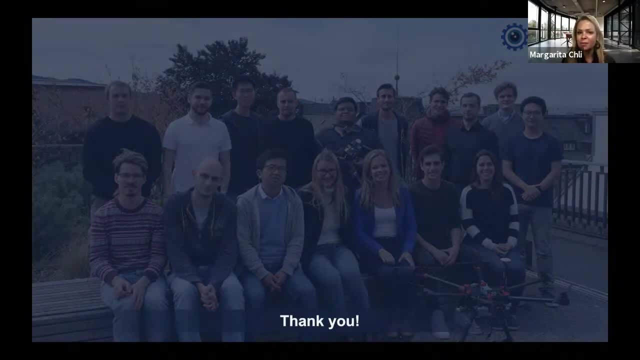 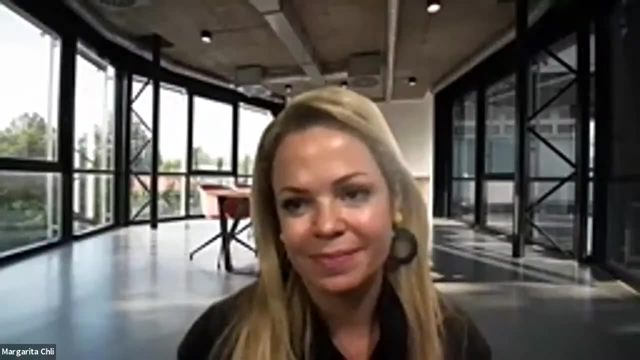 And with this I would like to thank my team. This is an old photograph already, but of course this is a team effort and thank you very much for your attention. I'm looking forward to your questions. Thank you so much, Margarita. 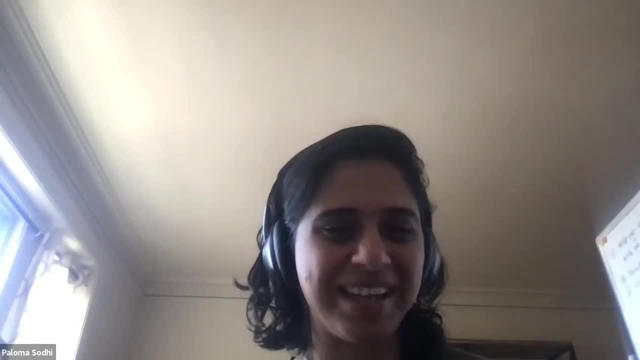 for the wonderful talk. I thought it touched on so many interesting and important problems in robotic perception and SLAM and it's very general And the work you're doing is very exciting. I also loved all the videos and we have a couple of questions. 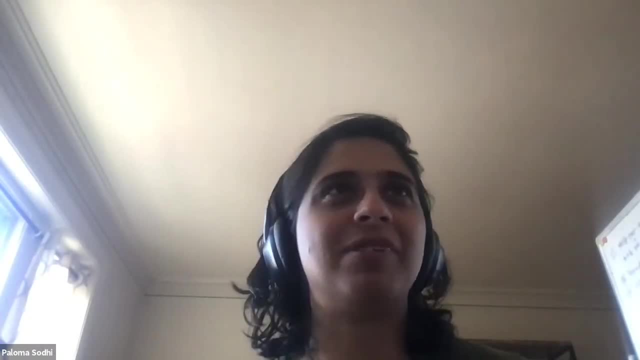 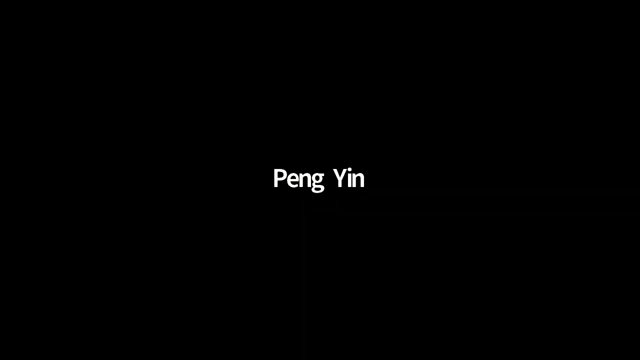 So maybe there's someone who's raised their hand, So maybe we'll take that first. Yes, So, Peng, do you want to say your question? Yeah, Okay, Can you hear me? Yeah, great, It's very impressive, Yeah. 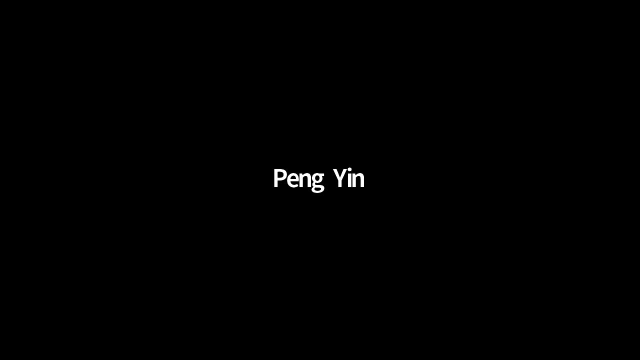 I'm going through all the videos and all the products. It's very impressive, Yeah. So I just want to wonder what? how are you doing the multi-agent, corporate mapping, corporate SLAM? I mean, if it's the same path? 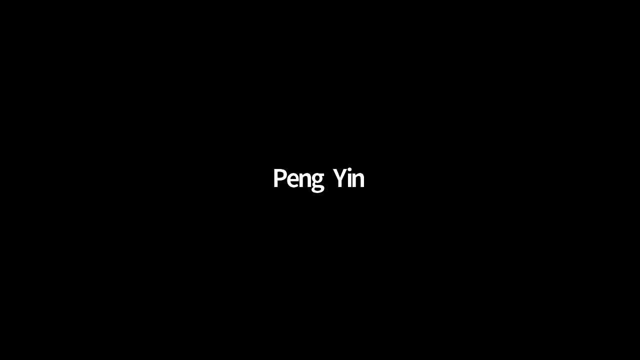 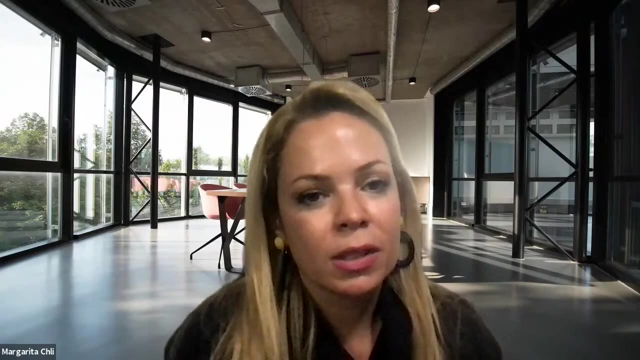 you're going to several times several trajectories. So in that case, how can you doing the data association between two trajectories? Good question. There are many ways one can do that, but the way that we do it is we take the modules of a traditional SLAM. 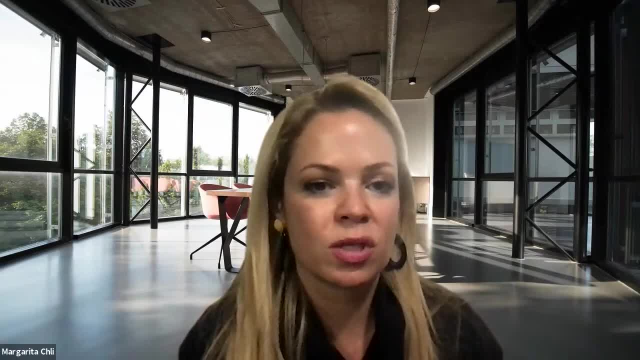 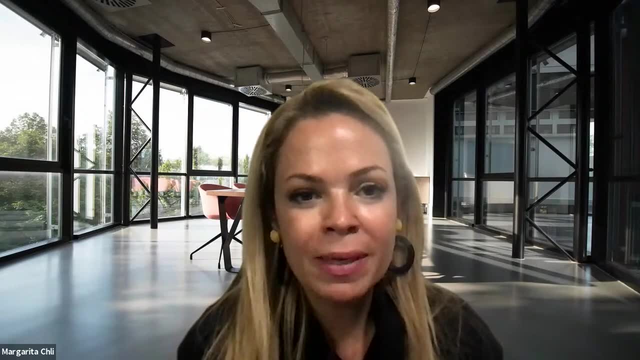 system. How would you do data association? How would you do place recognition right For one robot? And then it's about streamlining the right inputs to that module And it comes up with a place recognition amongst the key frames that you. 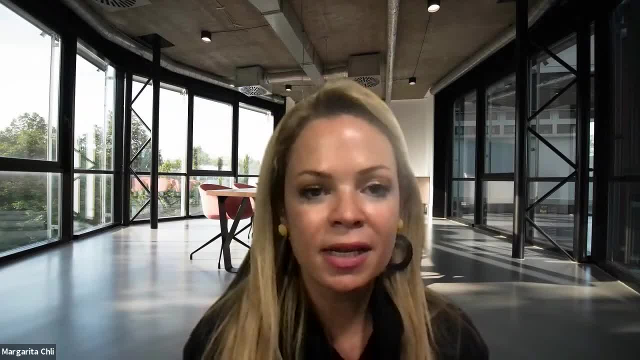 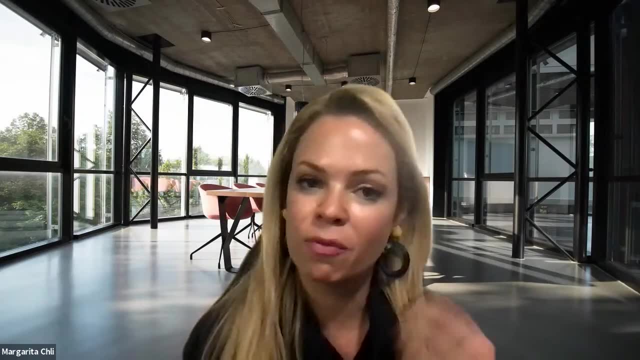 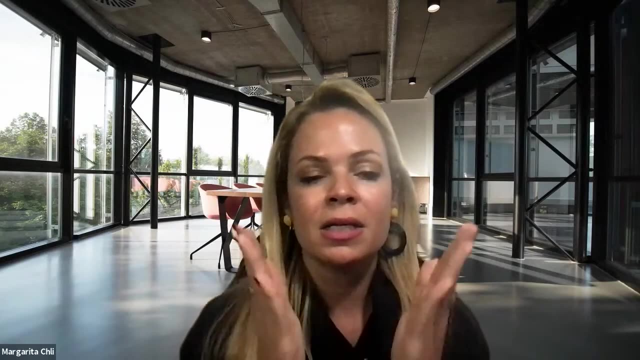 you give it right And it's doing data association amongst the key frames that you give it. So the frame to frame mapping is coming from the individual agents. So it's done already. But then when these key frames are streamed, the line streamlined down to. 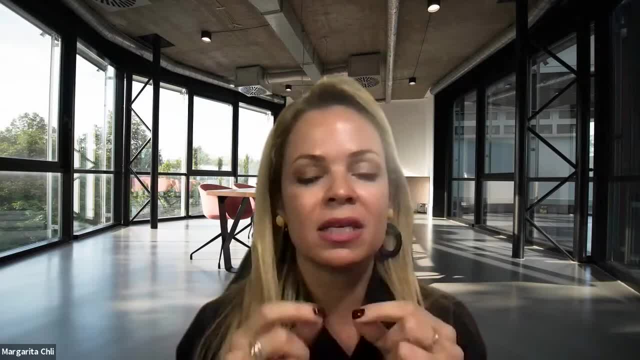 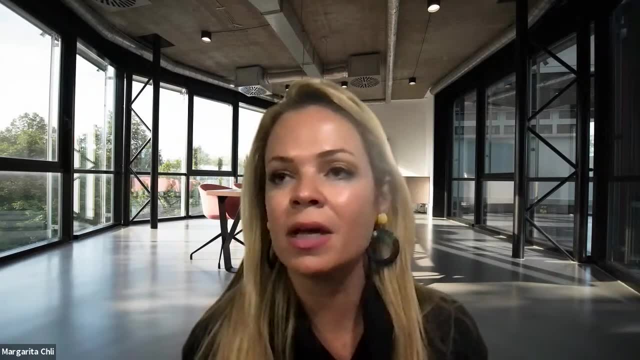 to the server, then that server is taking these key frames and it's trying to match one by one with respect to the database of images that it has. So, in the same way that we're doing, basically, we're doing it for a single robot. 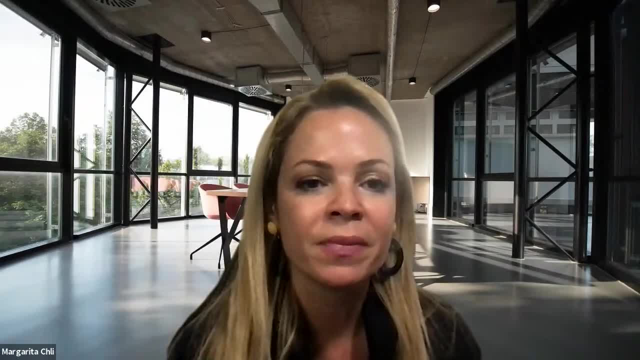 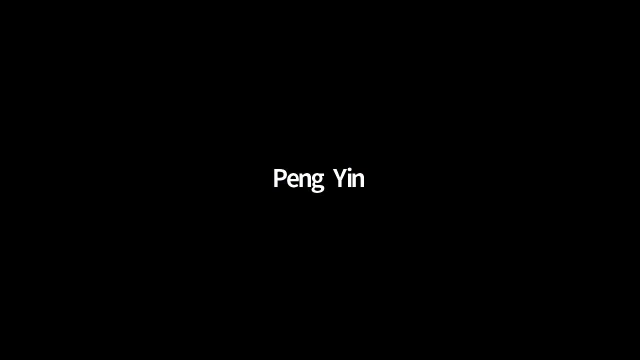 then you can do it for multiple robots in this scheme of collaborating in this centralized, in this architecture. Okay, Got it. So I was just once you wonder. so it is for the same area. maybe you'll wait more, you'll be. 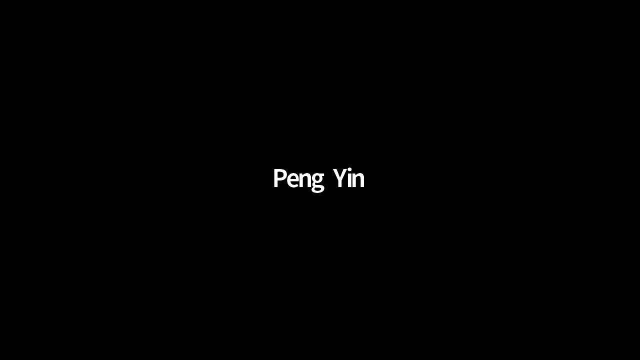 maybe your robot will be visiting here for multiple times. I mean so mostly we. you didn't come here for two times. It's okay. We're doing the data association for two drives, It doesn't matter, But for the if there's a 10 track. 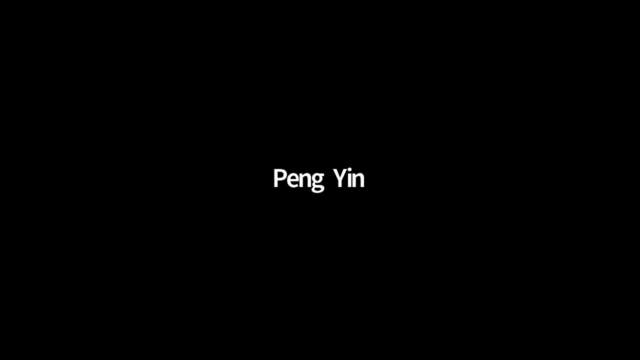 10 robots going here at a different time, maybe the lighting is changing, Maybe the viewpoint is changing. So, in that case, if the data association some can, it's up to us to to, to allow, to allow it to be. 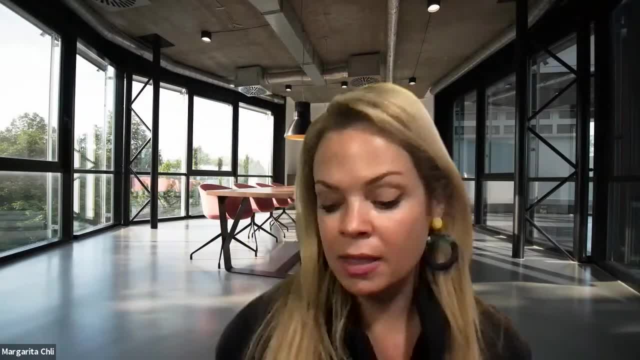 to allow it to be more accurate. So which we were making a photograph. This is. this is spot on, And that's a very nice topic, Basically, for someone to figure out. shall I trust the math that I have already, or? 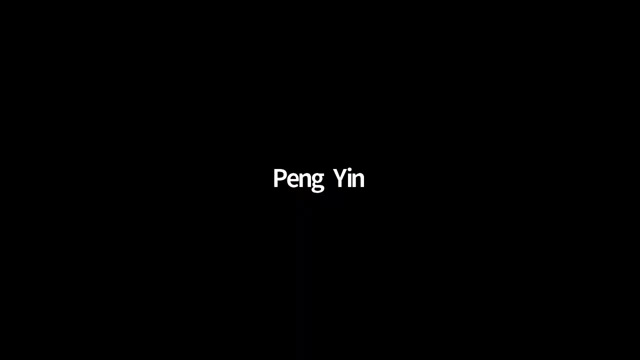 Delete them. So is this building Something that has been demolished and is not there anymore, or it's my current perception of where I think I am distorted. So it's then also goes on about The, the, the, The, the. 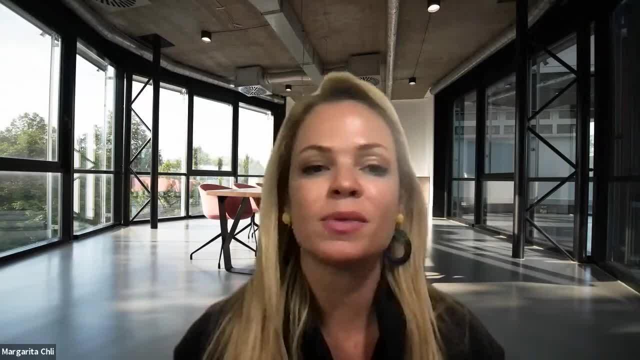 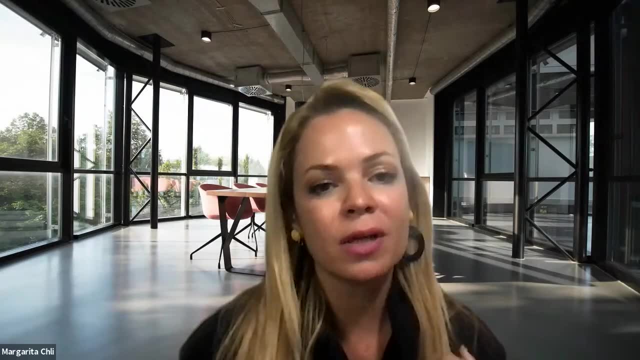 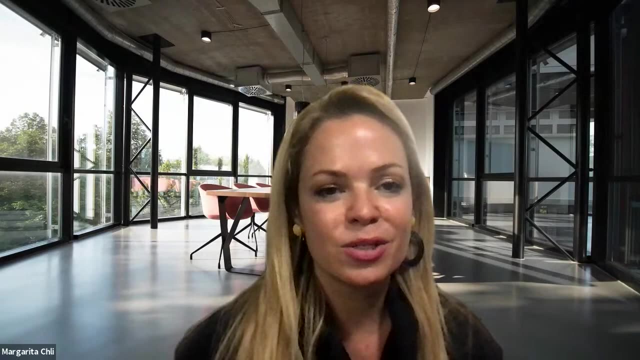 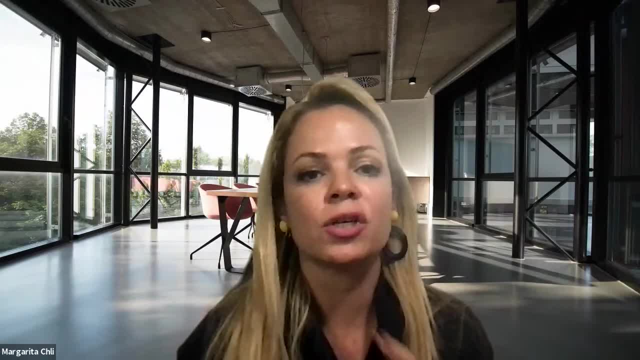 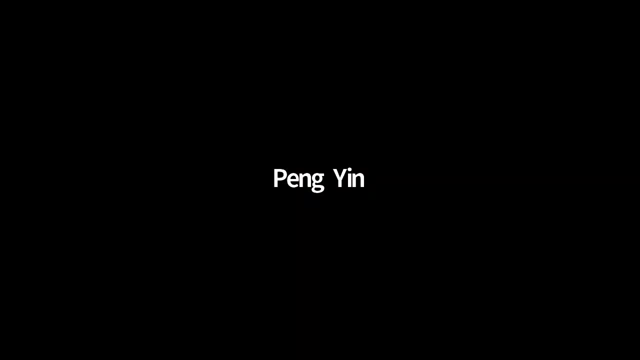 work. that looks up, looks into multi-session, um place recognition. it's a very interesting actually, so, actually, uh, so i'm max, i'm from basis lab, protestantist, so actually we are also doing the same thing. yeah, fantastic, yeah, later we can talk in more detail, absolutely, absolutely. 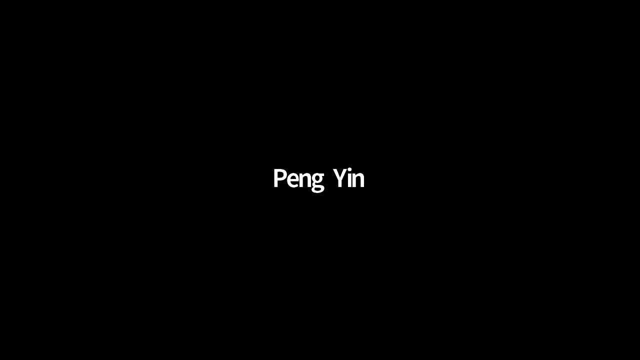 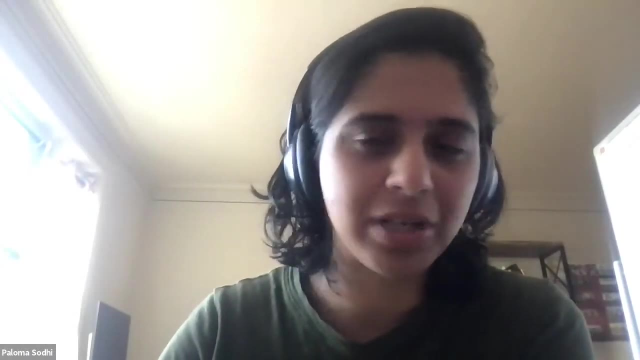 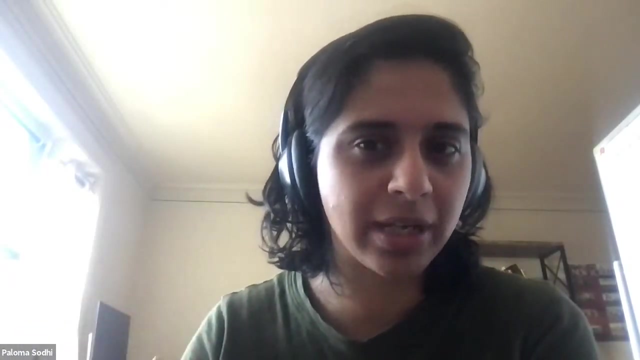 thank you, thank you, thanks, uh, thanks, thanks for the question. um, so then maybe now, since we're talking about place recognition, uh, there's a question. when you were talking about the first part of your work on, like, how these approaches, uh, would be similar to like build room in a day. 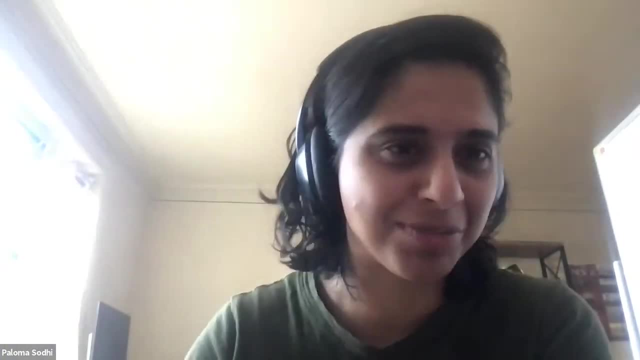 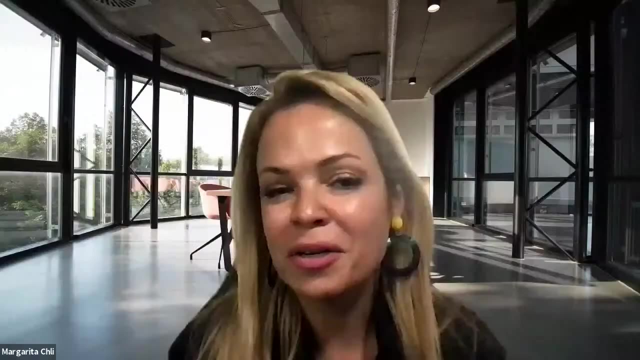 and how different are they? i guess you handle it later when you talk about adjustment, but it would be good to maybe discuss that in context of place recognition, can you? can you repeat the question, because i didn't really catch that. so the question is: is this similar to build room in a day? and i think this. 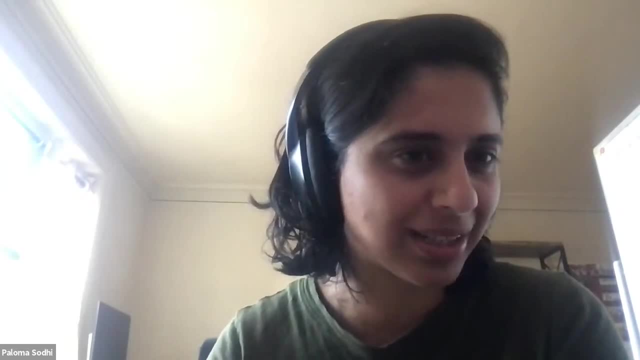 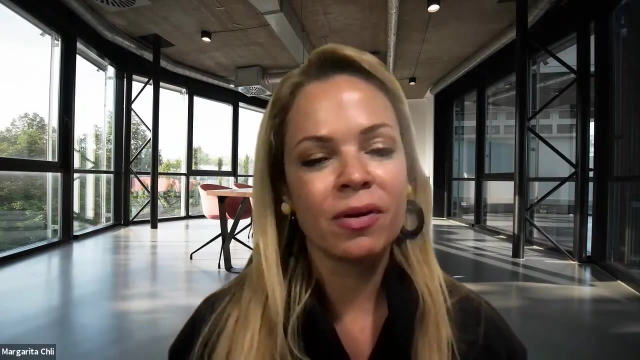 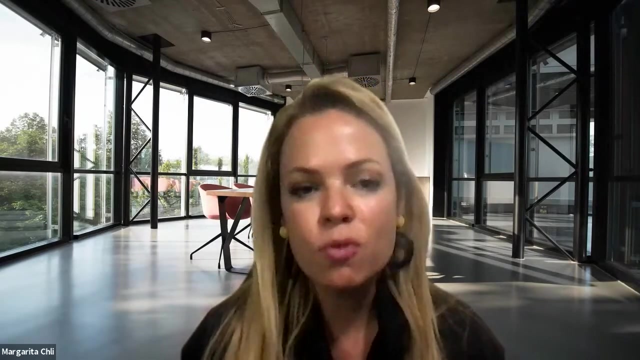 is referring to the first part of your work around place: building room in a day. so um yeah, um no, because i'm not sure what exactly we're referring to. but building room in a day is essentially um capturing a lot of data, right? so this is what we call the full bundle adjustment. 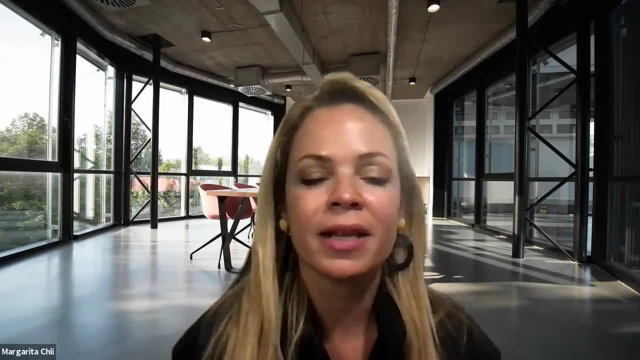 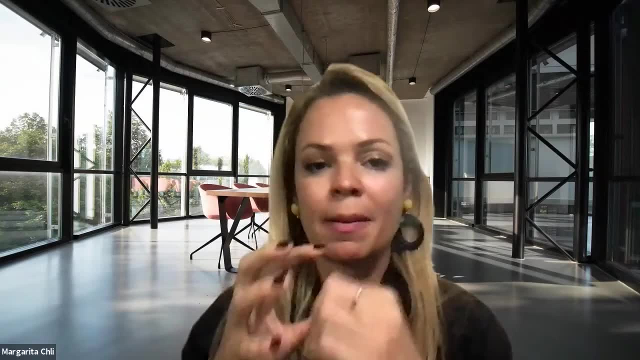 capturing a lot of data. and then we're talking about the first part of your work on place: recognition of data, and then putting them in a cluster and coming up with a map and, um, uh, the poses of where these images were captured from right. so this is the full offline problem. now what we do in the 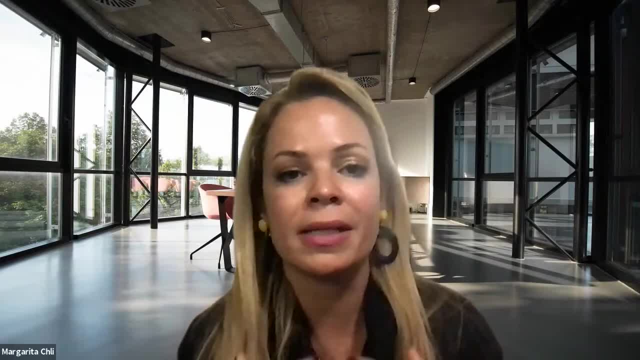 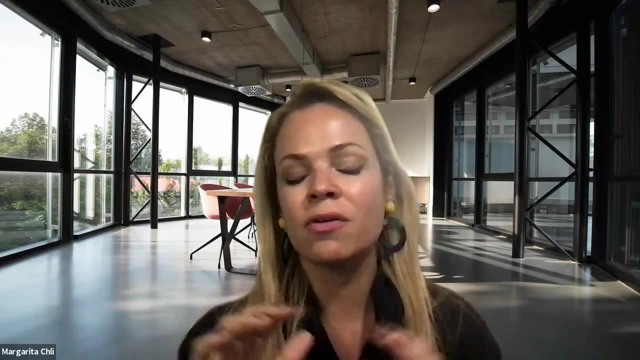 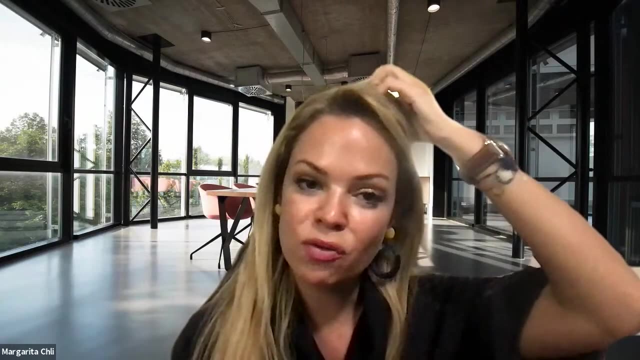 slam approaches that i have shown is mostly incremental right. so you build your map as you're estimating your, your pose. so the the full global bundle adjustment when i talked at the end, when i was talking about the different ways of solving slam, then the full global bundle. 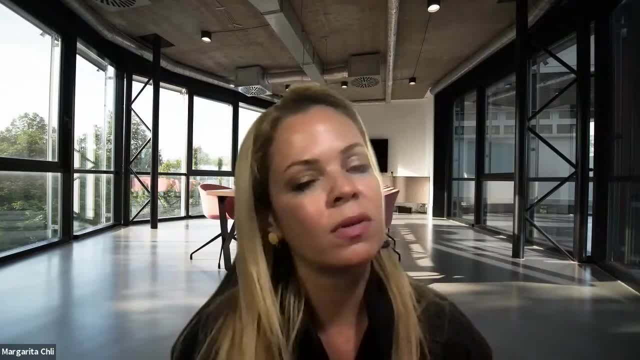 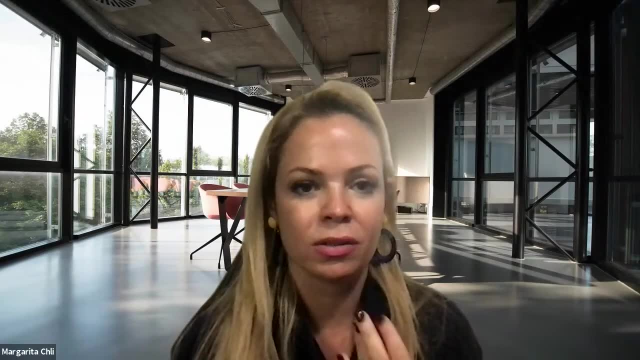 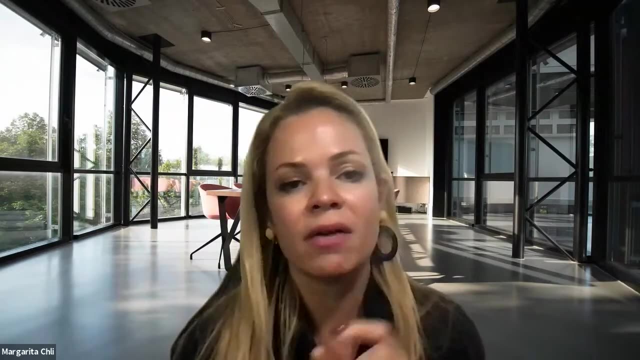 adjustment corresponds to um rome in a day. but overall, the way that we use slam in the videos that i've shown is an incremental online fashion, so that can mean also access to fewer data, right, because sometimes we do select to have a more limited horizon, time horizon than the full global. 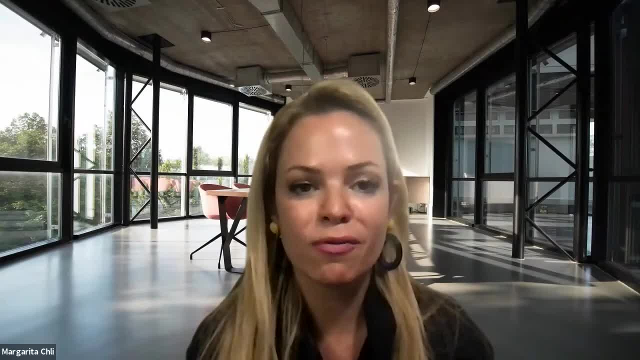 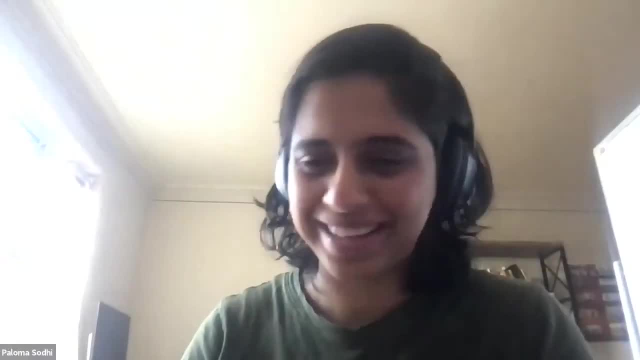 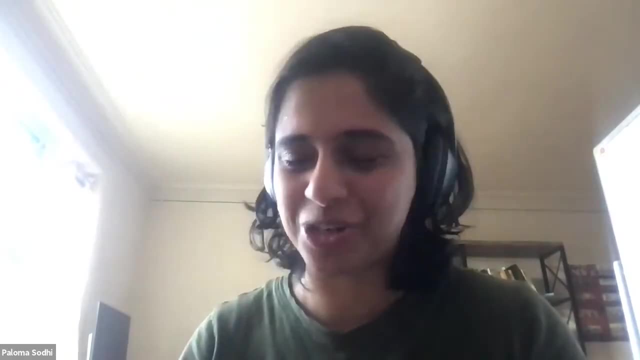 optimization, but in general, it's the way forward if you want to have some autonomy on your robot in real time. uh, thank you. yeah, um, agreed, like there's a real-time constraint, definitely with slam problems, to apply there. uh, i, i had a question when you were talking about the place recognition, some. 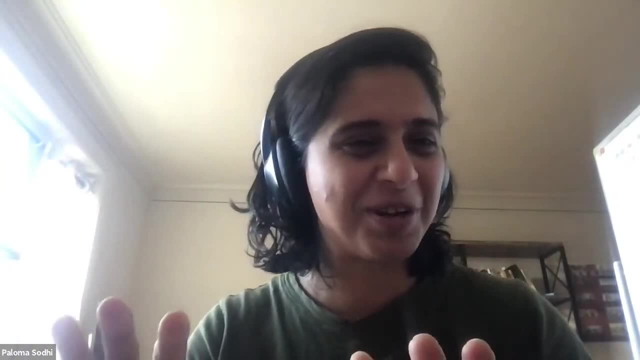 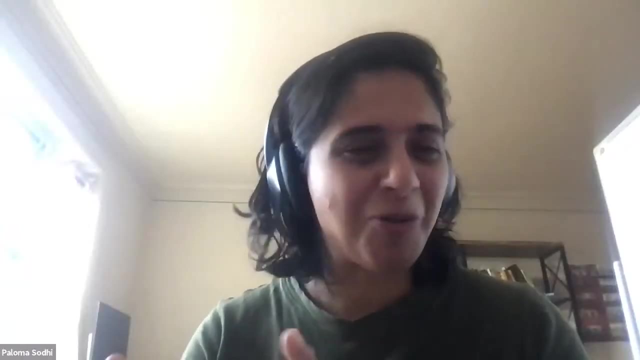 of the images that you showed, it seemed like you. it was even hard for a human to match those two. absolutely, absolutely, i agree. yes. so in that context, what do you think like? how far can you push, like these place trickings in a way that you're not going to be able to do in real time? 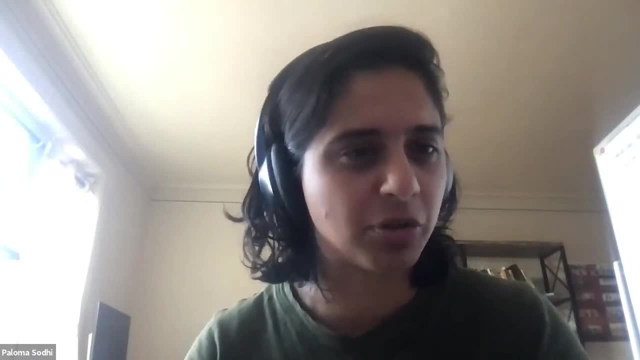 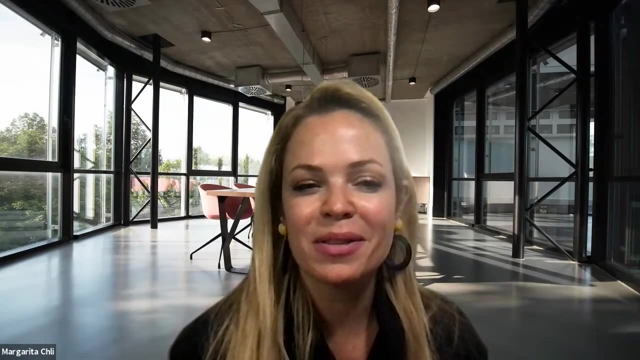 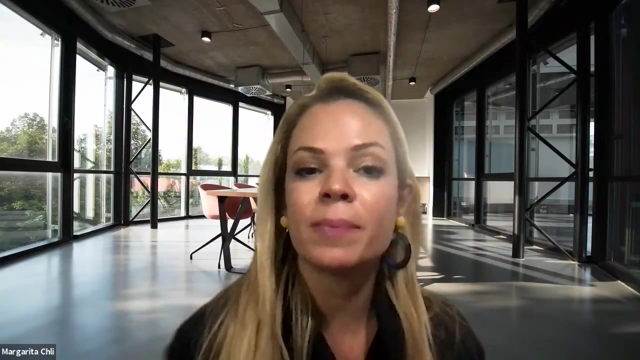 across scene changes and where, like, maybe something else that would be useful to do. yes, i mean, um, a great question, because, uh, i do start by talk, as uh, talking about the motivation that comes from nature, and it does come from nature, right, and but i think place recognition is one example. 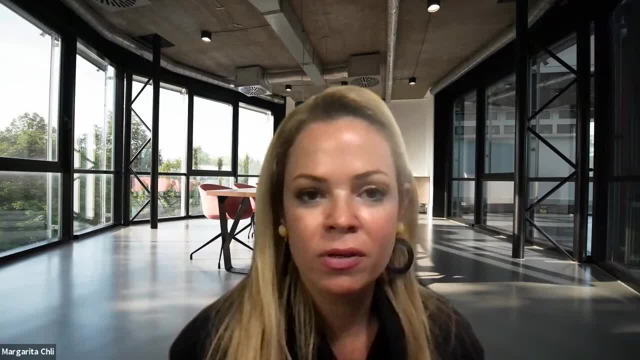 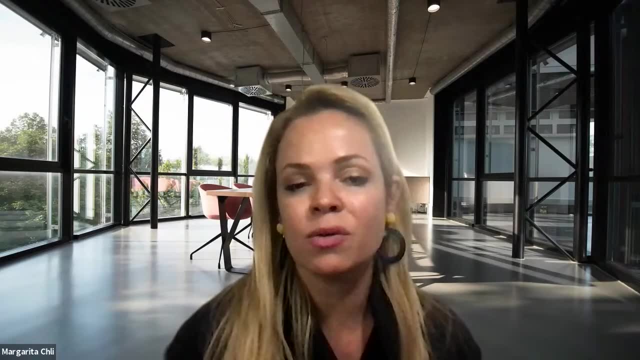 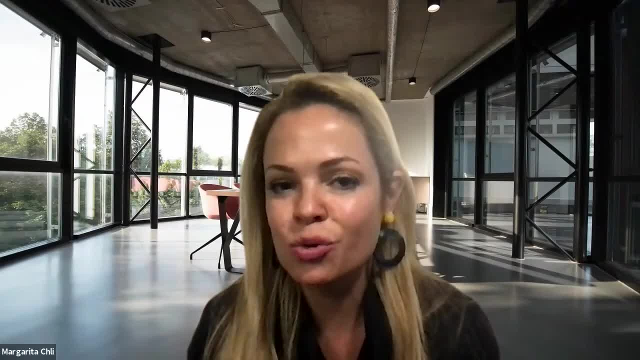 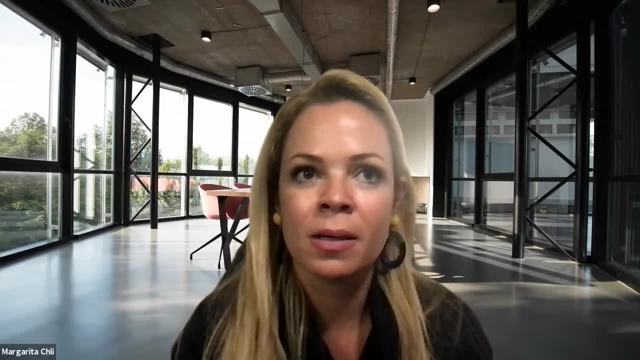 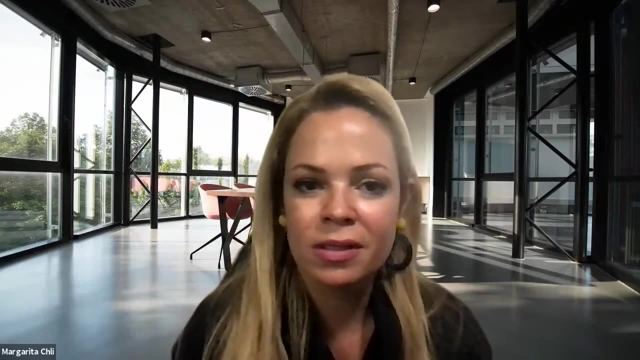 i? i don't know the answer to this, to be honest, and i think it's good to use the motivation of um- you know, the bio inspiration, if you'd like, as um, to kick off where one is going with one's discipline, but then don't stay limited to it. and uh again, deep learning, it is the, the techniques. 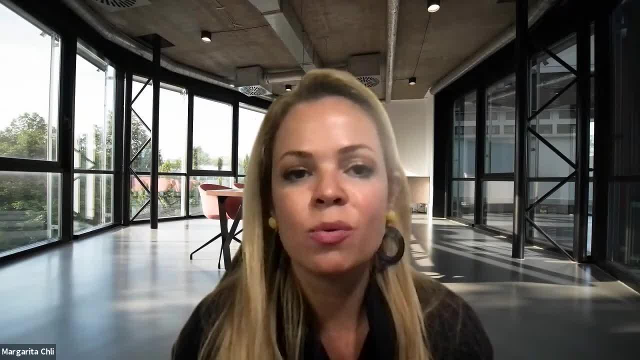 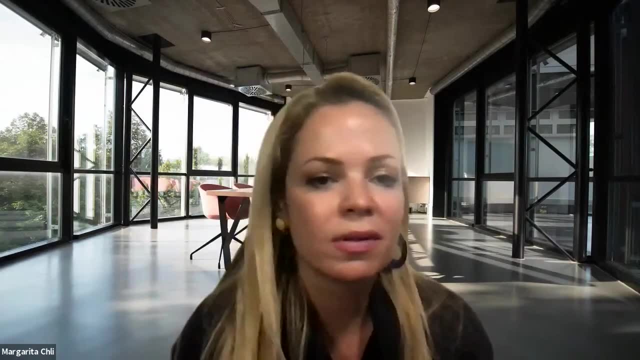 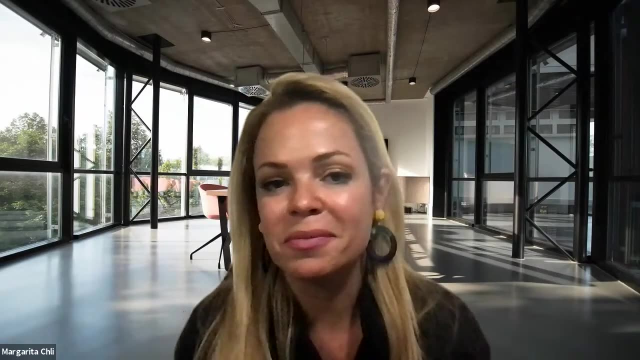 are bio inspired because, um, this is how we learn, right from example and, uh, from looking at different cases. then we start judging about whether this place is the same as this place or uh, so on and so forth. but, um, yeah, i, i don't know where we're going with this. uh, it's exciting to see how far 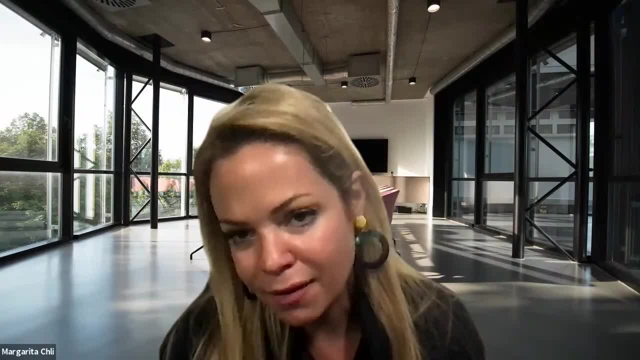 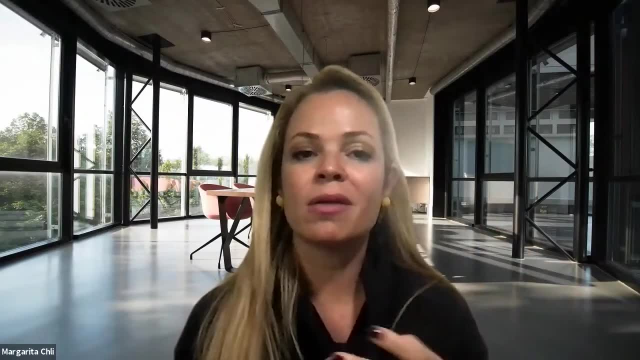 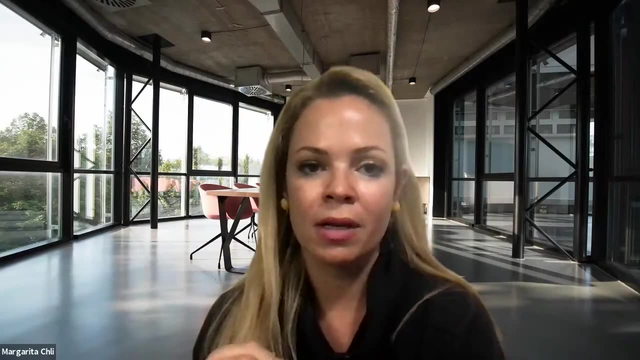 we can push place recognition, but still have to say the bad side of this, as i said during the talk, and i think that, um such methods that work impressively on one particular specialized set of questions, they don't necessarily work as well. well, they don't work well. um, when you tweak even a 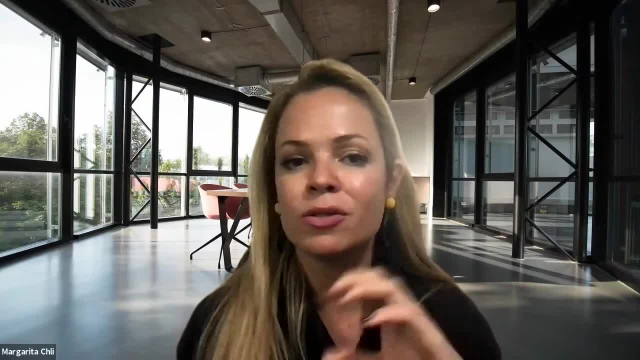 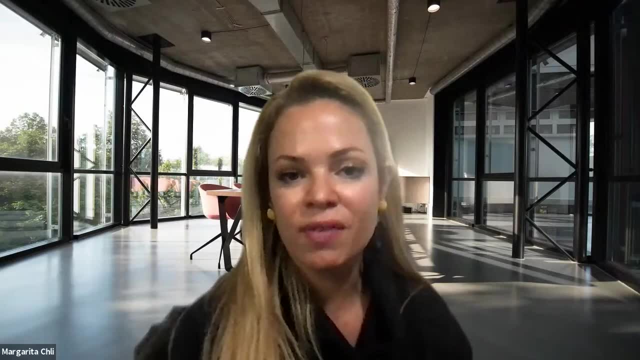 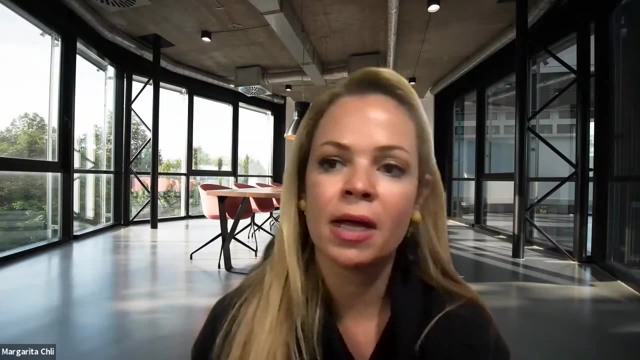 little bit, for example the, the viewpoint right- and i'm not talking about 0 to 45 degrees, i'm talking a small roll- um, rotation and such deep learning techniques would fail. and this is also, i would say, quite a good difference between autonomous driving research and autonomous flying research, because, um, when you're training your 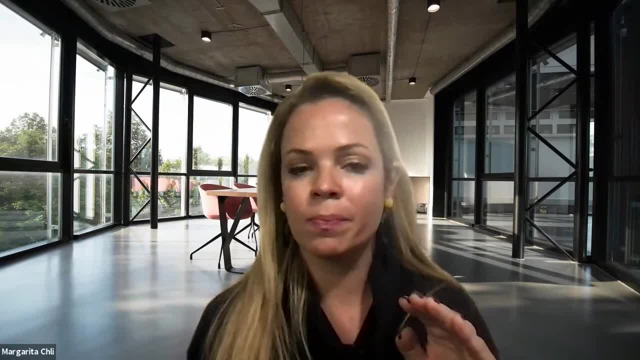 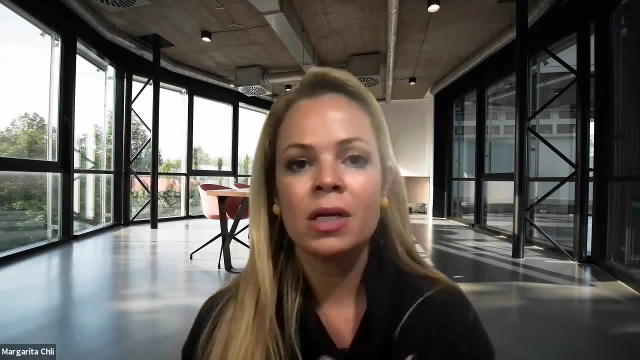 network where and and the, the road is always on the bottom half and the sky is always on the top half, then to to do that for your drone, then of course you're losing some of the accuracy because you don't have that assumption anymore and of course you need different data. 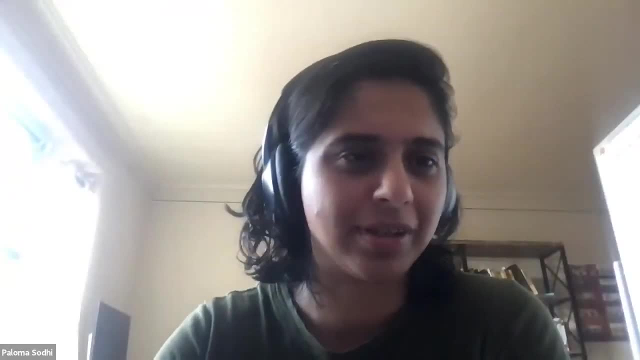 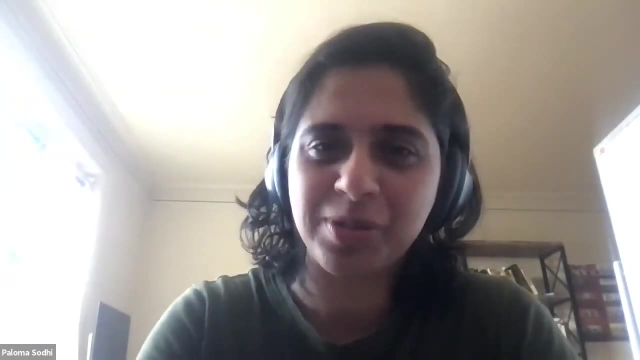 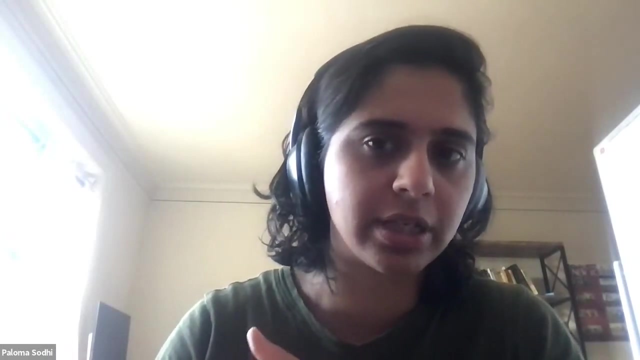 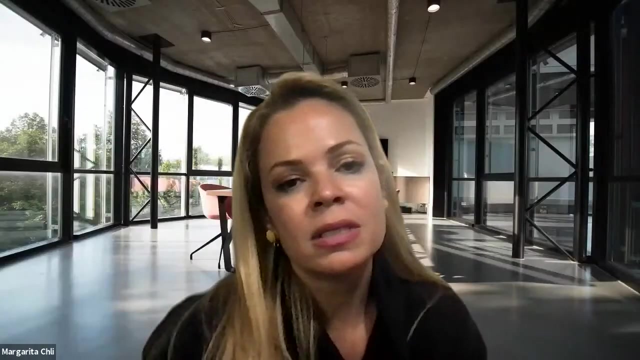 right, so distribution of data is different from there. okay, thank you, uh. and then the next question is the more specific question that we have is: uh, how can you connect two different viewpoints, taken from a different place or with a different orientation, of the same scene, in in slam, for example? um, so the way we do this is, um, we're looking at a scene. 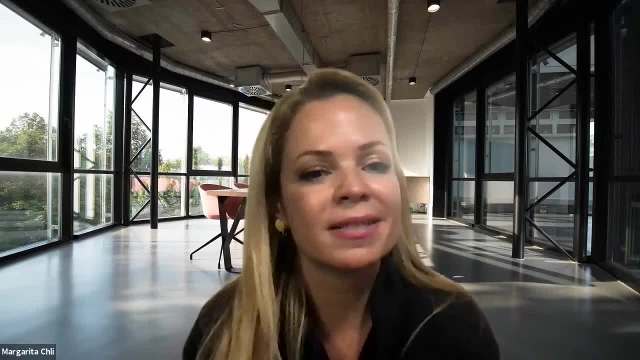 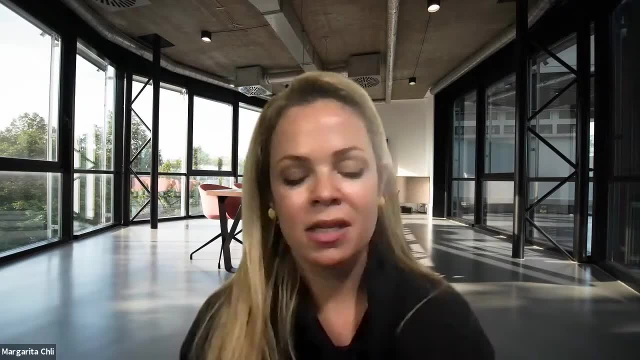 and instead of looking at the full pixels of the scene, we are reducing it into a set of features, right? instead of images. we are reducing it into a set of features, right? instead of images. so you're image patches, And so you detect the image patches of one viewpoint, the image patches of another. 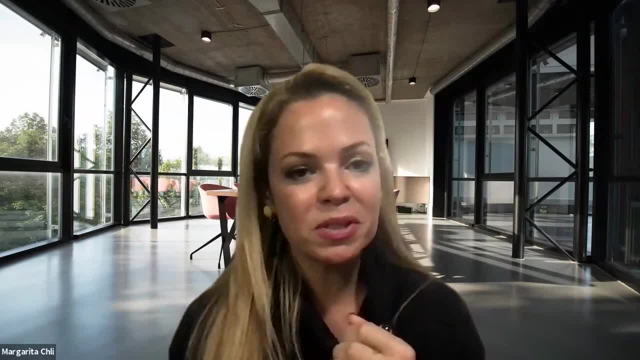 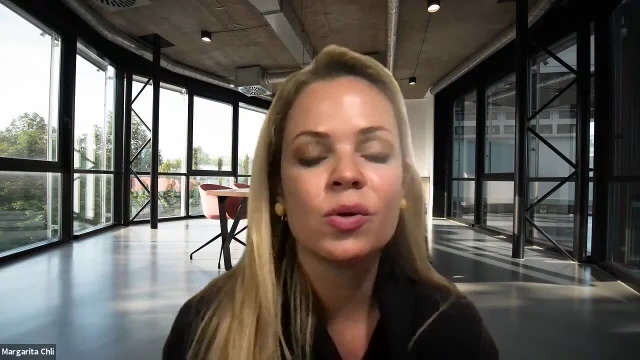 viewpoint, And as long as these two patches correspond to each other visually and also structurally right, so they have the same constellation in 3D, then we accept these to correspond to the same place And you can also imagine this as a registration of one particular. 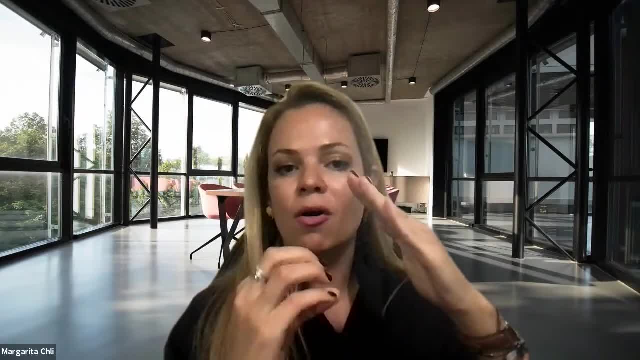 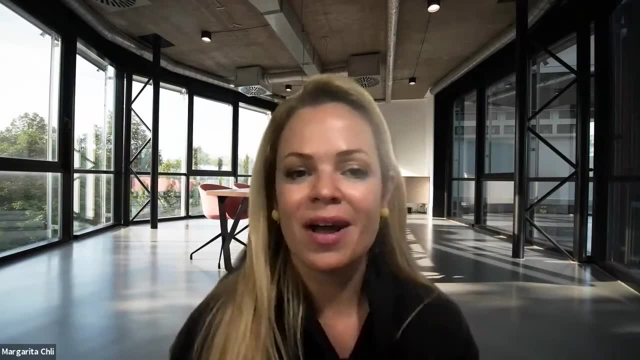 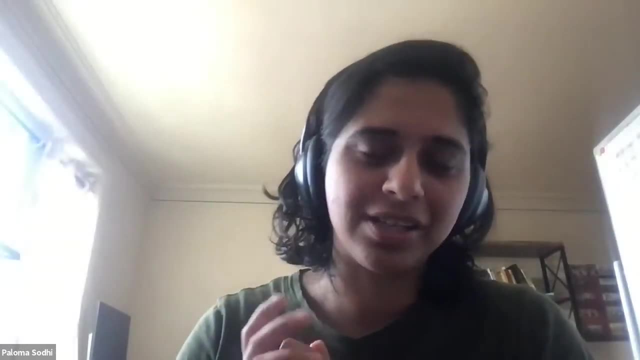 image to a 3D map and another viewpoint of the same area to that map. So that's how you can start visualizing in your brain how SLAM would do it. Thanks, And the next question that we have is for visual SLAM tasks on drones. 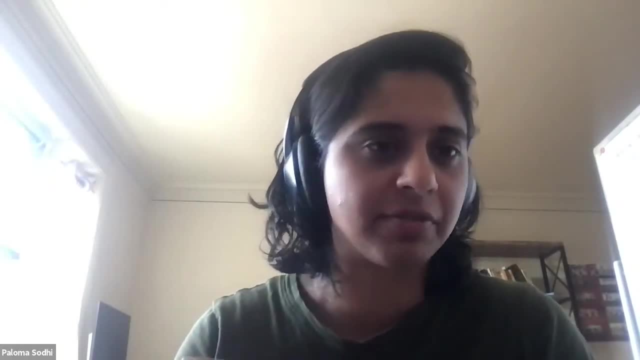 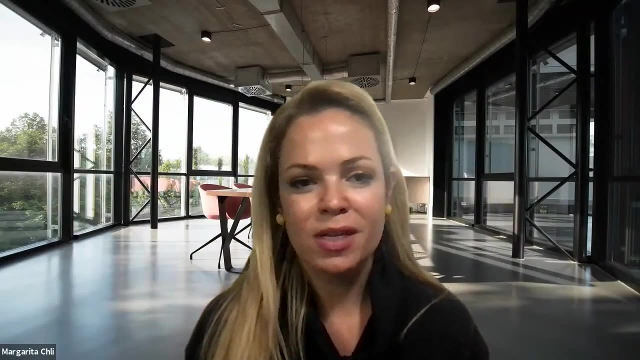 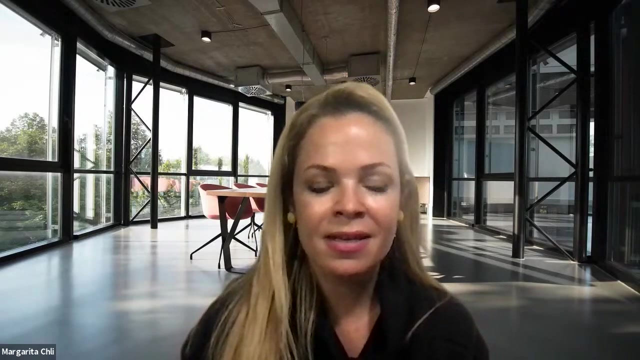 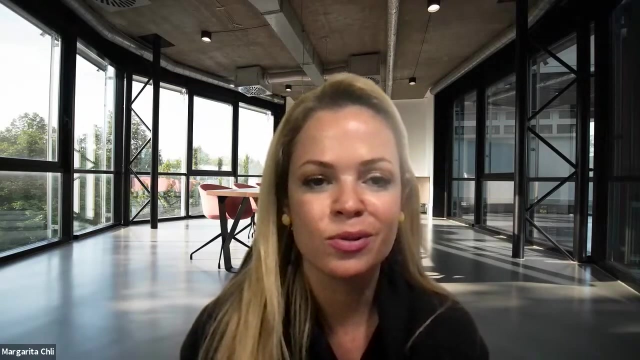 what computing platforms are you using to achieve these impressive results? Another good question. So, of course, to have such impressive videos, we rely on a whole body of work that has been done in other disciplines: In sensing, in boosting the battery lifetime, in having great processors to put on our drones. 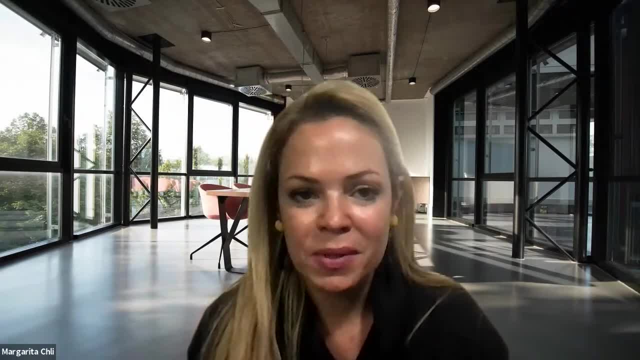 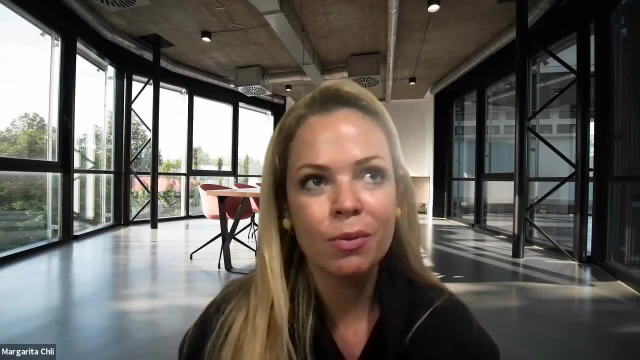 And since, when I started working with drones, our drones were about 25,000 euros. Now you can have a drone for about- well, a fully equipped drone- for about 5,000.. But it really depends on what sensors you put on there. 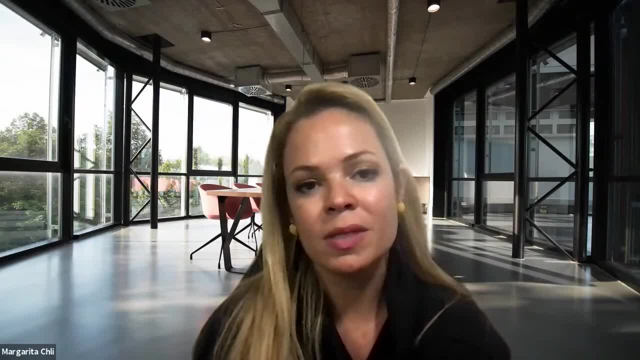 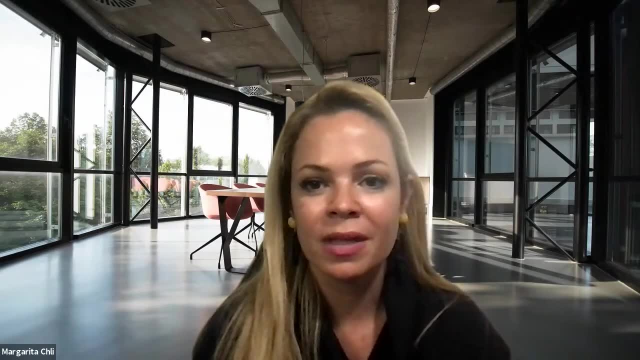 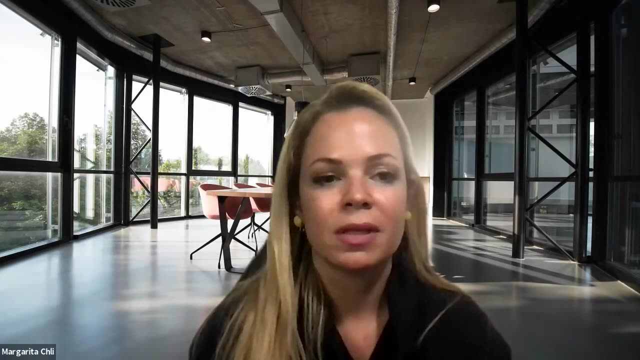 So right now we're using Intel. I think I just had a discussion with my students just before to talk about this. It's 11th generation Intel NUCs, I think. So whatever the industry can provide us, we are taking it. 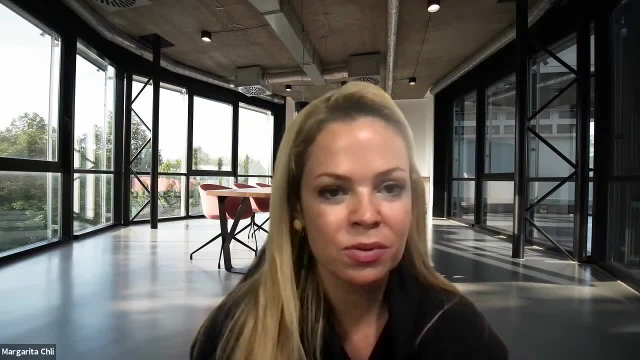 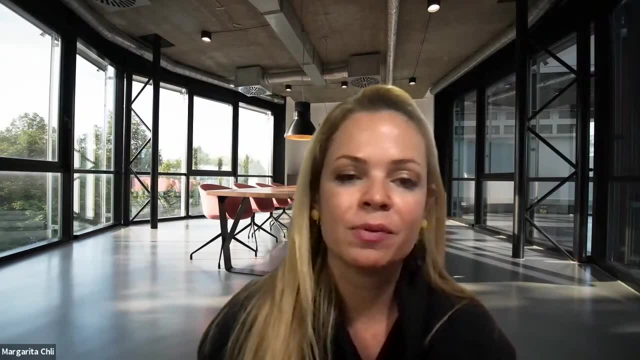 And in some cases we also have GPUs on board, Very small ones, of course. They're not comparable at all to what you have on your laptop or your autonomous computer. So we're using Intel NUCs, I think, And in some cases we also have GPUs on board, Very small ones, of course. They're not comparable at all to what you have on your laptop or your autonomous computer. 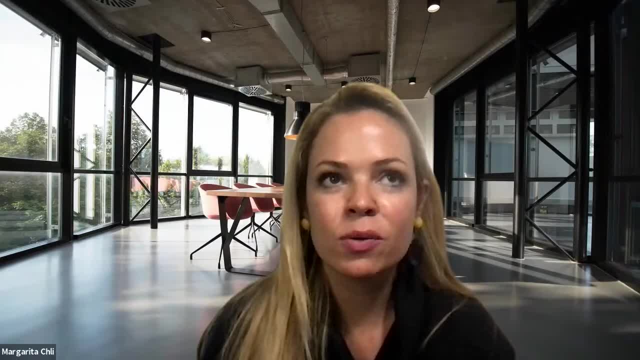 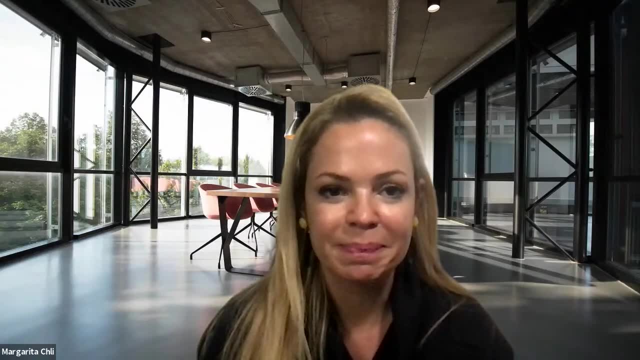 So, whatever the industry can provide us, we are taking it, But this is a very fluid scene, if you'd like, And we are also adapting with respect to that. see, And maybe have another quick one to ask you on your second work. 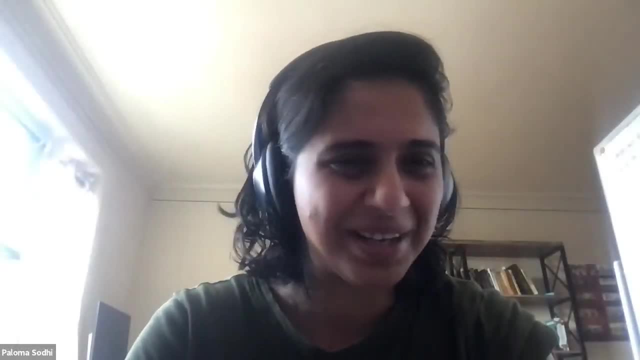 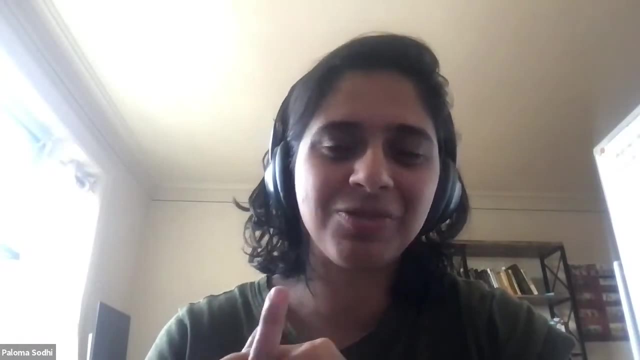 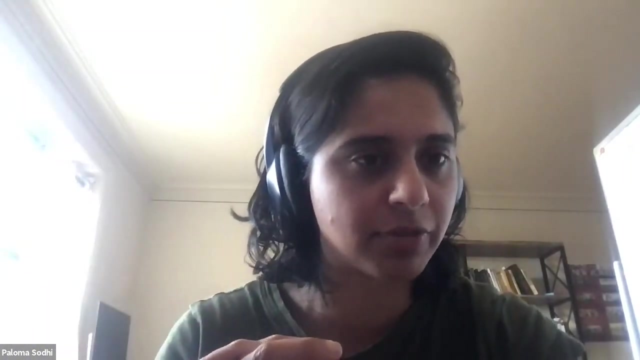 Which was very exciting to me, like using it at a mining application as well. So I guess I want to get your general thoughts on like what. like was that an occupancy grid that was being built, built, and then you were constructing scene reconstructions from there and like what, what? 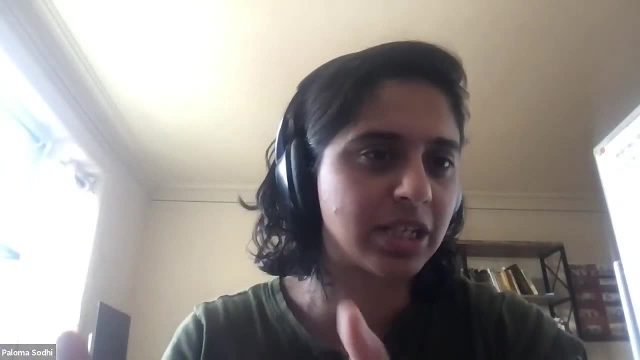 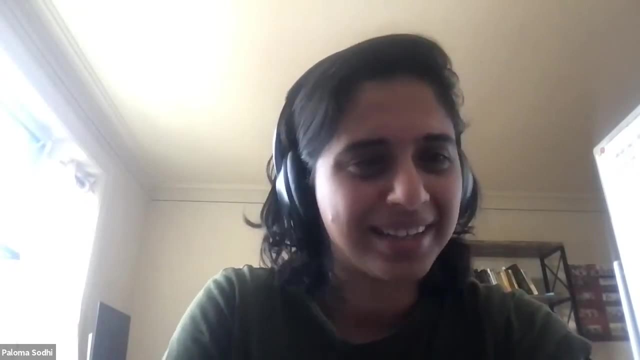 did you like? what would you say are like good? like scene representations that work across like slam, as well as path planning, where you have to have free space and unknown space information, like you mentioned. that's a great phd topic right there, paloma. so what is a good scene? 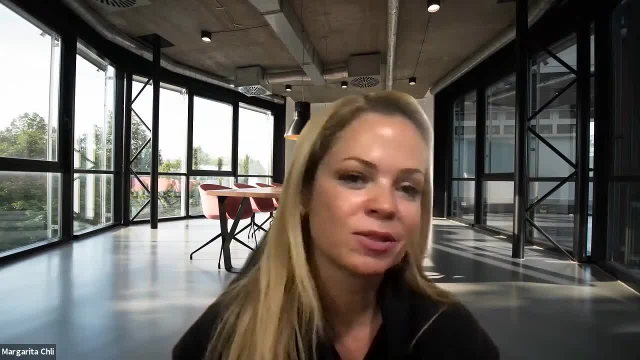 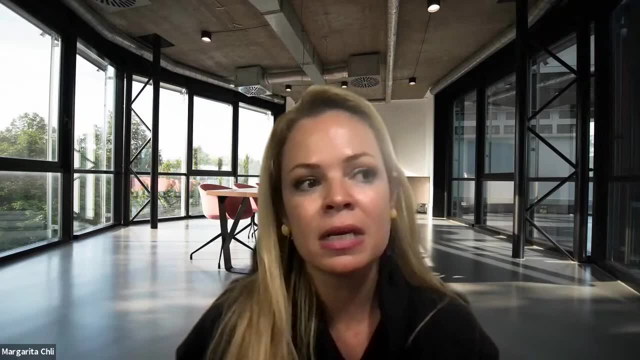 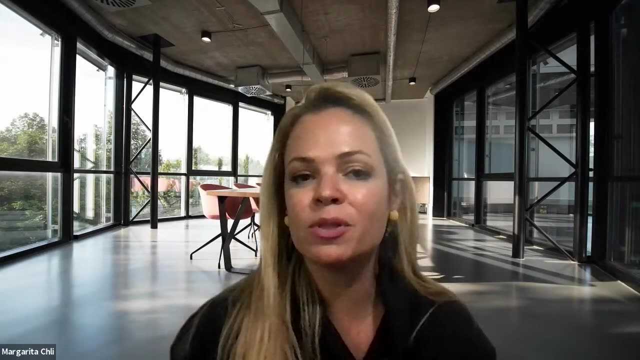 representation for effective path planning. so to me, this is something that i would put someone to work on straight away. um, yes, we are working with existing um structures, that they're out there right um voxel grid to be able to augment this um with whatever information we can encode. that. 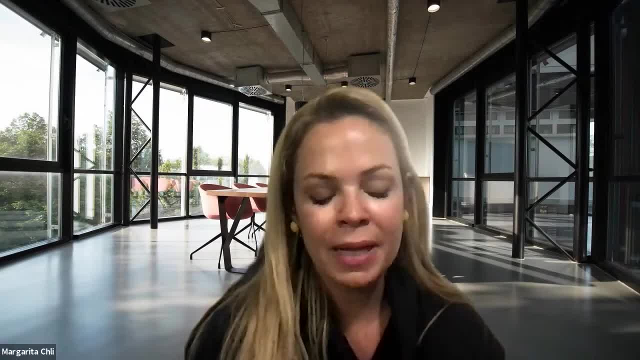 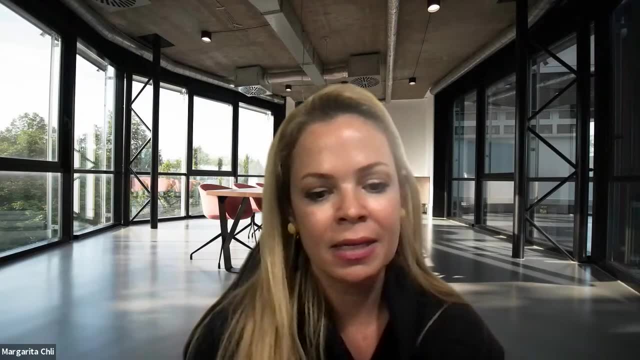 will be helpful for our um, for our path planning, but um, it's not the final answer. i think there's. so we work with different representations and um, everyone has his pros and cons. i think it's good to keep experimenting and, uh, again, it's not something i can give a definite. 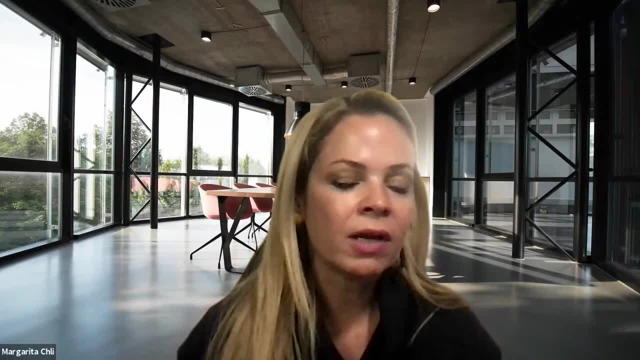 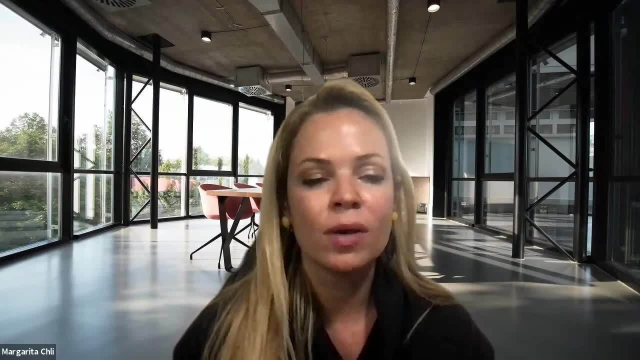 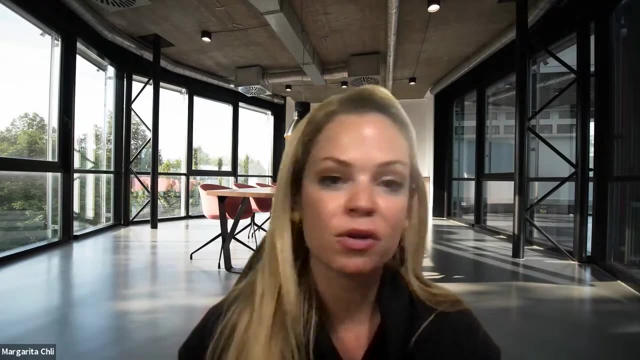 answer for, and i think it's um a very interesting question and and i think also, at the same time, it's cool that we're asking this, because it means that we are at that stage where we are optimizing to that extent um our algorithms, path planning and reconstruction, right um to really ask what. 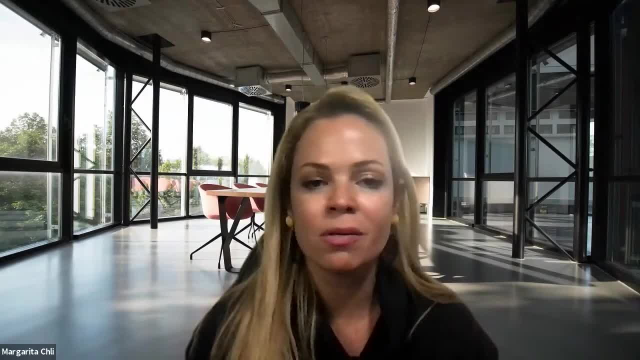 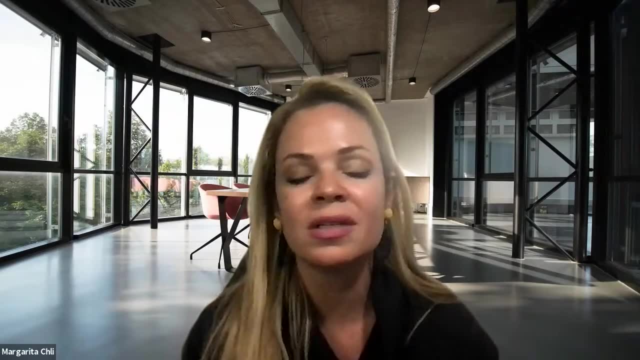 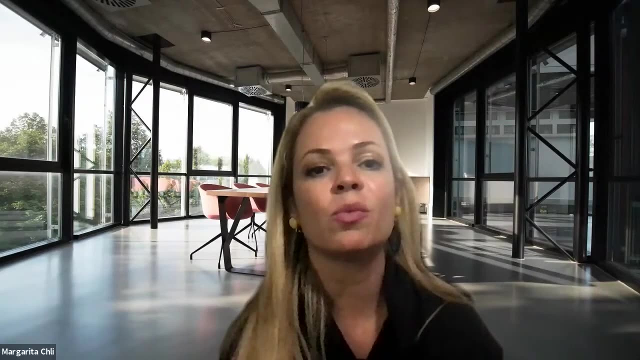 makes good scene representations, um, and that we started all the way from point clouds. right then, what makes a good 3d scene reconstruction? and now, what makes good scene representations in order to avoid obstacles or even um to manipulate objects? and that's even more important, and so i think um your decision. 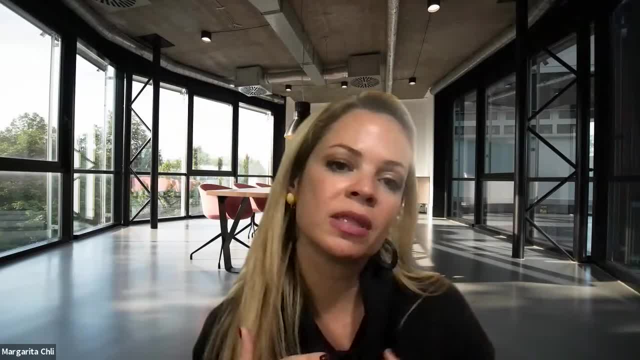 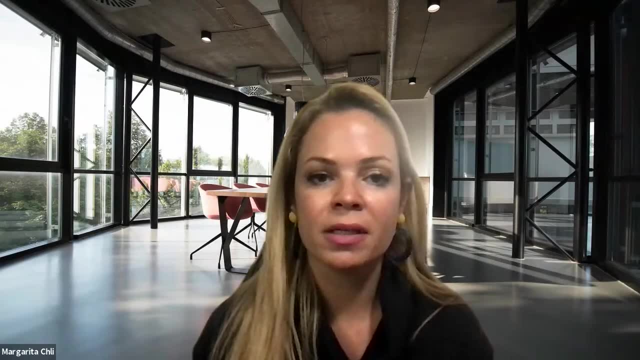 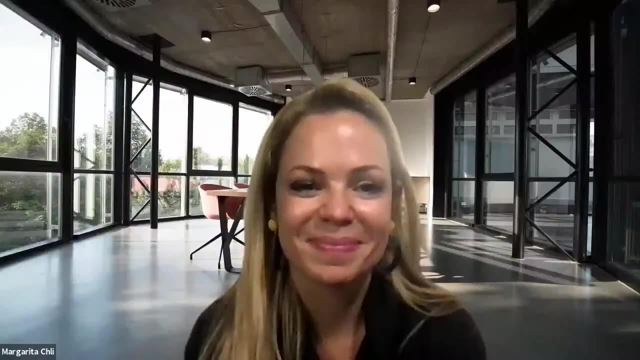 making in that sense goes hand in hand with the application that one has um in mind, and that means basically the accuracy, um and the time requirement. yeah, that makes a lot of sense and definitely an open-ended question. uh, that's probably pretty task dependent. what resolution or free space do you want to work? exactly, exactly, cool, uh, awesome. 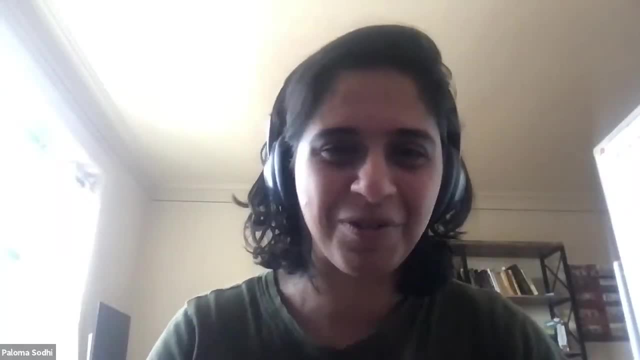 and we're a little bit over time, but i do. there are a couple of questions i'll just uh summarize them and ask you, and that's on the last part of your work on multi-agent collaboration. uh, so i guess, like this work that you showed was um the central server, that the maps were being computed. 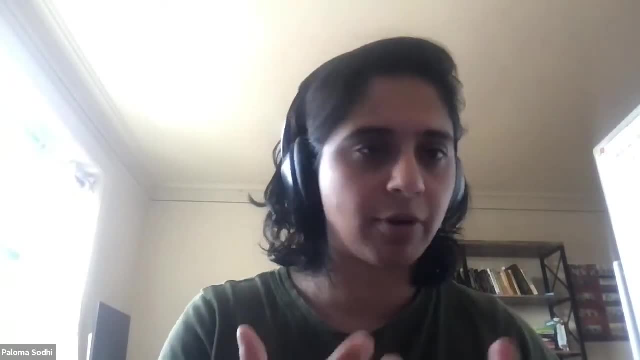 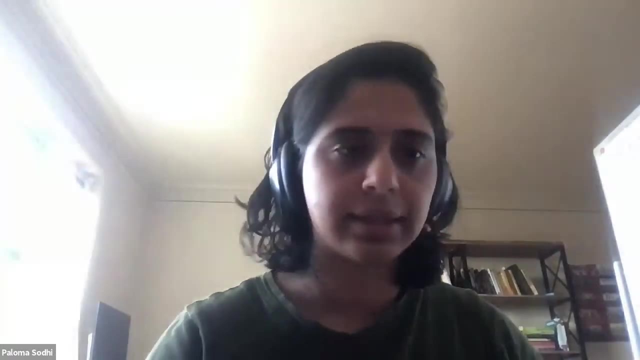 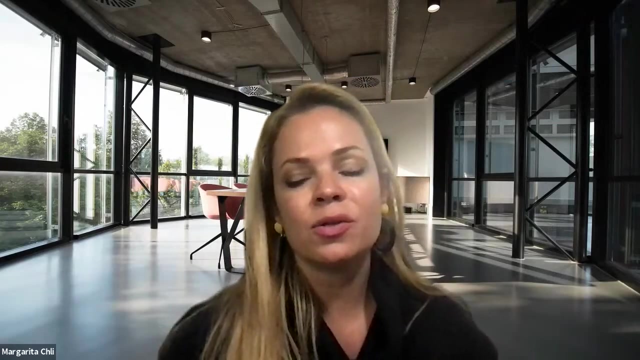 to um. so what do you see are the challenges and what are the challenges that you're trying to move from a central server to a peer-to-peer fashion style um map sharing. what are the bottlenecks in that? so the area where we are focused in- and i think it's quite interesting- is: how do you make? 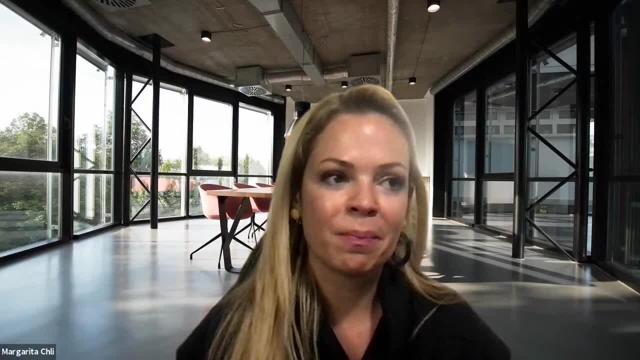 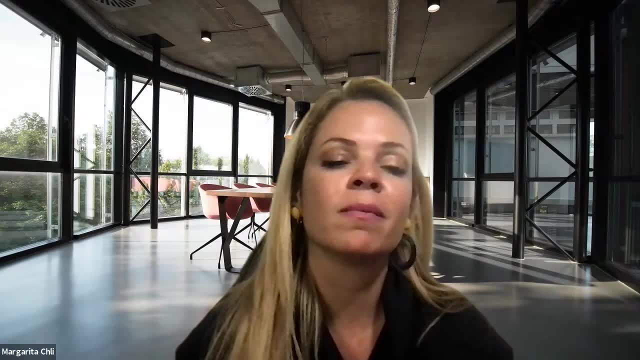 sure that you remain consistent and within your estimates, because with a peer-to-peer communication, with a peer-to-peer- um sorry, this- distributed fashion, you don't instantly have access to the map, so you don't have to be able to do that. so i think that's a really good point, um. 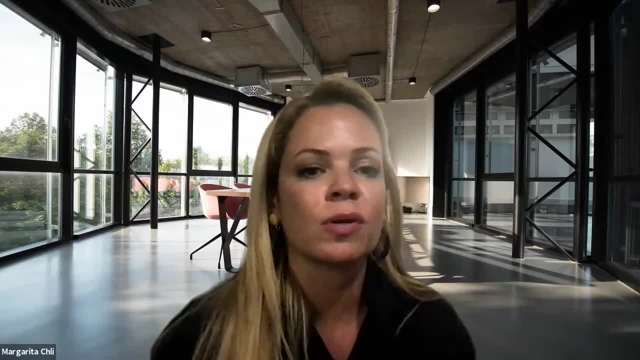 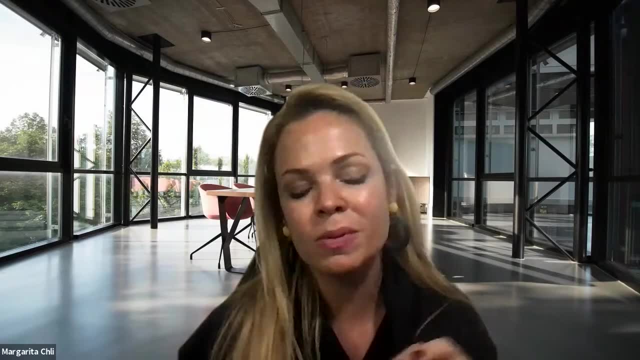 whole map. so this is the beauty of the centralized approach, right? so you can say: i want to see where my drones are right now and what the map looks like, and you have it at an instant, whereas in the distributed formation then you have all the information, but not in a centralized location. so 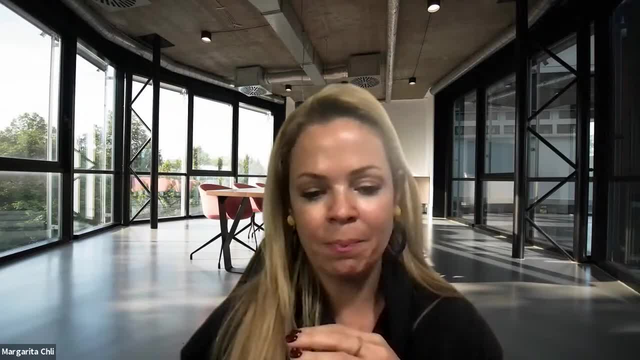 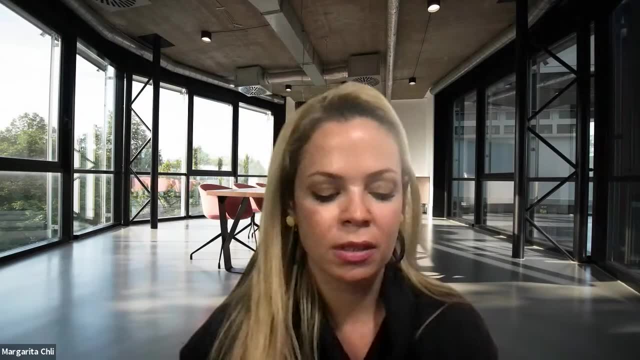 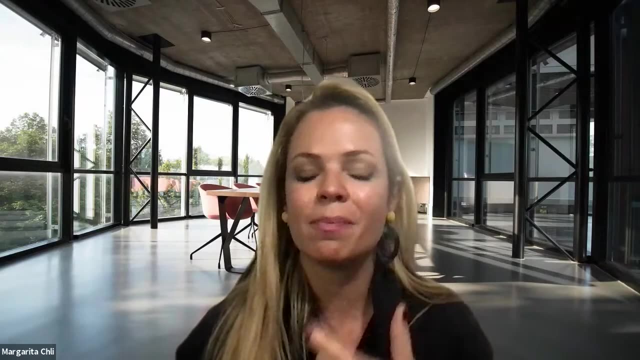 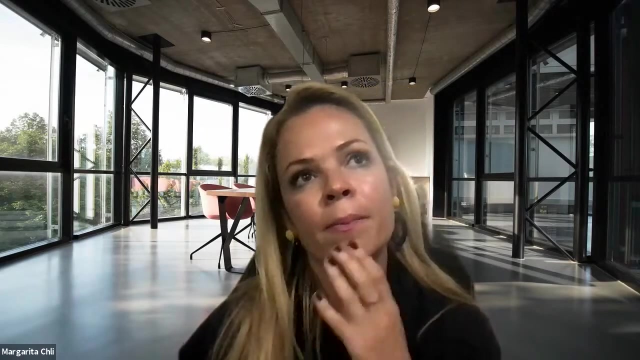 you have to unfold it and, um, there we are studying existing um, uh, existing optimization um strategies, right with message passing, and to see how you experience overlap between different agents. make sure that you understand what is a good neighbor to talk to. so this is on the, on the 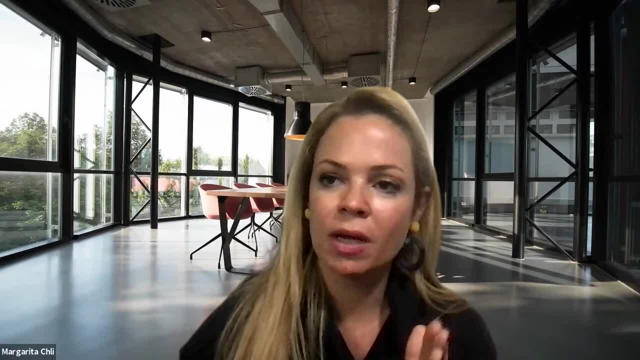 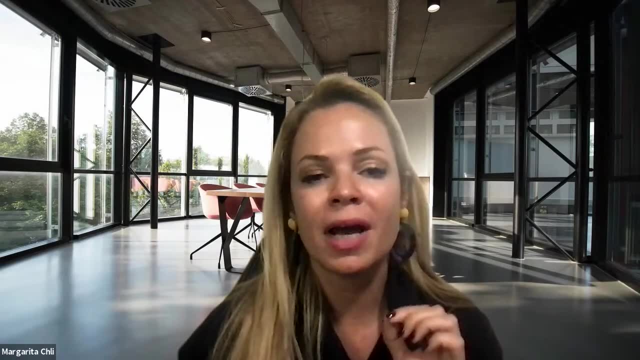 conceptual side of things. now, on the practical side of things, we have some obstacles that i haven't found a good way to overcome yet, and this is really on the communication. really, how do you transmit information from one drone to the other effectively, right? so so far, we are simulating this. 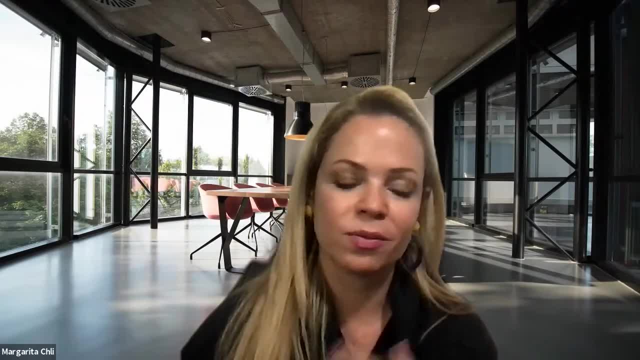 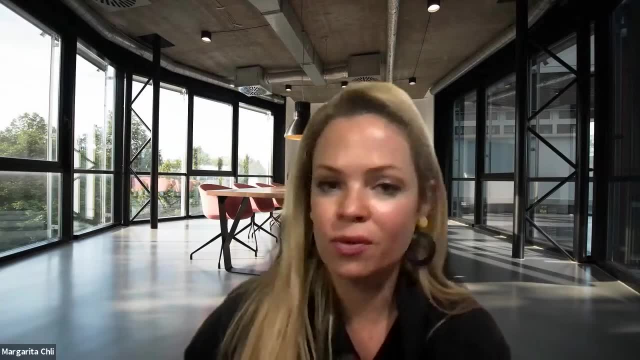 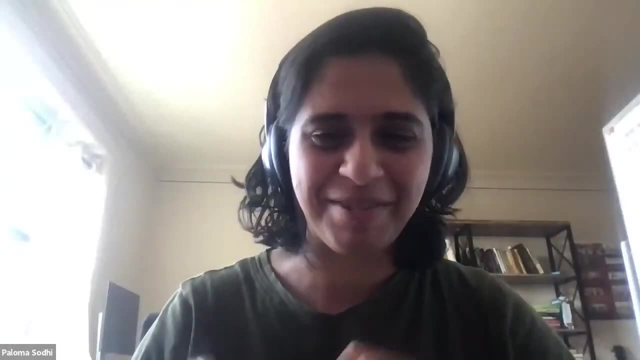 communication by um, a wi-fi network which is not distributed but it's very much centralized, uh. so i think there's also there there's a way to go for the hardware and way to go for the software side as well. definitely, and this is like great, first uh thing to uh yeah, have a baseline on uh. 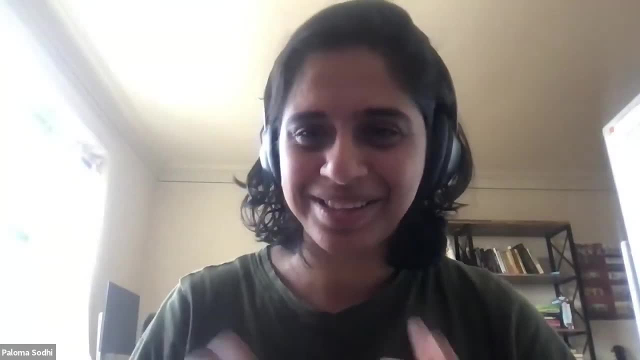 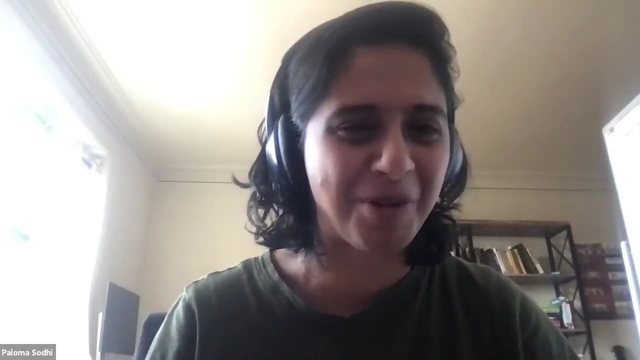 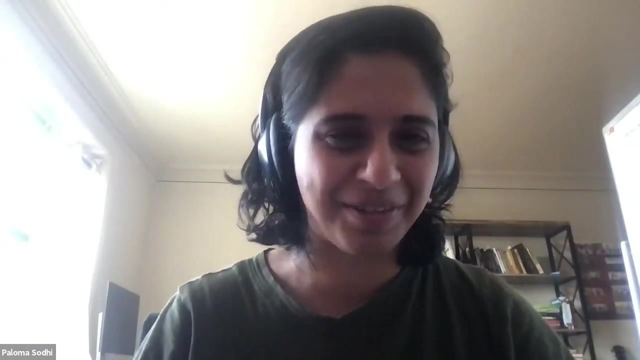 to compare. okay, awesome, uh, i think. uh, that's all the questions and, um, thank you so much for coming out here. i think your talk really highlighted some very important problems in slam that, uh, we should be thinking about and, uh, thank you so much for your time and it was a pleasure having you here. 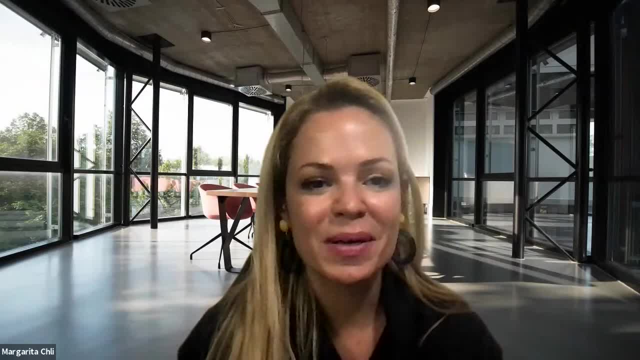 thank you for the invitation. it was a pleasure to give the talk and to have all these questions, so have a good afternoon, everyone. see you.